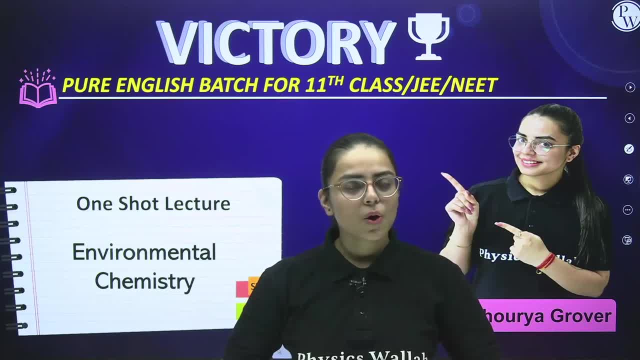 are going to deal it in a quite different manner. We are going to deal it in a quite different manner. We are going to take our NCRTs with us. Okay, I want you all to take out your NCRTs. keep it in a. 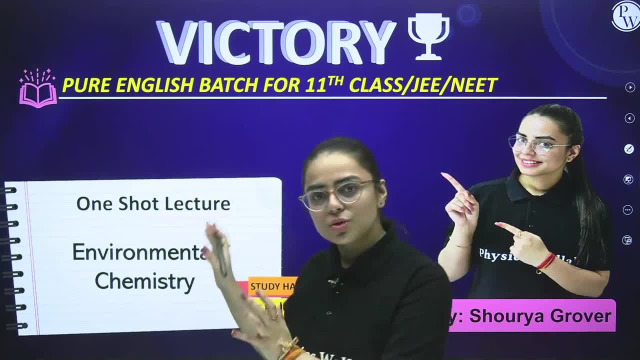 side and, you know, keep marking the points which I am going to tell you, And if there is any another different point, you can also add in your NCRTs. So this will be a best way to deal with this chapter, right? So, first of all, students, what do you mean by environmental pollution? Now, I think 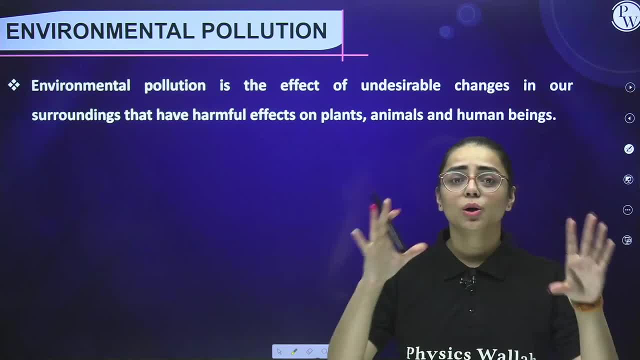 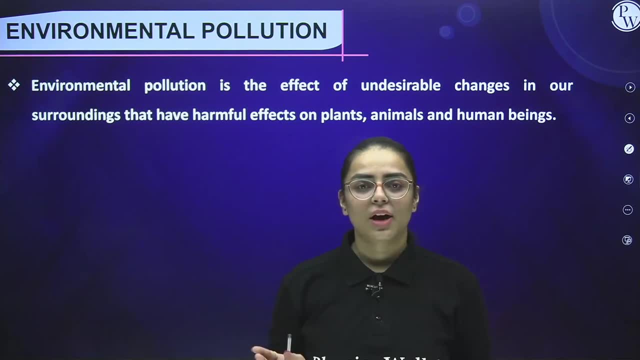 that there is no need to define environmental pollution because you all know very easily what is environmental pollution: Any you know undesirable change that is occurring in our environment that basically causes a harmful effect on plants, animals and we all human beings. So that undesirable, you know, changes that are 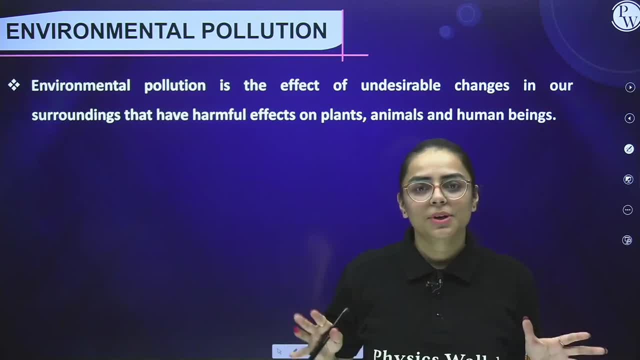 occurring, you know, due to which something is happening in our environment. that is basically environmental pollution, right? So if I am going to define it is: it is the effect of undesirable changes in our surroundings that have harmful effects on plants, animals and human beings. This is environmental pollution. Now, students, we need to know about pollutants. 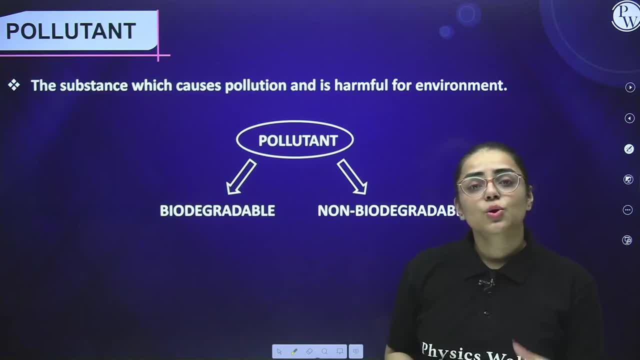 Now, what do you mean by pollutants? These are those substances which causes pollution, which are responsible for causing pollution, So these are referred to as pollutants. okay, And this is harmful for environment? Why? it is harmful for environment? Because it is causing pollution right Now, students. 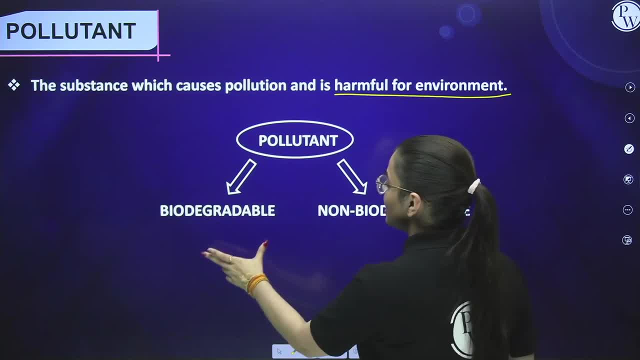 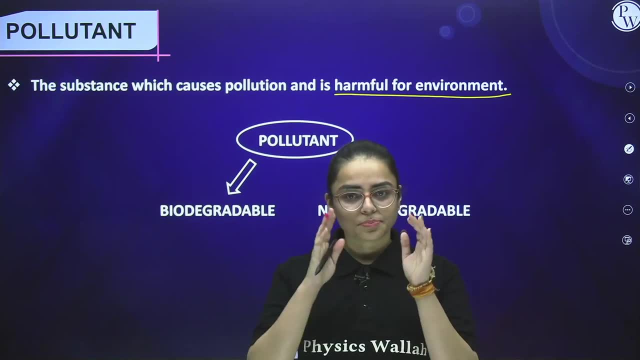 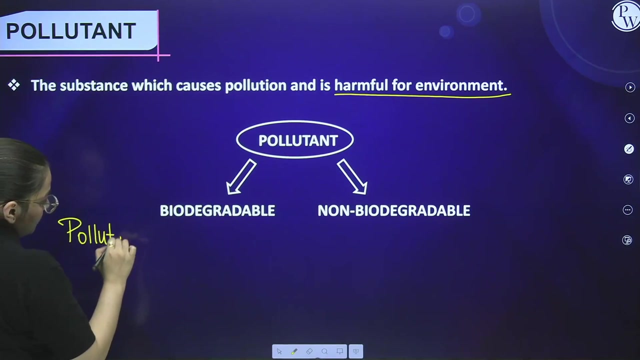 it is further categorized into two types: One is biodegradable and another one is non biodegradable. What are non biodegradable substances? You know the pollutants are, you know, natural, organic substances which can be decomposed by biological processes. They are biodegradable Pollutants. 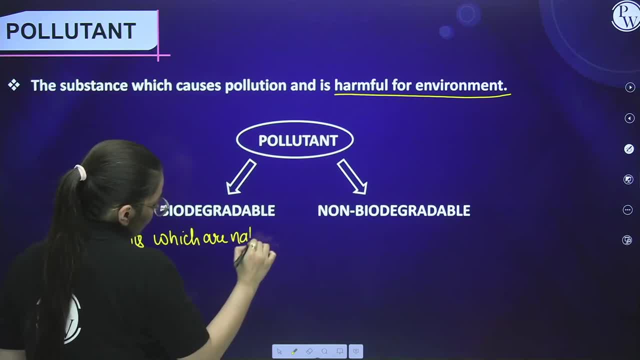 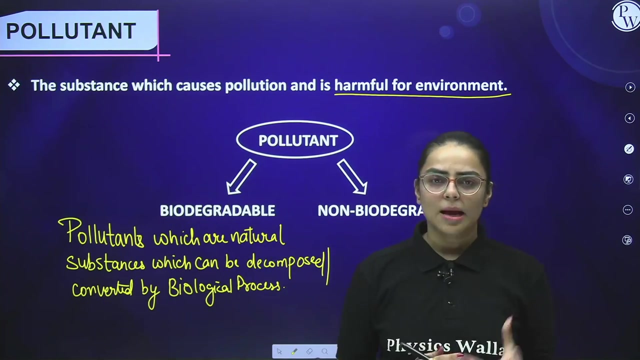 which are natural substances Which can be decomposed or either converted, you can say, by biological process, By biological process is known as biodegradable substances or biodegradable pollutants. Clear students, Now some of the examples for biodegradable, I would say, domestic waste, of course of. 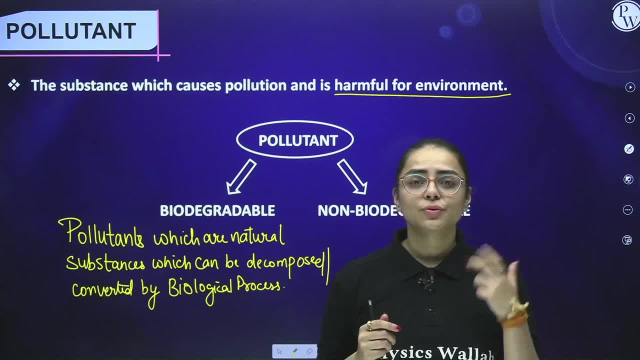 all kinds of waste, But what is biodegradable? What is biodegradable? What is biodegradable? If I would say paper, I would say wood. all of these lie under the category of biodegradable. Other than this, you can take vegetables, stuff, plants, okay, all of these, So we can write over. 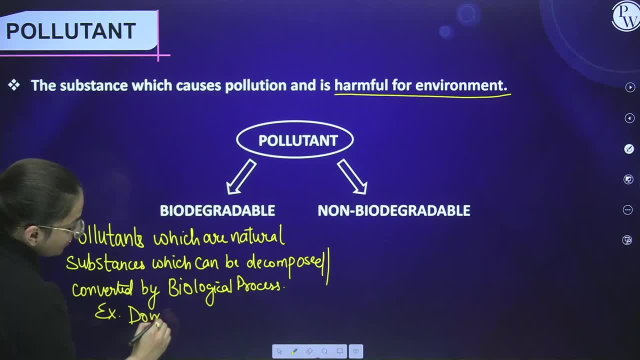 here. if you want to write the example, It can be domestic waste, paper, wood. all of these lie under the category of biodegradable. Now, if I talk about what do you mean by non biodegradable? Basically, these are biodegradable substances. They are biodegradable substances. They are biodegradable. 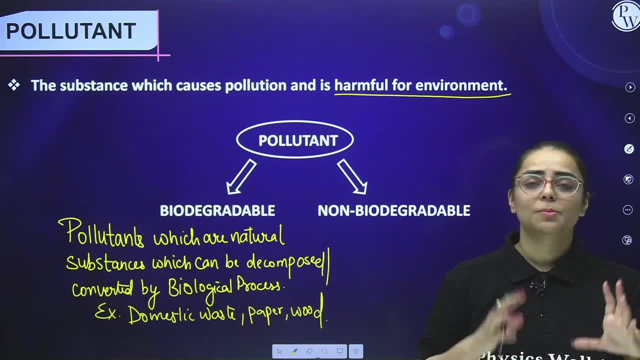 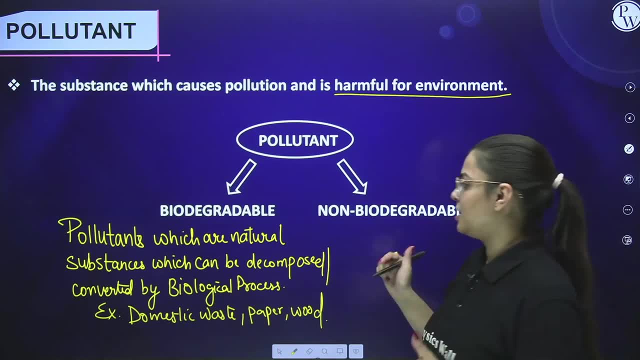 liquid good. they are biodegradable carbon. they are biodegradable fat. They are biodegradable polythene intersections, which are biodegradable. So all these biodegradable substances is non biodegradable substances. If you look at the chocolate, bar, lipstick or jousts, All 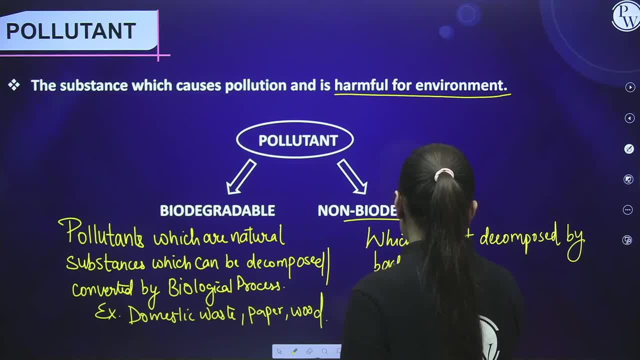 of the factors. welcome tonali thesis of musun with the� wardrobe, which is, of course, a biodegradable substance In the past, while and today it is due to freshman materials'. other than this, we can say more example of pesticides: okay, we can take DDT also in this. 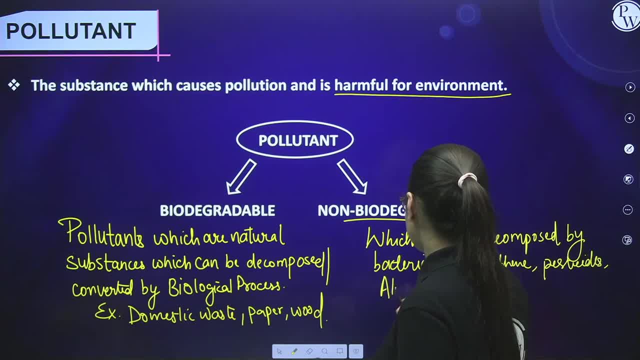 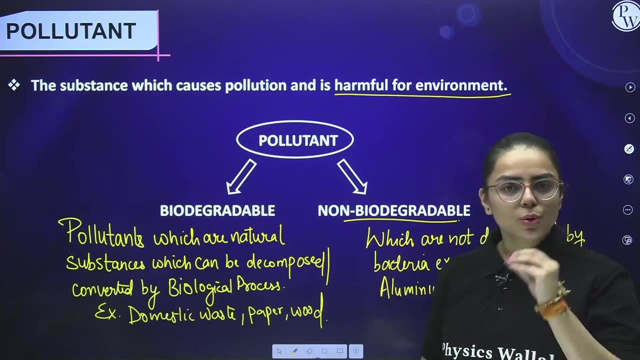 we can take aluminium, you know, can also in this. Now these all are referred to as biodegradable or non-biodegradable substances, and these are referred to as the biodegradable one. Now you know what do you mean by pollutants, The one which causes pollution, right? 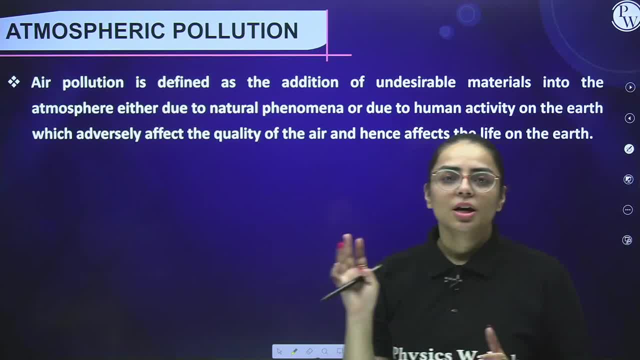 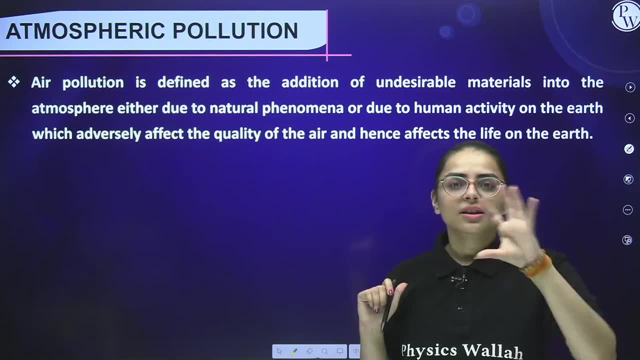 Now let us see our next segment, that is, atmospheric pollution. Now comes a very important topic. atmospheric pollution is basically air pollution. Air pollution is the one there. we can say that basically it is the addition of undesirable materials into the atmosphere, into the air, which leads to you know the harmful effects. 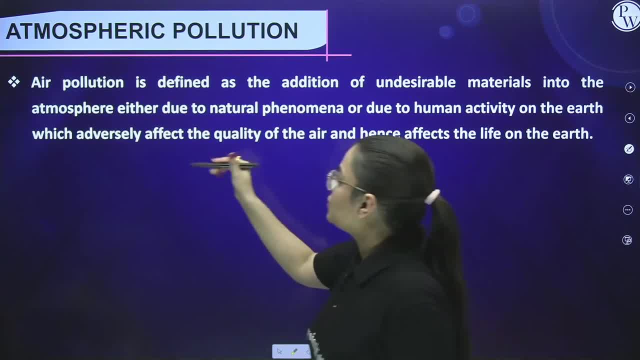 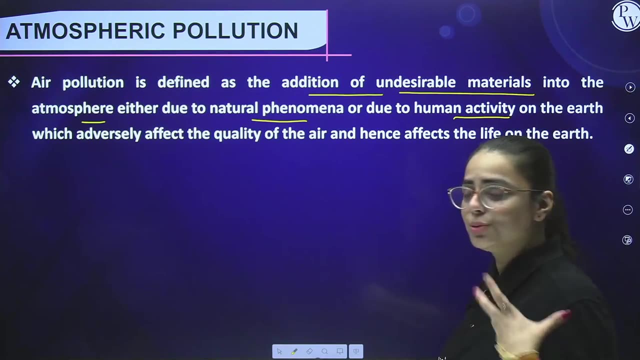 on plants, animals, human beings right. So if I would say air pollution is defined as the addition of undesirable materials into the atmosphere or into the air, either due to natural phenomena which is occurring naturally right, or due to human activity that we all do, you know, human activity. 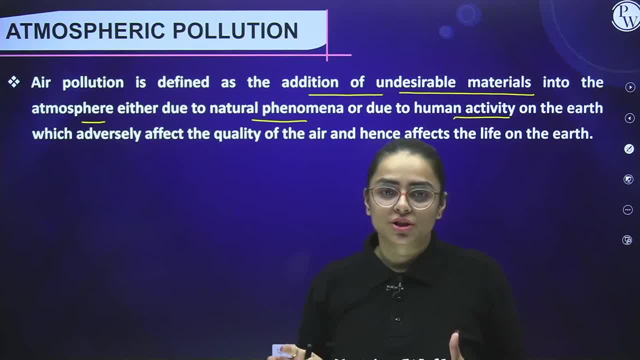 We humans are also responsible for causing a lot of pollution. yes, why not? So, students, over here, they are saying the one which is automatically caused, that which means that is natural process, and the another one that is causing the. you know the humans. we humans are causing some of the pollution through the vehicles. I would say. 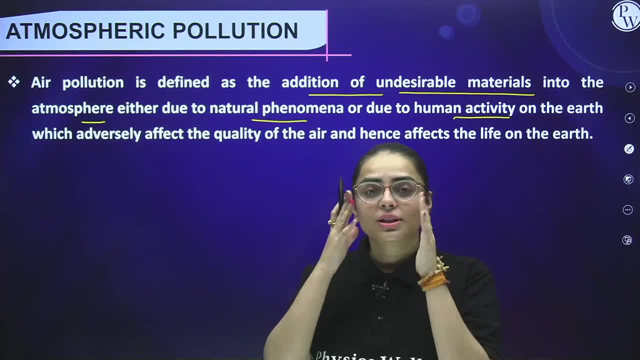 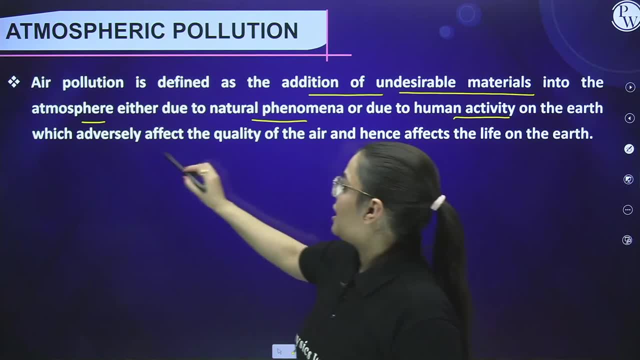 So we humans are responsible for causing some of the pollution through the vehicles. I would say, Or you can. you can say the vehicles, right. So the pollution that is caused from them is air pollution, right, So we can say which adversely affected the quality of the air and hence the affect the 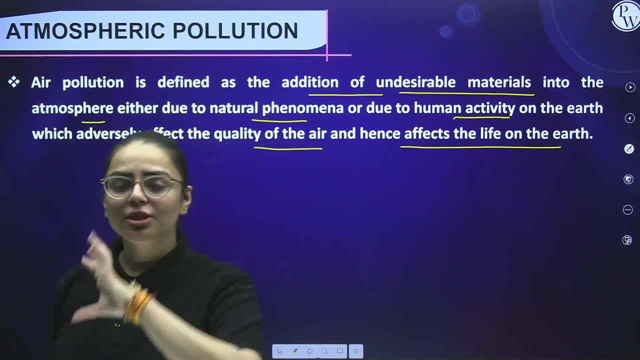 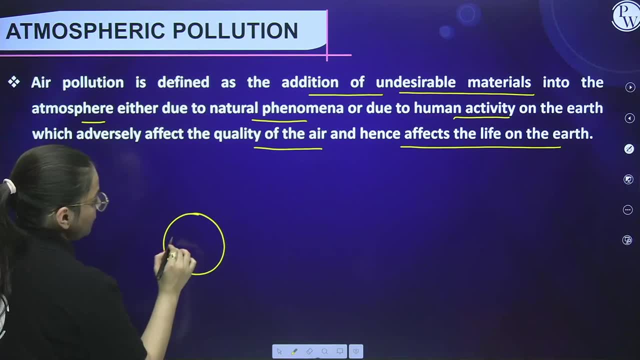 life on the earth, right, right, students, Now let us talk about you know earth. If I talk about earth and its surroundings, I would say: if, for example, this is earth, right, If this is the earth at 10 kilometer from earth sea level. 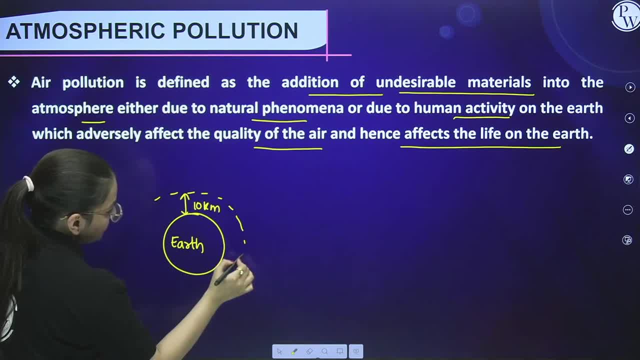 At 10 kilometer from earth sea level troposphere is found. which layer is seen, Troposphere layer And from troposphere? you know, at 40 kilometers From troposphere, at 40 kilometers Or at 10 kilometers from earth? 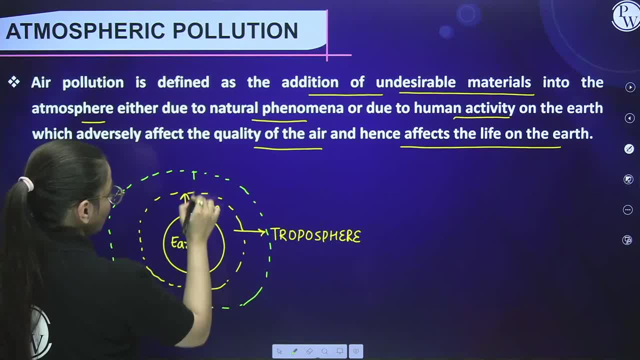 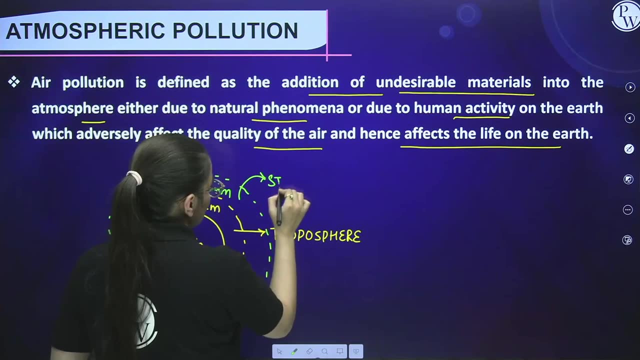 Okay, So I would say from the sea level at 50 kilometers. If I am talking about the sea level, it is 50 kilometers. If I am talking about only from the troposphere, it is 40 kilometers. right Now, this layer, the second layer, is stratosphere. 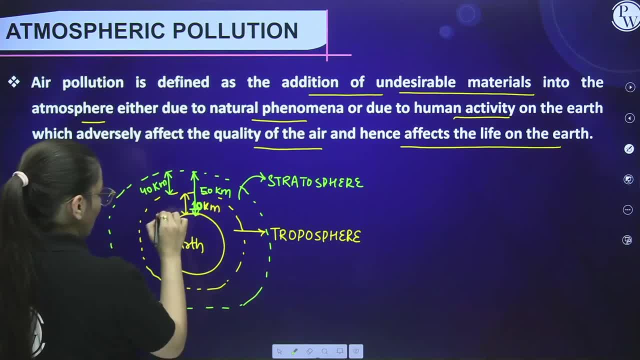 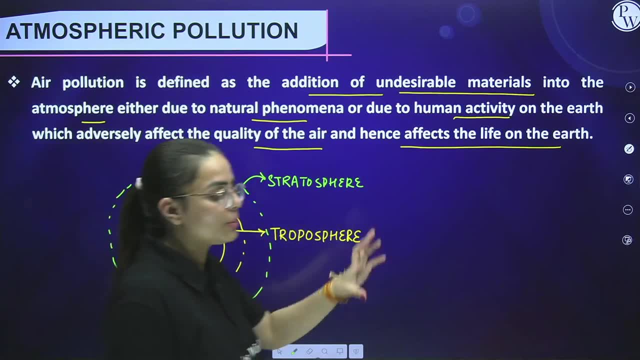 Now, here I am writing this again. it is 10 kilometers. I am writing over here. Do not get confused. This is 10 kilometers, This is 40 kilometers, It combines to 50 kilometers. Now, if I am talking about troposphere, it is at the 10 kilometers from the earth sea. 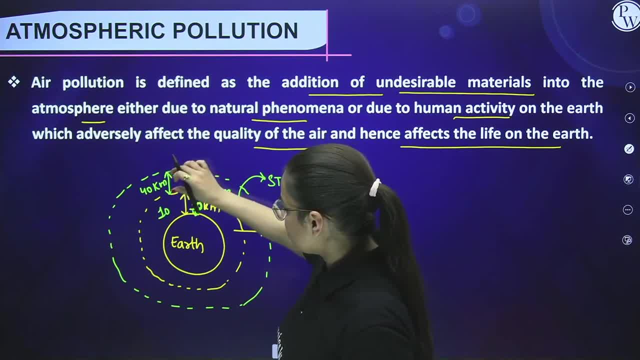 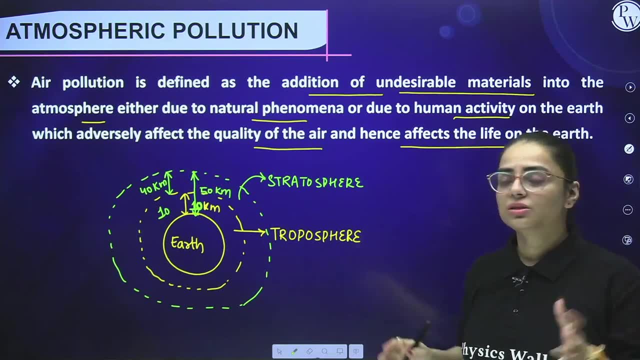 level and basically stratosphere lies at the 40 kilometers from the troposphere or 50 kilometers from the sea level. Is it clear? Now? these are very important because we are going to learn what is the tropospheric pollution and what is the stratospheric pollution, because we are talking about atmospheric pollution. 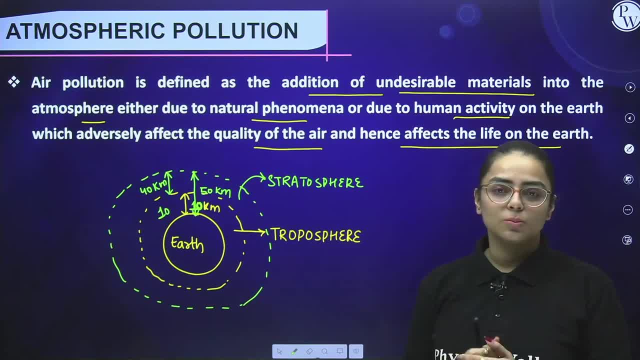 So we are going to talk about all about atmosphere that is occurring in our atmosphere. Now, if I talk about what are the things that land on the earth, What are the things that lie in the troposphere, or what are the things that lie in the stratosphere, 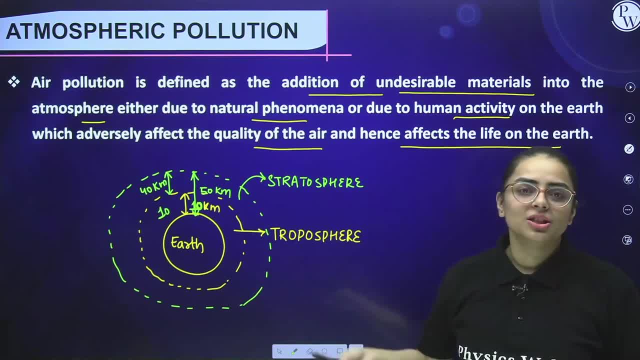 First of all comes troposphere. You know all the climatic changes we talk about, the weather changes we talk about, You know all of these basically lies under troposphere. You know, over here I would say it is the climate change or I would say it is the weather change. 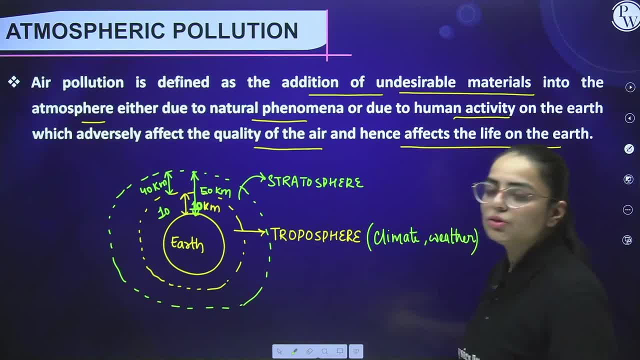 Everything that you know, we look over, we look over in the troposphere, We study in the troposphere, right, And if I am talking about the stratosphere, here O3 is present. That means ozone is present over here. Here ozone is present which protects from the harmful radiations of the sun, which protects 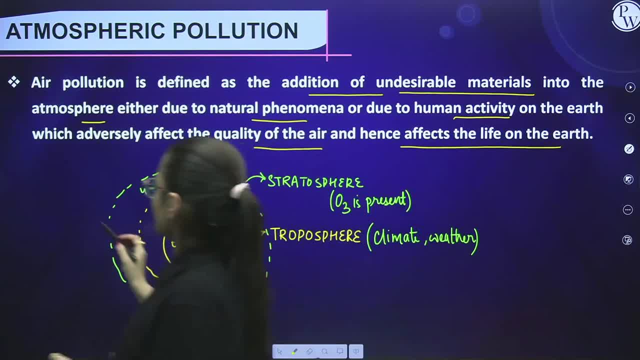 our earth from the harmful radiations. For example, students, here is the sun, here is the sun, here is the sun. So harmful radiations are caused by the sun. Now, basically what happens? Our stratosphere contains ozone, which protects our earth from harmful radiations. 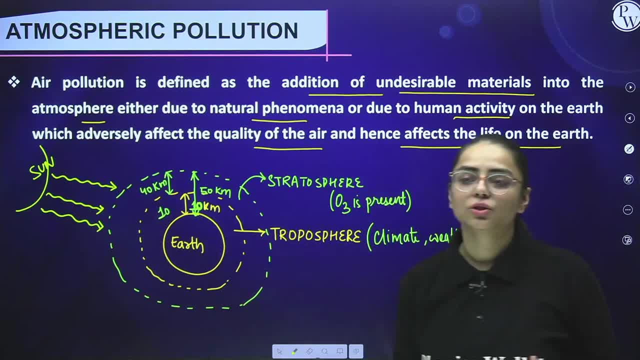 So here is the sun. Our earth contains ozone which protects our earth from this harmful rays of the sun. right, This protects from the harmful radiations of the sun, harmful radiations coming from sun. right, Very sorry. Okay, So these protect from the harmful air, harmful radiation that comes from the sun. 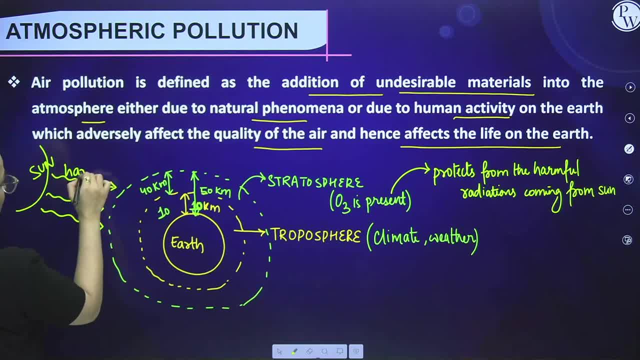 In other words, I can write over here also: these are the harmful radiations. Okay, now, students, this you have got to know about: what is troposphere, What is stratosphere? right Now, if I move forward, if I go forward, I am going to see the pollution, the kinds of 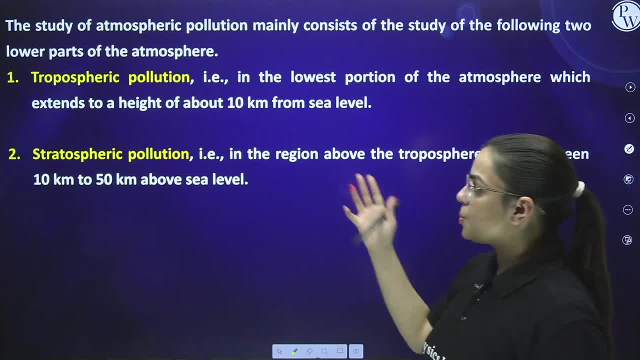 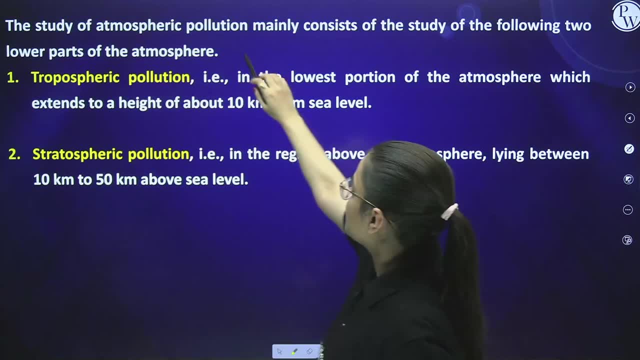 pollution. The very first kind of pollution which I talk about is tropospheric pollution, and the second one is stratospheric pollution. see when I'm talking about tropospheric pollution. the study of atmospheric pollution mainly consists of the study of the two following lower parts of the atmosphere: tropospheric and the stratospheric one. 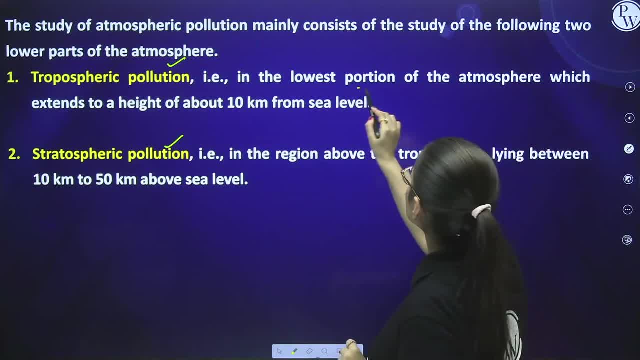 tropospheric pollution is the one that is, the lowest portion of the atmosphere, which extends to a height of about 10 kilometer from the sea level. right, I've already told you, and if I talk about stratospheric pollution, it is the region above the troposphere lying between 10 kilometers to 50 kilometers above the. 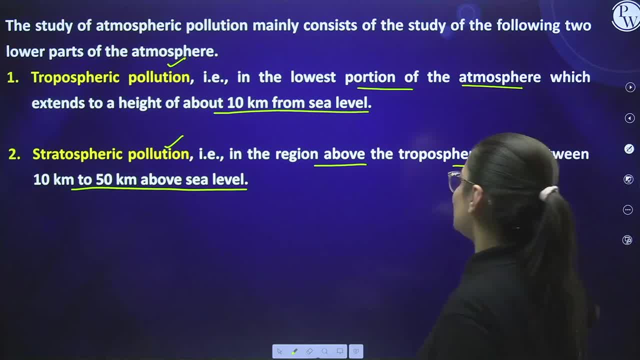 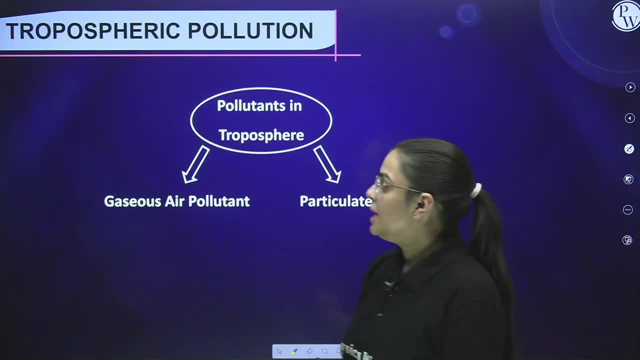 sea level, is it clear? okay, this I have already told you with the help of an example. now come students. our first category, that is tropospheric pollution. see if I talk about tropospheric pollution here. which are the pollutants? now, what are the pollutants? pollutants are the one which causes. 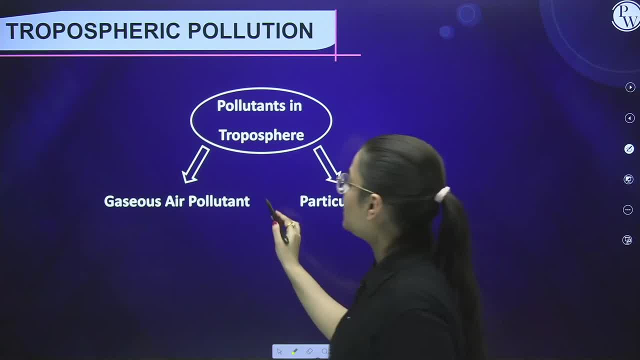 pollution. right, so the pollutants in the troposphere are basically gaseous air pollutants and another one are particulate pollutants. right, students? if I talk about the gaseous pollutants, let us take an example. if I talk about SO2, you know, which is seen from the industrial waste? 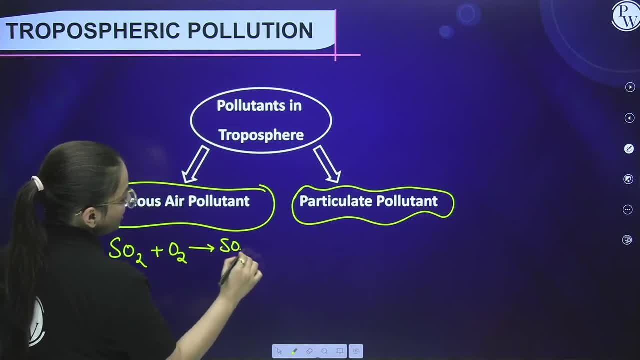 now, when it reacts with O2, it basically forms SO3. this comes from the industrial waste. okay, so when it combines with O2, it forms SO3 and SO3 on for the combination with H2O forms H2SO4, now SO3. on for the 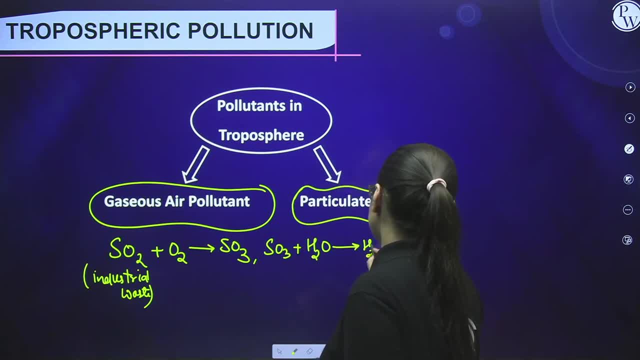 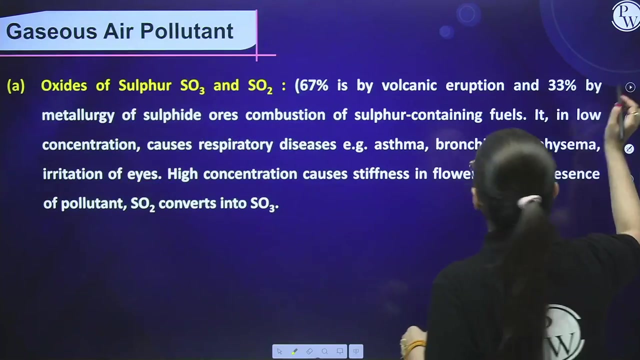 combination with H2O forms H2SO4. now when students H2SO4 is produced. basically it causes a lot of diseases. it causes respiratory problems and mainly it causes a greenhouse effect also. greenhouse effect also and also respiratory problems are seen. greenhouse effect is also seen right now, students moving forward. I will tell you. 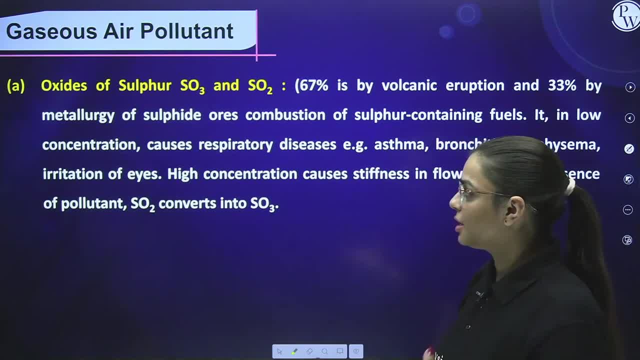 about the gaseous air pollutant. the very first gaseous air pollutant is about oxides of Sulfer, that is, SO3 and SO2.. I just told you the example. when SO2 reacts with O2, it forms so3, SO3 and 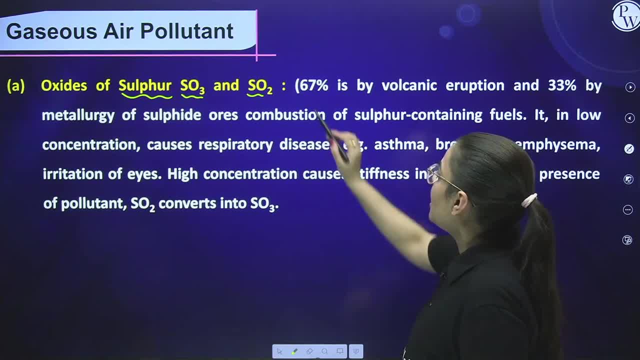 for the reaction is water search with the food which causes respiratory problems. right, who see what they are saying? 67% is by volcanic eruption, маг estructury- and here I just talked about the geological picture that the 하면서e basketball- and volcanic eruption. and 33% by metallurgy of sulphide ores, combustion of sulphur containing. 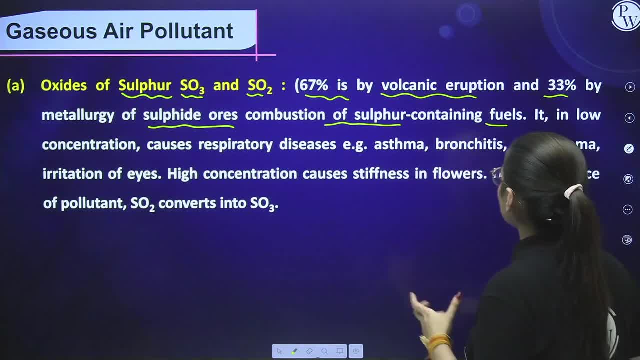 fumes. you know these are for the responsible. right now it, in low concentration, causes respiratory diseases. now, when it is present, in low concentration, respiratory diseases are being caused, which I have already told you. example: asthma is seen, bronchitis disease is also observed. you can say emphysema is seen, irritation in the eyes. you know high concentration causes stiffness. 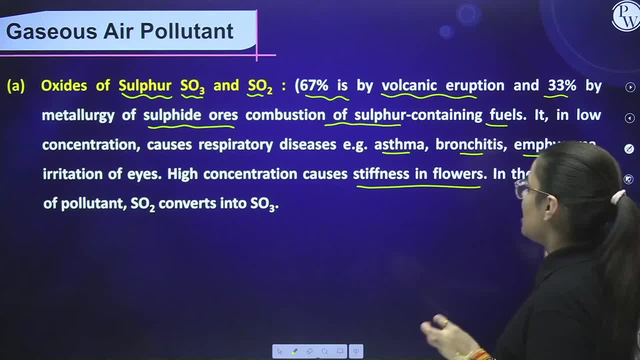 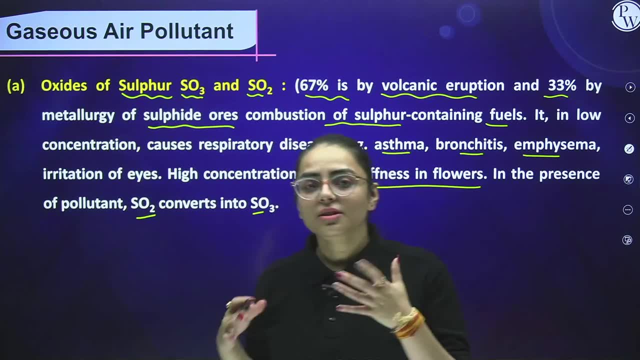 in the flowers, okay, and in the presence of pollutant SO2, converts into SO3, which we have already seen. right. so there are basically, they have told you all the effects that is being caused with the low concentration and with the high concentration. now I would again. 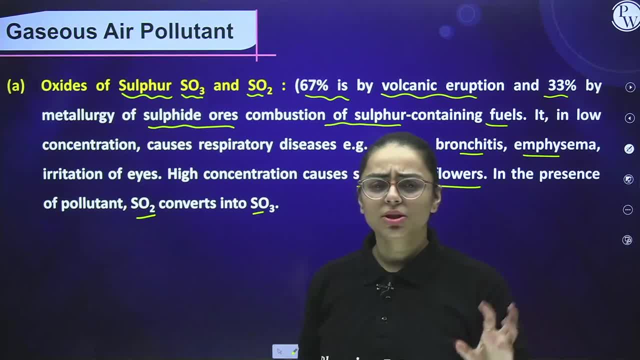 recommend you kindly open up your MCRT, because this is a theoretical kind of you know session. so we are going to you know. we know all the things I know. we are going to know all the things I know you all people know- about pollution. so do not skip. first of all, do not skip because 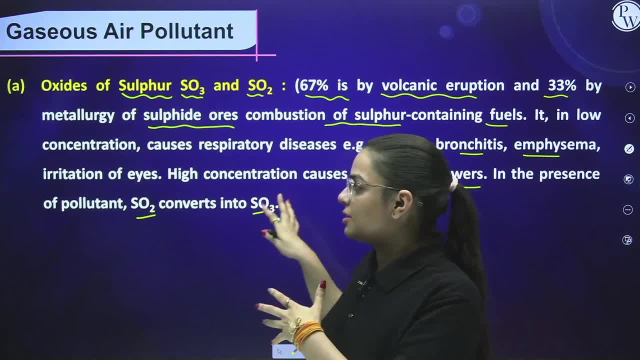 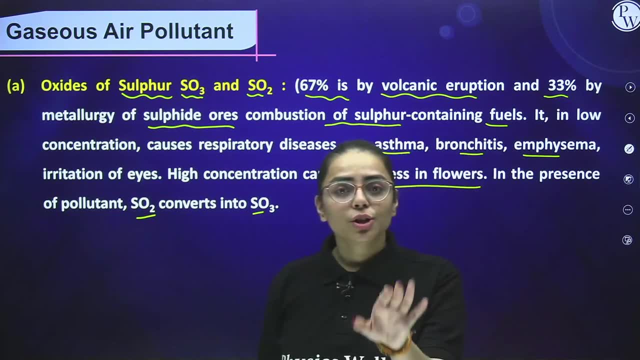 yes, there, if you are looking towards this segment, I want you all to you know if you are getting any question in your examination. I want you all to get the full marks in this chapter right. so what you have to do is you have to cover the NCFT lines one by one. so 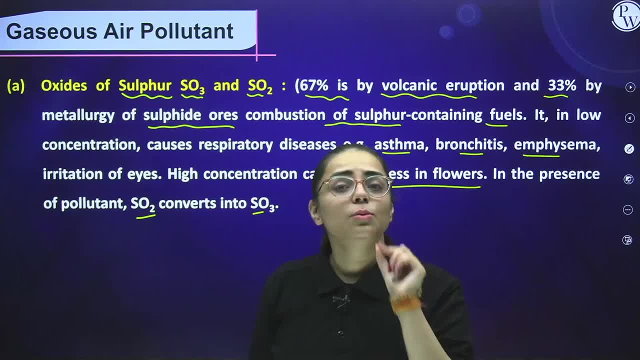 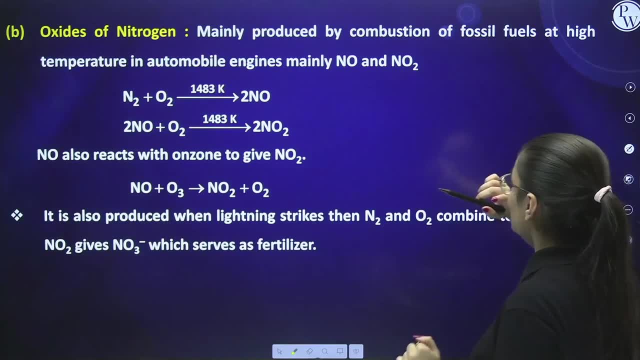 kindly put a highlighter or a pencil and underline the important points at the time. also underline them right now, students, comes the second gaseous case. what you can, if I talk about it is of types of nitrosine. See, if I am talking about nitrogen. in nitrogen, the most of pollutant gas is NO2. this is the. 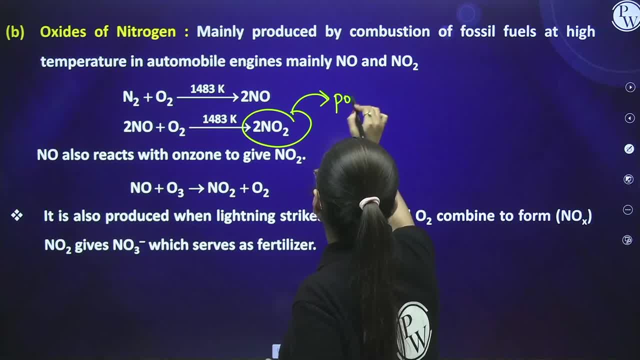 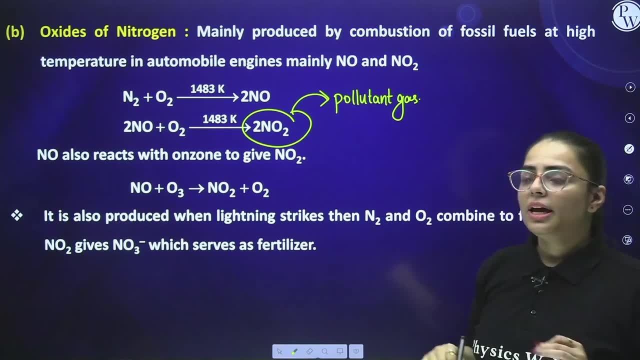 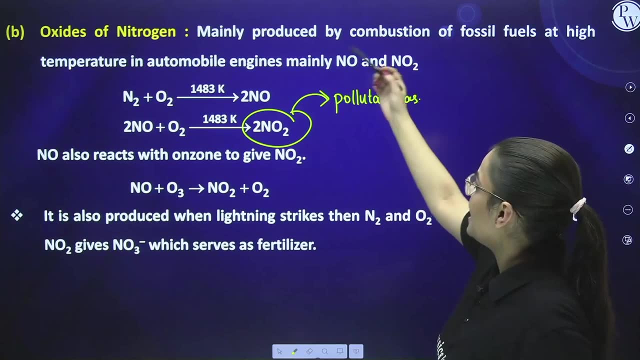 pollutant gas. this is the pollutant gas basically- ok now if I talk over here- mainly produced by combustion of fossil fuels at high temperature in automobile engines, mainly NO and NO2. they talk about this. first of all, what is going to happen see. N2 plus O2 forms the NO and 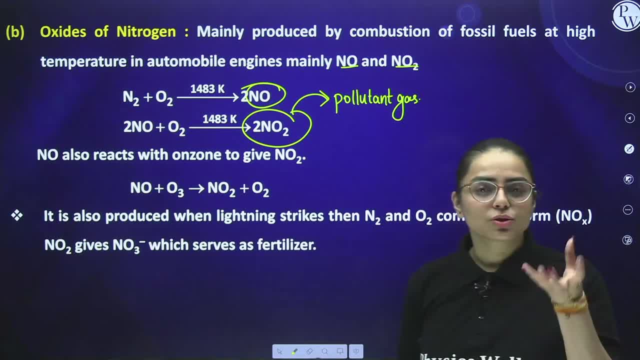 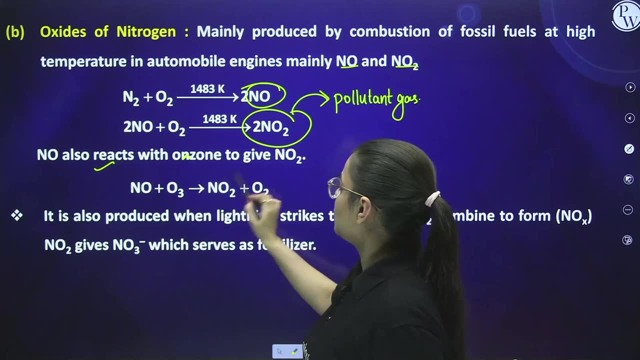 O2 forms. NO, right now NO. and further reaction: with oxygen at a particular temperature which is 1483 kelvin, it produces NO2, which is a pollutant gas. which is a pollutant gas. now what happens over here? see now NO also reacts with, you know, ozone, ozone to give NO2 here. 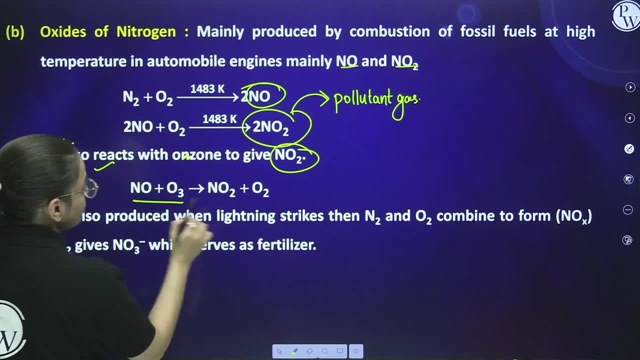 this reaction, students, when NO is reacting with O3 to form NO2. in this reaction, see what is happening: N2 is combining with O2 to form NO, then NO, and further reaction with O2 at a particular temperature forms NO2. but when NO on reaction with O3 instead of O2, it forms. 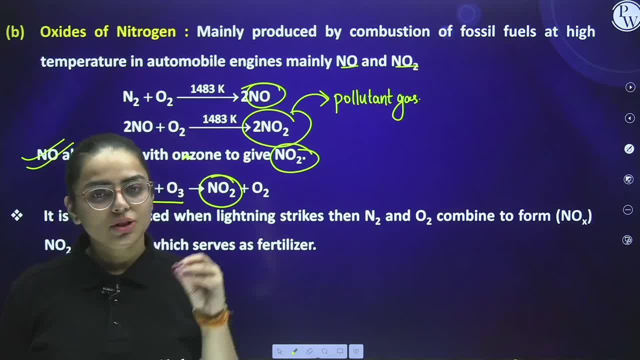 NO2. see, NO2 is produced by both way, either with, you know, with O2 and O3- both way, but with O3, when you are reacting, you know this reaction is quite fast and when it is fast, more amount of NO2 is produced and, as I told you, it is a pollutant gas if NO2 is produced. 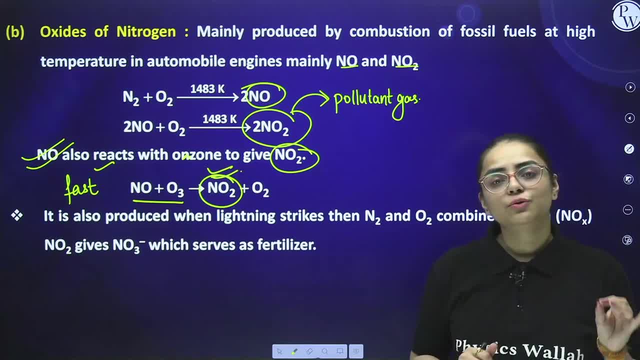 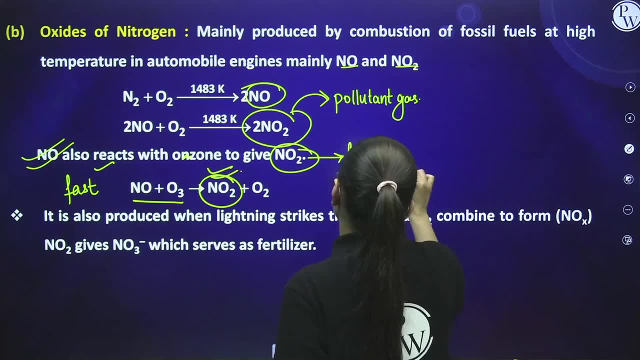 in more amount, then it is very harmful, very, very harmful. so this- this reaction is basically. this reaction is very, very harmful and it occurs very fast. ok, it is also produced when lightning strikes. then N2 and O2 combines to form NO, NO2 and NO3. you know what happens. 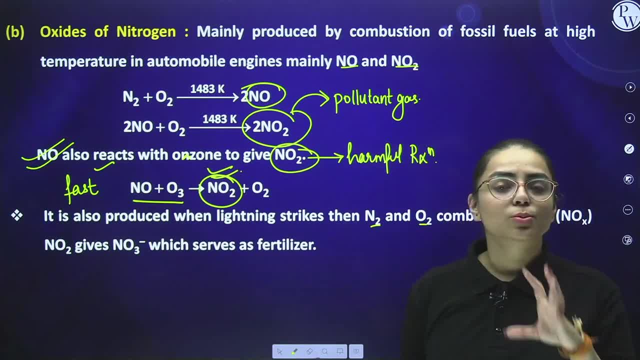 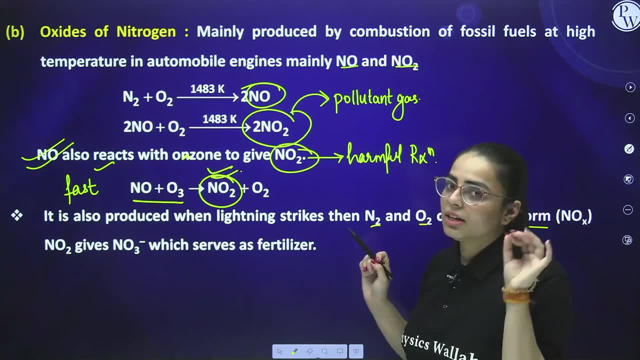 when lightning is there. NO2 is produced because N2 and O2- both they combine with each other, right, students? now what happens? see, this is quite easy concept that you need to remember. very thing in they talk about nitrogen oxide. you should know that NO2 is produced by NO2. 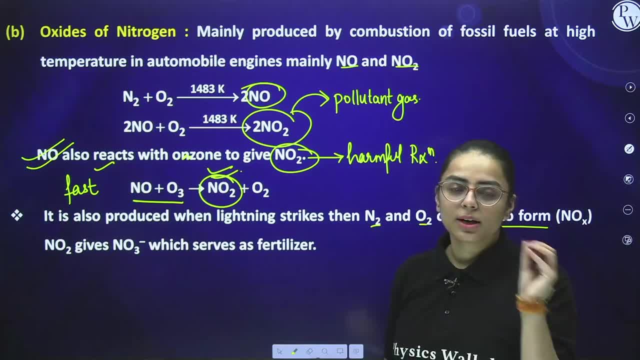 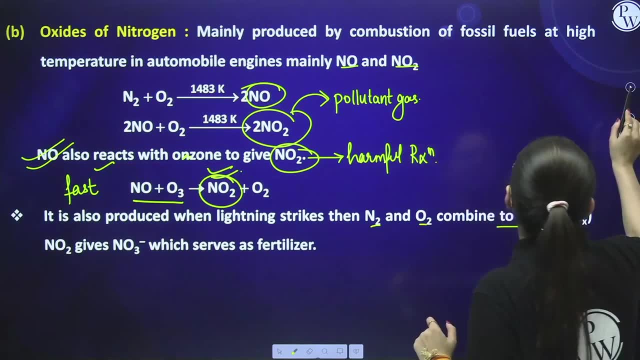 is a pollutant gas. it can be produced by O2, it can be produced by O3. when it is produced by O3, it is harmful because it is fast, right, ok now, students, moving forward towards our effect section. if I talk about effect, we have already done this. effect is basically respiratory. 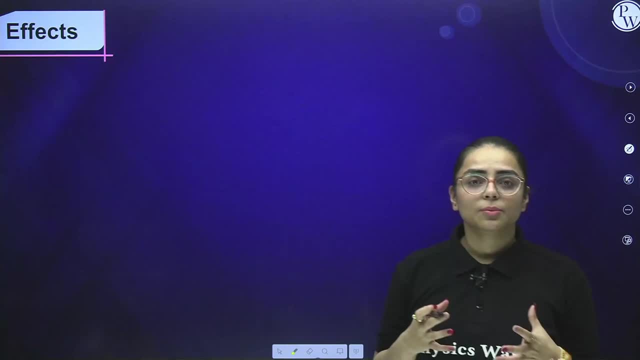 diseases are seen. you know CO2 gases, basically what happens over here. CO2 also act as a gaseous pollutant. if I talk about general CO2- we have seen oxide of sulphur, we have seen oxide of nitrogen now- and what happens here? CO2 acts as a gaseous pollutant. if I talk about general, 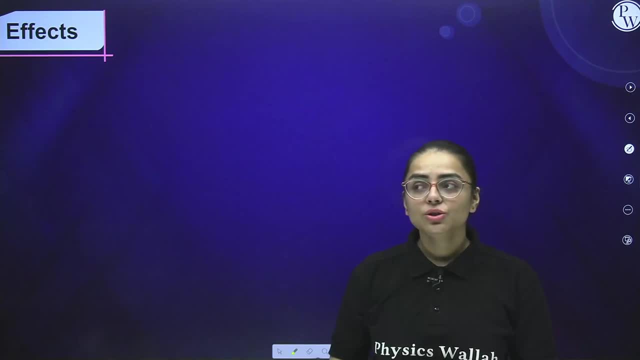 CO2. now another gaseous pollutant, I would say CO2. you know CO2 is necessary for plants also, right, you know this thing now. CO2 is necessary for plants, but the excess amount of CO2 can cause greenhouse effect, right? other than this, what effects can we seen we have? 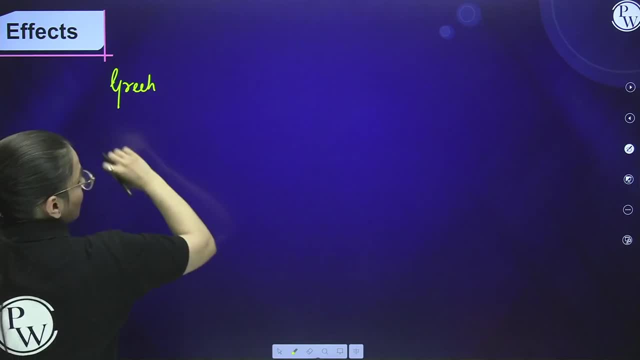 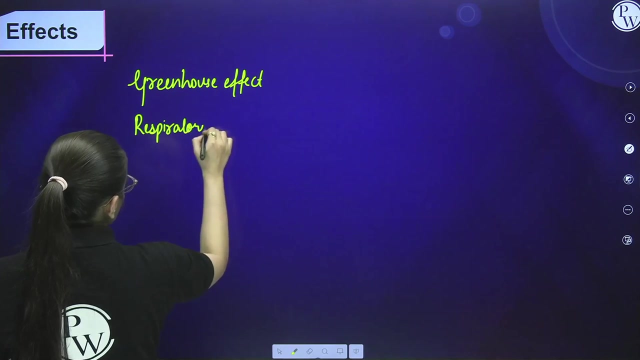 seen greenhouse effect. you can write all the diseases which I mentioned in the previous. you know slide ok, other than this. respiratory problems: you can write all the respiratory problems over here, right, and you can say: you can see the irritation in eyes also, right, students now moving forward. 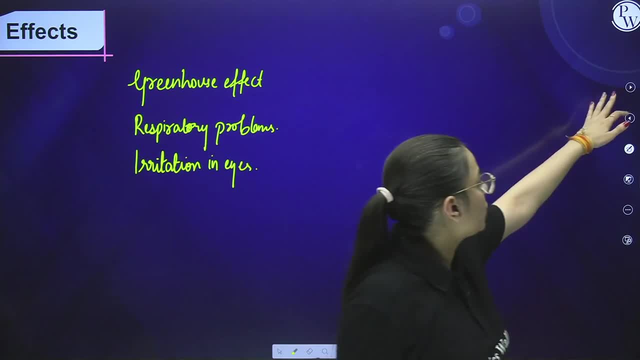 you can write all of these from the LCRT also. it is quite easy, right? students now moving forward. you can write all of these from the LCRT also. it is quite easy, right, students now moving forward. you can write all of these from the LCRT also. it is quite easy, right. 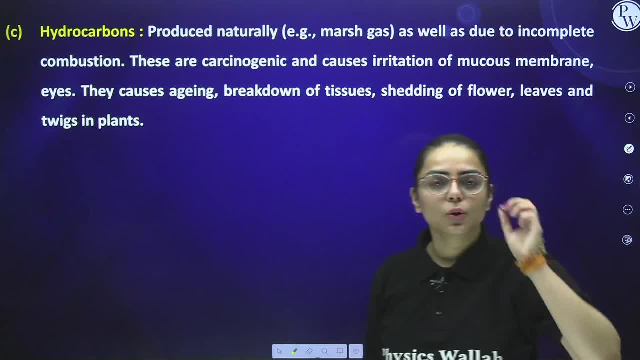 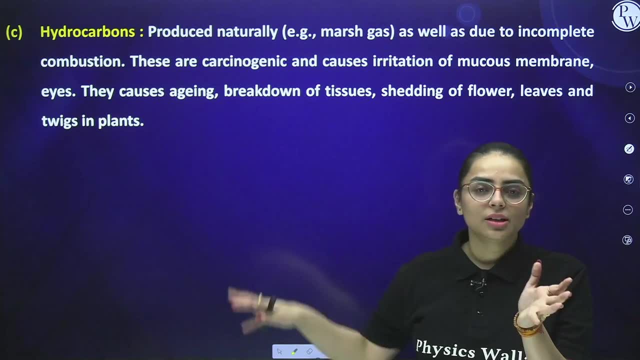 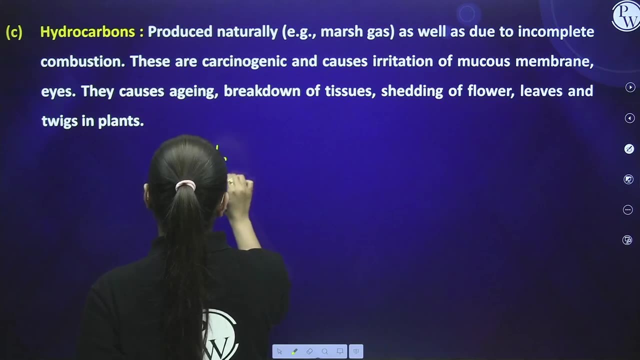 students. now coming to the next pollutant, that is, hydrocarbon. if I talk about hydrocarbon, what happens over here? so, petrol and gasoline in the reaction, in the incomplete combustion, they produced unburnt fuel. what happens, see, when petrol or gasoline taken and incomplete combustion occurs. incomplete combustion occurs so during the reaction of, the reaction of 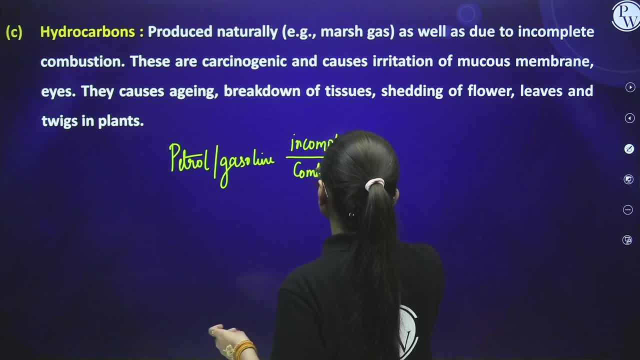 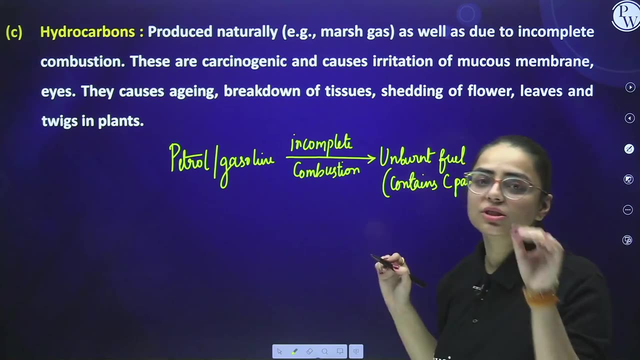 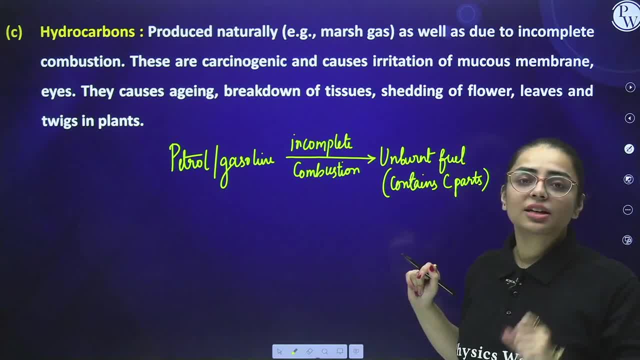 that is produced from this side is carcinogenic in nature. that causes cancer, you know. so this: basically it produces hydrocarbon. that is produced from this side is carcinogenic in nature because only kannst hydrogen is there alone, which is carcinogenic in nature. so this is really very important to you to understand right now. let us read over here: produce naturally. 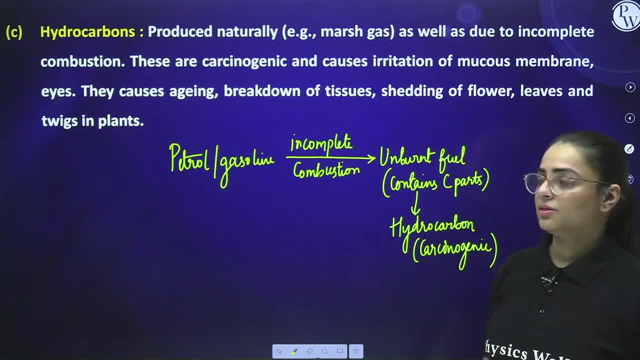 they are produced naturally- example marsh gas- as well as they are produced due to incomplete combustion, which I have already told you. these are carcinogenic and causes irritation of mucus membrane. there is an irritation of the mucus membrane in the eyes right. they causes age in the eyes right, the eyes right. then comes erosion in the eyes and the eyes arterial. 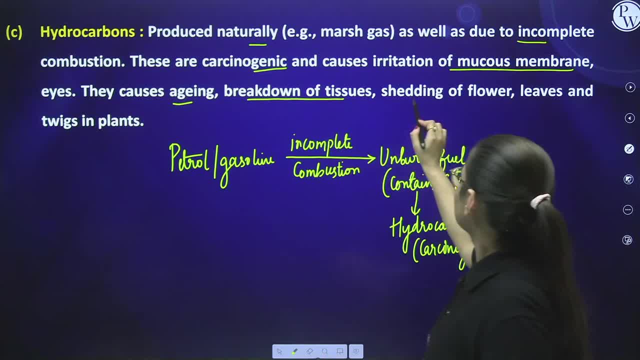 труд behind around you. this result causes irritation of the mucus membrane due to incomplete combustion, breakdown of tissues, shedding of flowers, leaves and twigs in plants, So in the plants also. they cause adverse effects in human beings also and animals also. right. 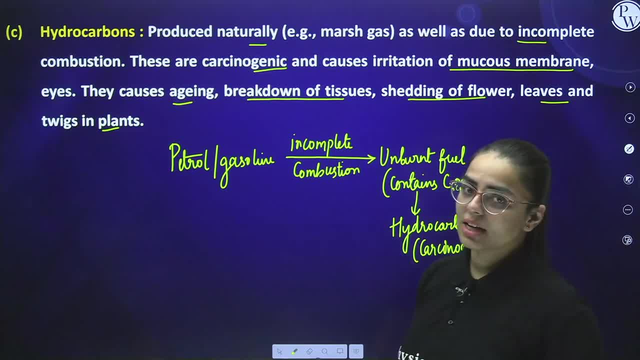 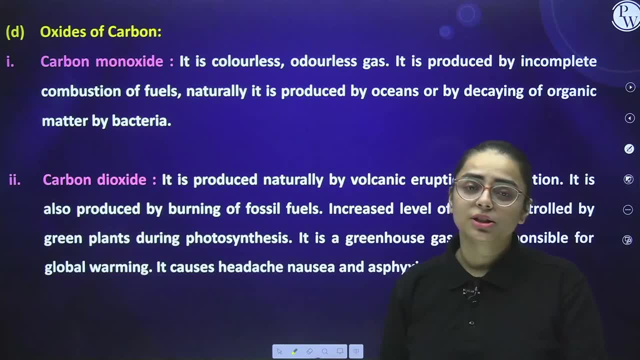 So this is really very important. kindly mention if it is not clear. Now let us see about the oxides of carbon. Now, if I talk about the oxides of carbon, it is quite easy See what happens: Carbon monoxide. you know how is carbon monoxide obtained? 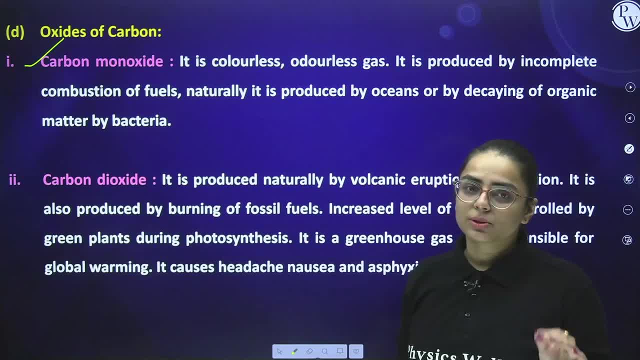 when limited supply of full oxygen reacts with carbon monoxide, is obtained, which is quite harmful. Now what happens? it is colourless, it is odourless gas. It is produced by incomplete combustion of fuels. naturally, It is produced by oceans or by decaying of organic matter by back Right. other than this we have. carbon dioxide, which I have already told you. Carbon dioxide is produced naturally by volcanic eruptions. respiration- okay, respiration process. It is also produced by burning of fossil fuels. By burning of fossil fuels, you can also compare CO2.. Increased level of CO2 is controlled by green plants during photosynthesis, When there is an increase. 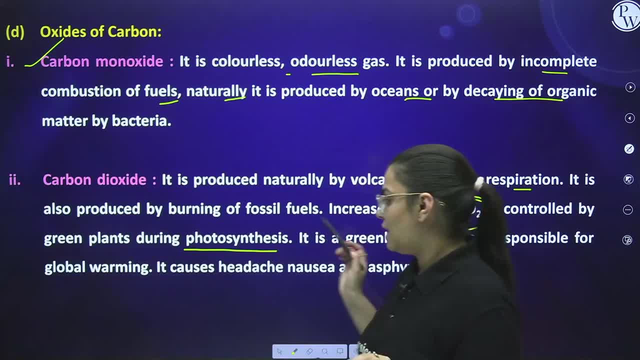 in the level of the CO2, green plants. they will control with the help of photosynthesis. It is a greenhouse gas and responsible for global warming, Responsible for global warming. but yes, it is necessary also. but high amount of this can cause adverse effects, right? 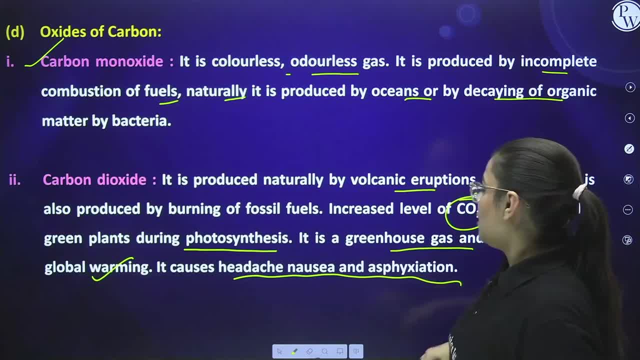 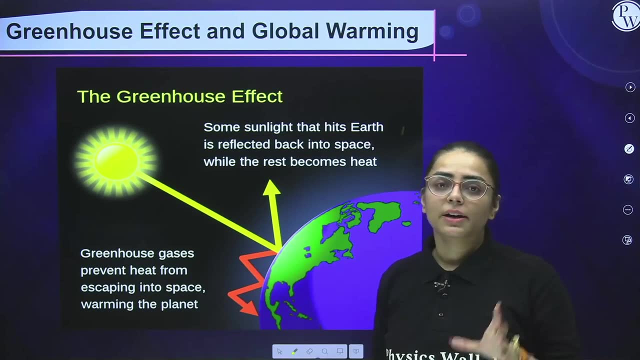 Okay, it causes headache, nausea. you know all of these problems. Respiratory problems are seen, irritation in the eyes, skin issues- These all effects it causes right Now. if I talk about greenhouse effect on global warming- We have seen all the pollutants- right Now comes. what do you mean by greenhouse effect? See what happens over here. Basically, 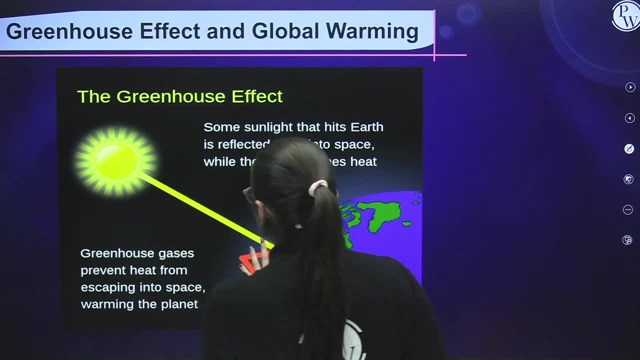 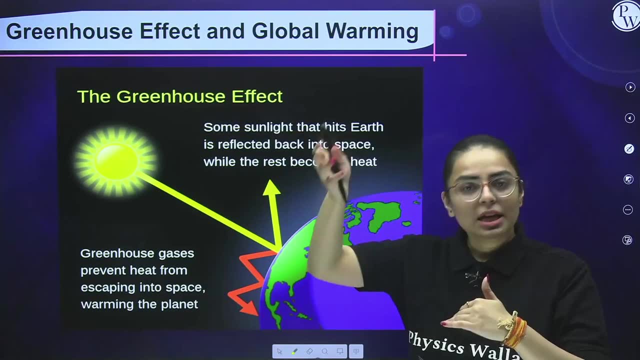 the sun. they, you know, put some harmful rays right, Harmful radiations on earth. Now what happens on earth? Some radiations are being transformed back, you know, They are radiated back, while some of the radiations move inwards the earth. Now what happens? 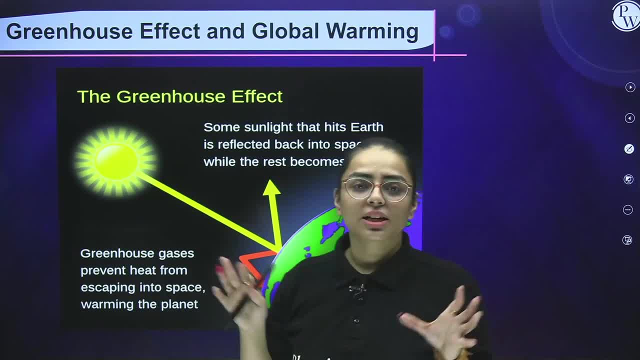 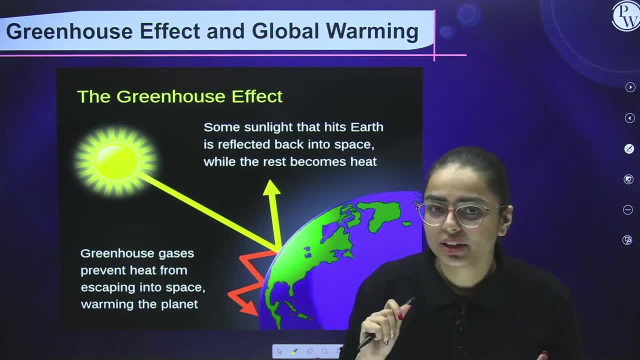 here Previously. what happened? the stratosphere, as we know, contain in that O3 layer, Ozone layer Now ozone layer. role was to protect the earth from the harmful radiations. Now what happens to here? Ozone layer deflection, you all know right. So what? 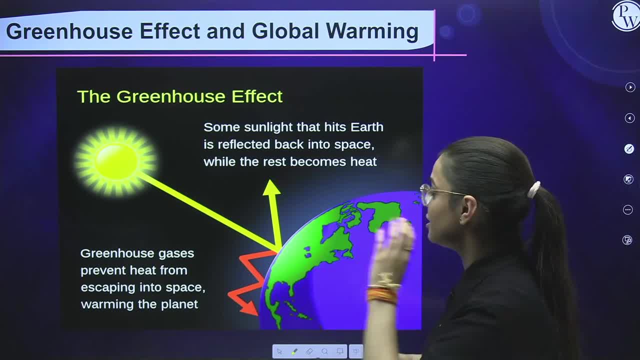 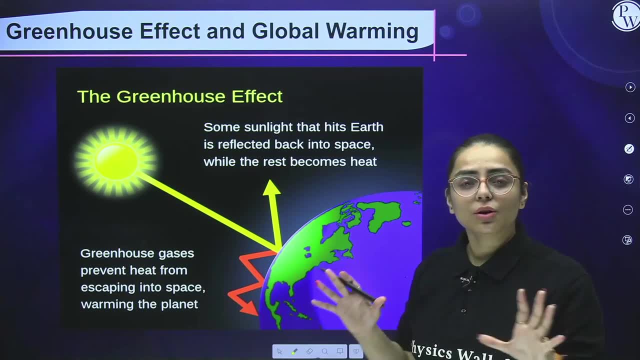 happened over there, When there is a lot of fear of harmful rays approaching towards the earth. Some of the rays you know put go inside. They produces a lot of temperature on the earth. So now what happens in the earth? We know that. We know that. 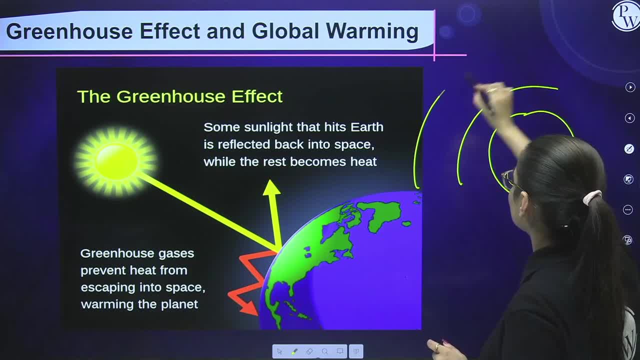 over earth. what happened? We have a troposphere, We have a stratosphere. Now, whenever the harmful radiations come, Some go back while some enter over here. Now, when students, some are entering over here, You know what happens When they enter in the stratosphere: there is 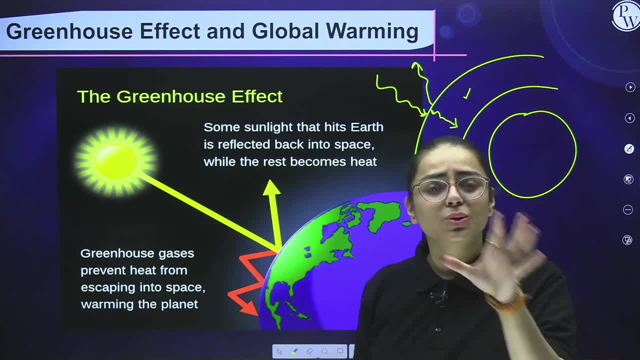 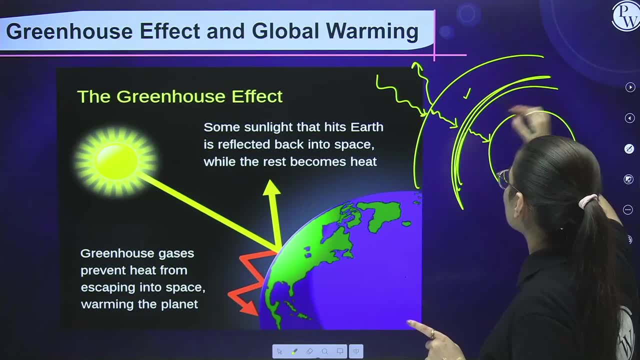 no problem, Because in the stratosphere O3 is present, which is going to protect the earth. But if they enter into the troposphere, students, When they enter into the troposphere- basically what happens Basically in the troposphere- they won't go back. They won't go back. 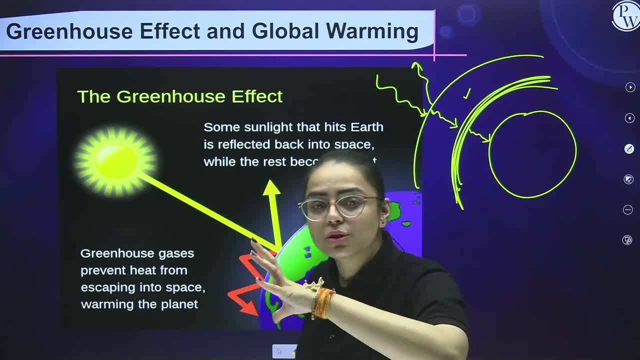 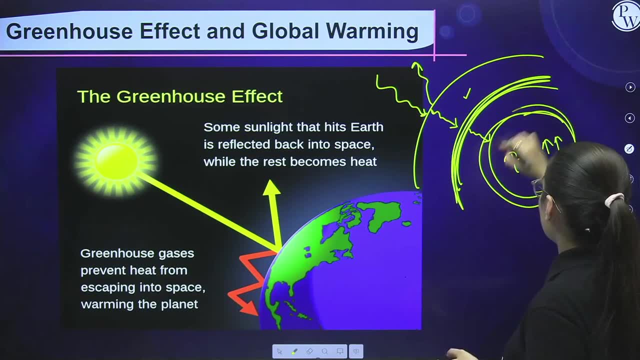 And will produce a harmful amount of a great amount of temperature on the earth's layer. Now, here, a great amount of temperature is produced, Heat is produced, A great amount of heat is produced over the earth. Now what happens? It is trapped. Neither it can go. 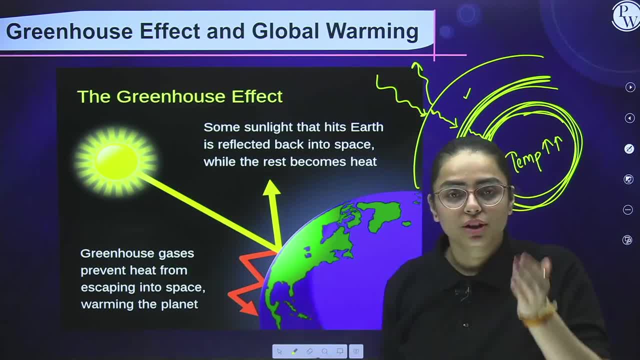 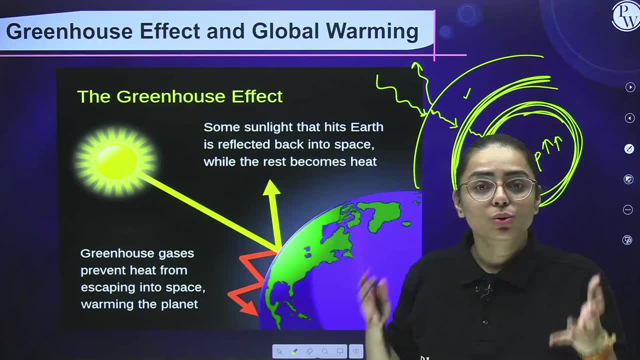 out. You know the greenhouse gases. They don't. they won't let it to go out. The greenhouse gases won't let that. you know temperature to release out And due to, due to this, a lot amount of you know what happens- Temperature increases on the earth. 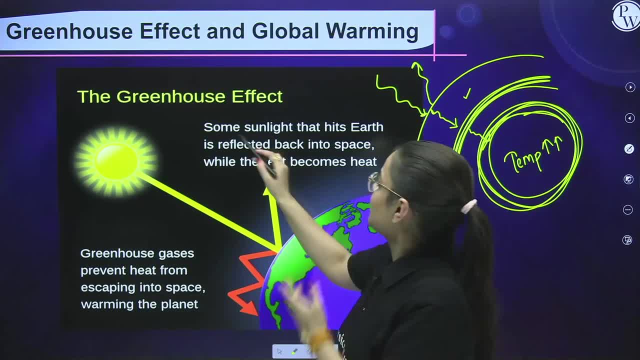 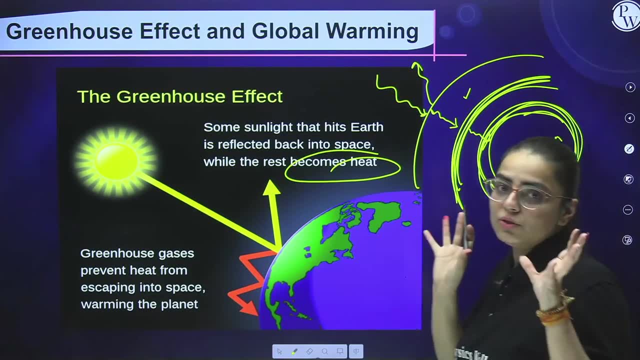 Which causes greenhouse effect. Now let us see Some sunlight that hits earth is reflected back into space, While some becomes heat. Some goes inside and produces lot of amount of heat. Because it is trapped into the troposphere, It should remain in the stratosphere. It is quite easy because 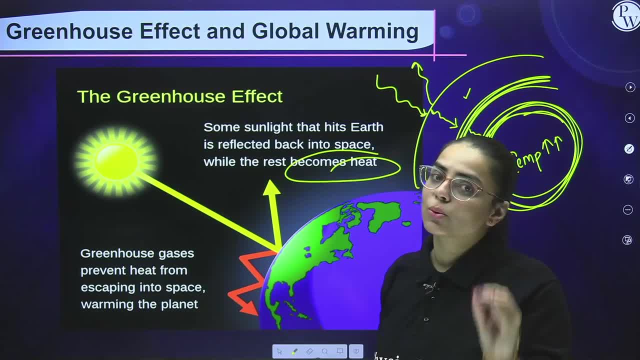 ozone layer will protect, But if it comes into the troposphere it is going to produce a lot of amount of heat. Greenhouse gases prevent heat from escaping into space, Warming the planet Again. this thing I am telling you Now. why does the temperature you know remains so much higher? 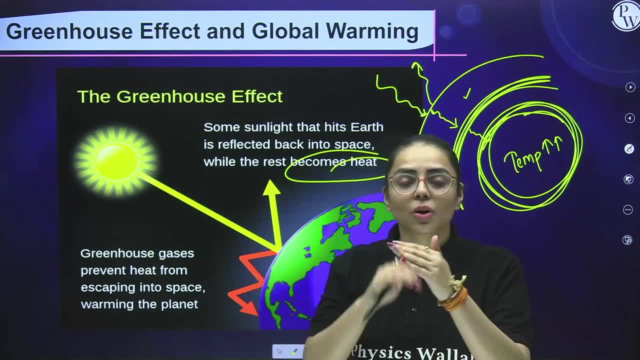 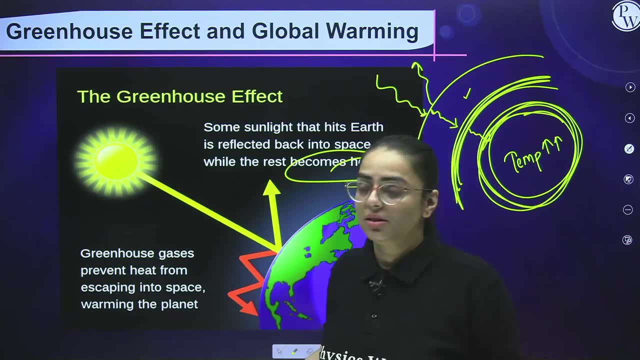 On the earth, Because the greenhouse gases do not let the temperature to move out from the earth into the space. They stop it right. That's why the temperature is increased day by day. There. Now, students, Now students, let us read. This effect was discovered. 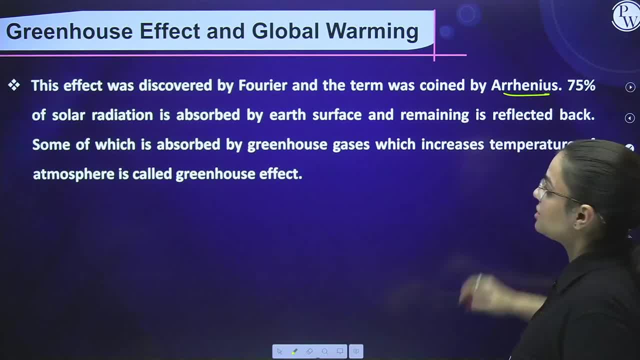 by Fourier And the term was coined by Arrhenius. 70% of the solar radiation is absorbed by the earth surface. They absorbed it How much radiation- 75 you know, And remaining is reflected back. You can see how much radiation is reflected back. 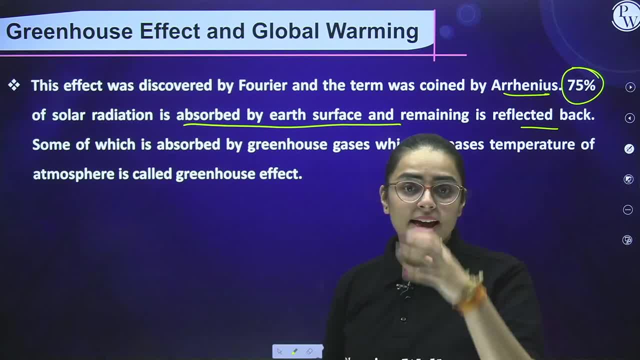 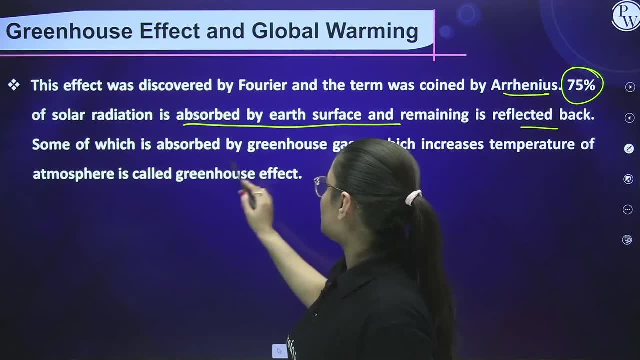 You can see how much is reflected back. 75% is present inside. They come inside the layers right, Some of which is absorbed by the greenhouse gases, Which increases the temperature of the atmosphere, called greenhouse In fact. now this is basically the greenhouse. If I talk about, what are the greenhouse gases? that? 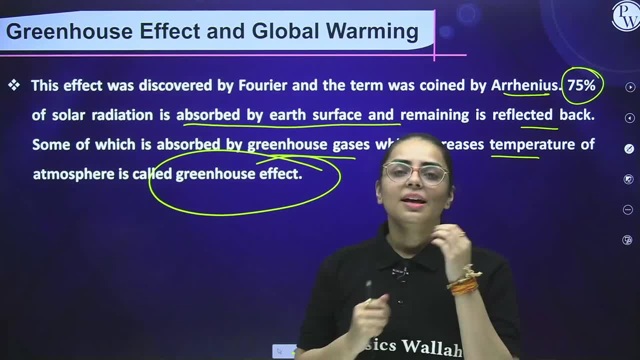 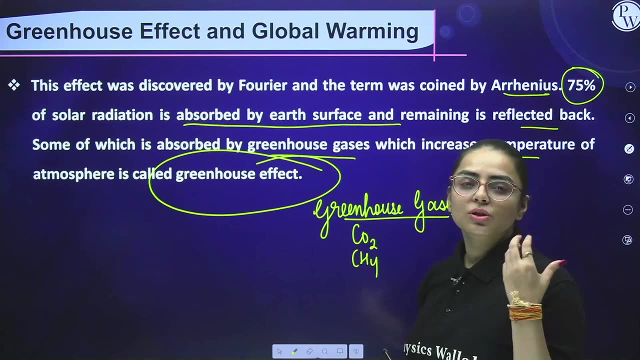 prevent the temperature to move out into the space. It can be CO2.. If I talk about greenhouse gases, Basically it is CO2.. It is CH4. I would say It can be, you know, CFCs. Other than this, it can be O3.. It can be. 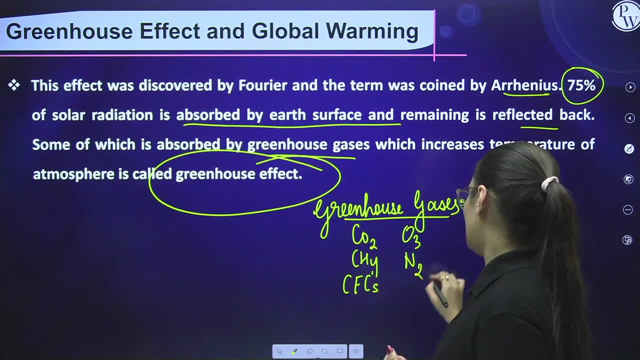 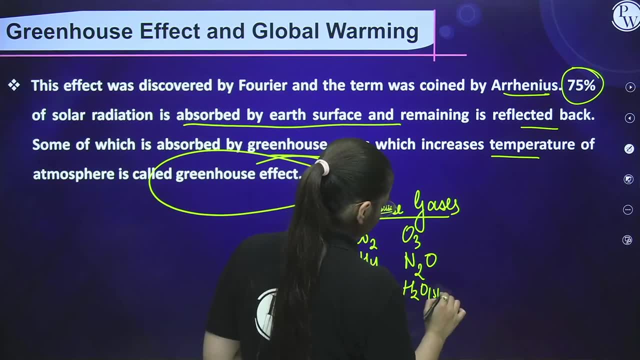 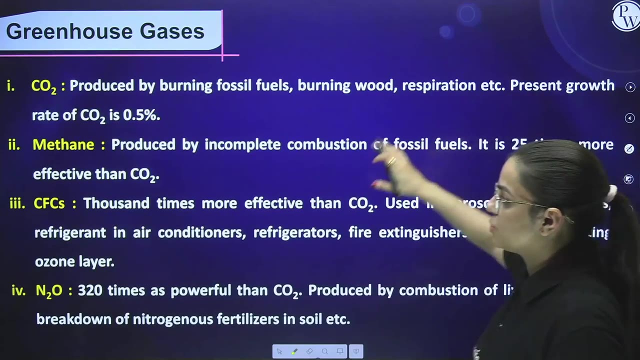 N2.. There can be various examples. You can take water in the form of steam. Yes, they are the greenhouse gases. you know Which causes, Which doesn't let the- basically the heat, the radiations, to move out, right, students Now? Now let us see the greenhouse gases in detail. If I talk about the very first one, it is CO2.. 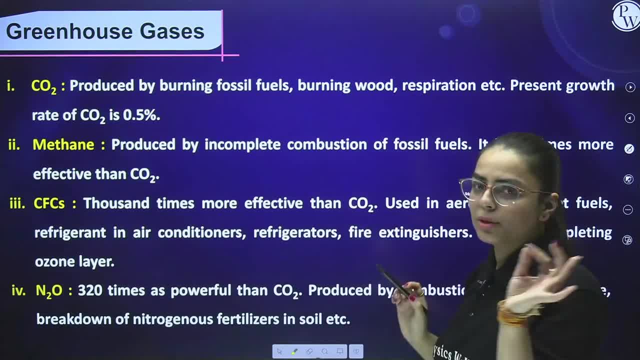 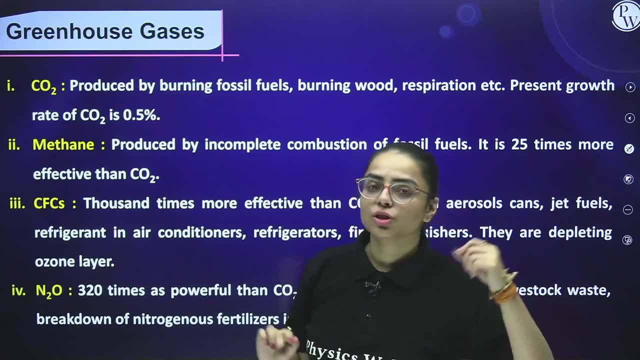 It is produced by burning fossil fuels. They have told you 119 that you need to know. Just know for the knowledge sake. right Now, questions asked from this chapter are also basically theoretical. So I want you all to attempt it in a very good way in your DPP section. 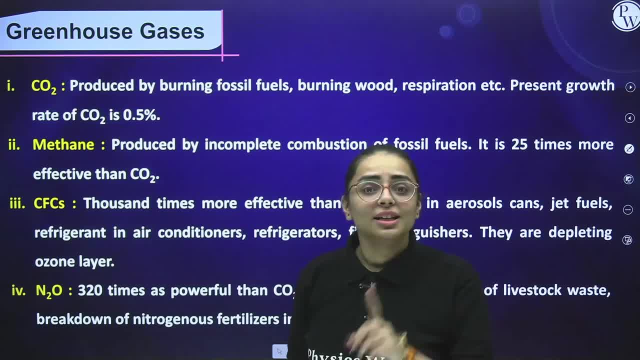 You are going to get a lot of questions in DPP. Kindly solve it okay. It will be a fun for you to do Because it is quite easy. chapter I would say Now, if I talk about CO2.. It is produced by burning. 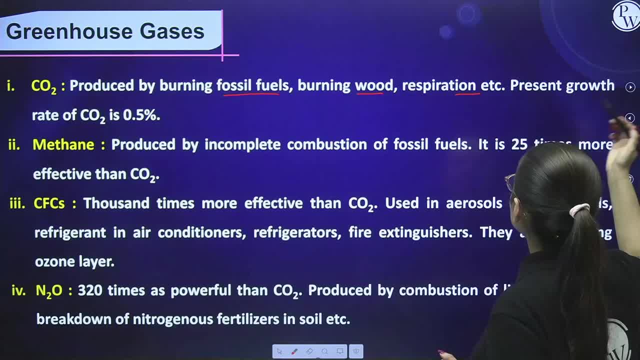 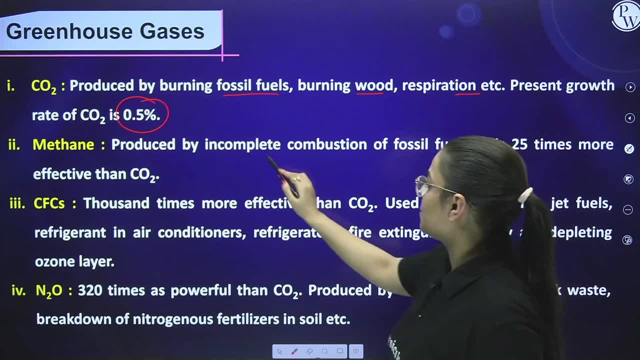 fossil fuels, Burning wood, respiration, etc. Present growth rate of CO2 is 0.5%. you know Okay. Now, if I talk about methane, It is produced by incomplete combustion of fossil fuels. It is 25 times more effective than CO2.. 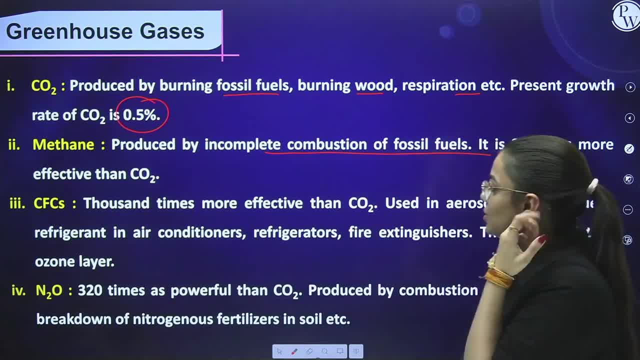 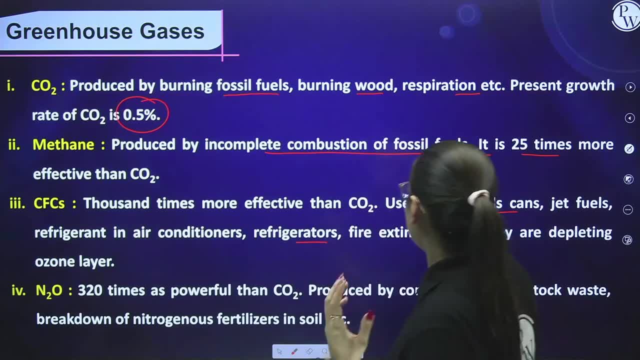 Clear. Okay, If I talk about CFCs, 1000 times more effective than CO2.. Again, used in aerosols, gas jet fuels, refrigerant in air conditioner, refrigerators, fire extinguishers. They are depicting ozone layer, which is really really, really harmful for us. 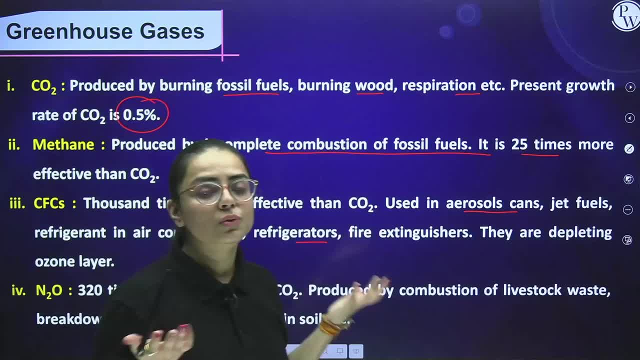 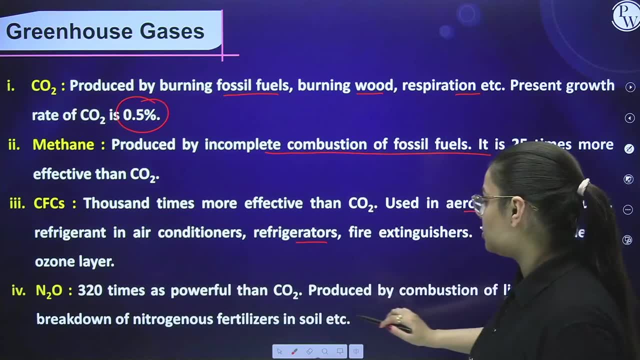 Because if ozone layer is depicting, then who will protect our earth from the harmful radiations? right, Okay, Now if I talk about N2O, 320 times as powerful than CO2.. Produced by the combustion of livestock waste, breakdown of nitrogenous fertilizers and soil extracts, etc. These are the greenhouse gases. 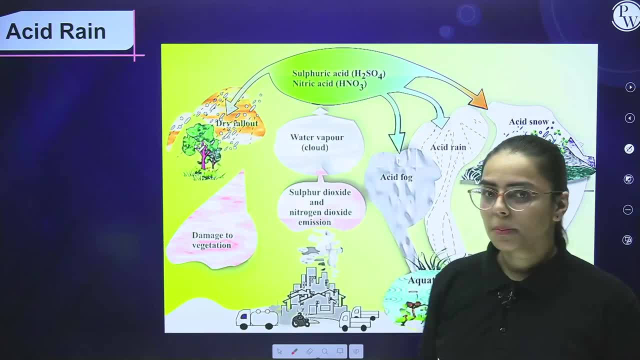 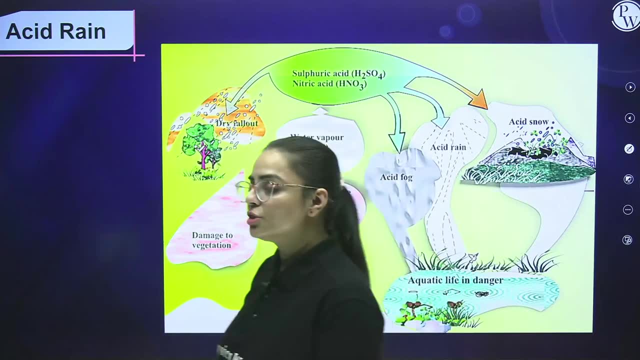 Now comes the next topic, that is, acid rain. If I talk about acid rain, basically In acid rain, we are going to see basically three are responsible for causing acid rain. If I talk about SO2, if I talk about NO2, if I talk about water, Okay, 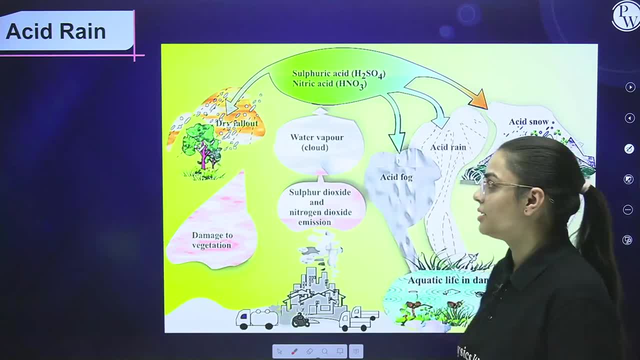 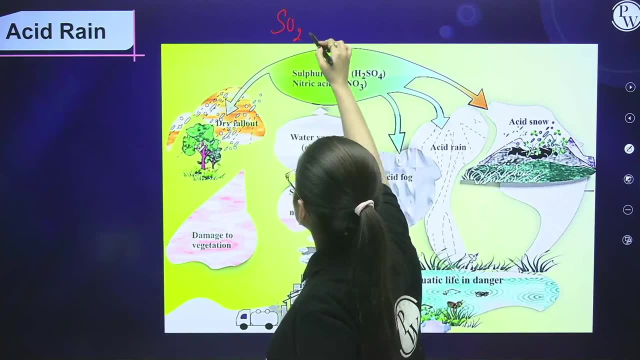 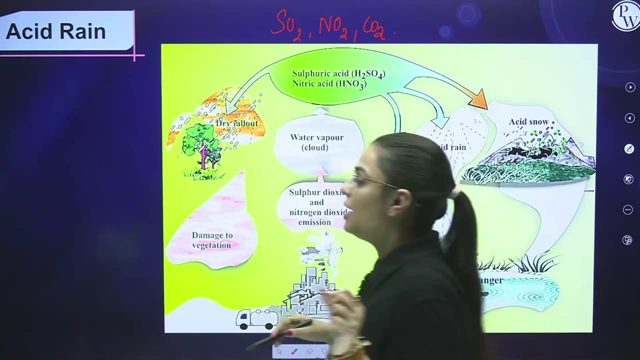 Because all of these are, you know, going to cause acid rain. Sorry, not water, it is CO2.. SO2, NO2 and CO2.. They all are responsible. How they are responsible, students. what is the reason? see What happens over here. when CO2- you know, CO2 from the waste material- 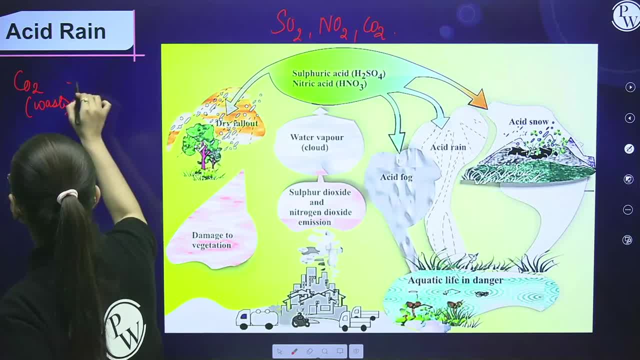 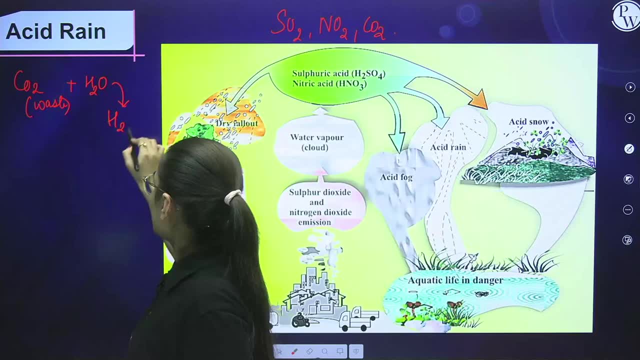 From the waste of the industries, or I would say, When it react with water, it basically forms H2CO3. right, It forms H2CO3 which further splits into H positive plus HCO3 negative. Now, when it is split into H positive and HCO3 negative, 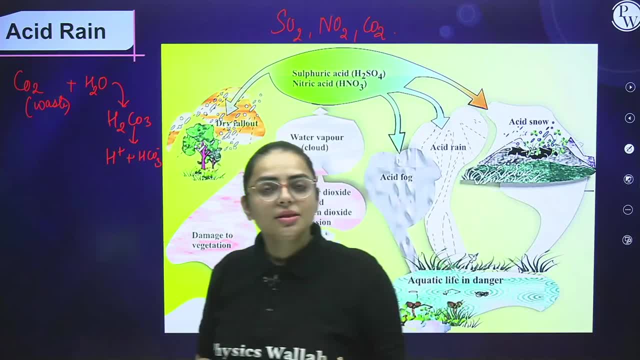 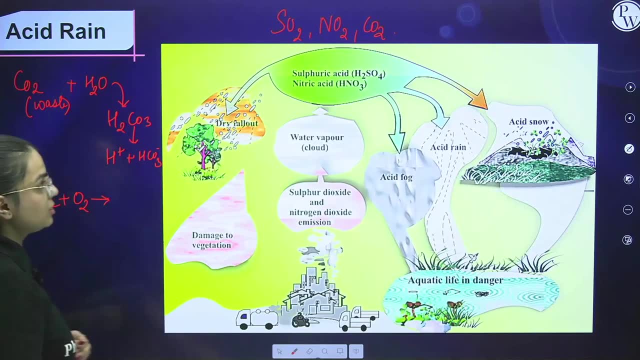 This basically causes acid rain. Other than this, how SO2 is responsible. If I talk about the next reaction, that SO2 on reaction with O2. What does it do See? SO2 on reaction with O2 and with water. Also, with water produces H2SO4. 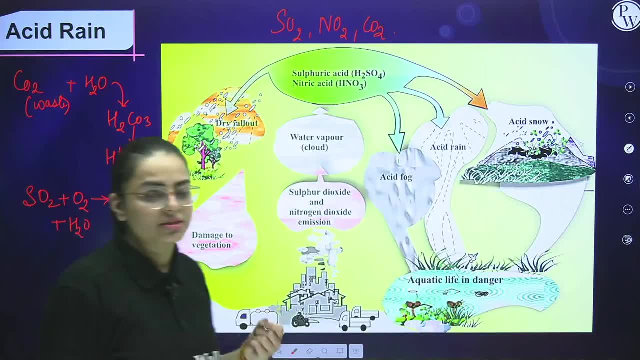 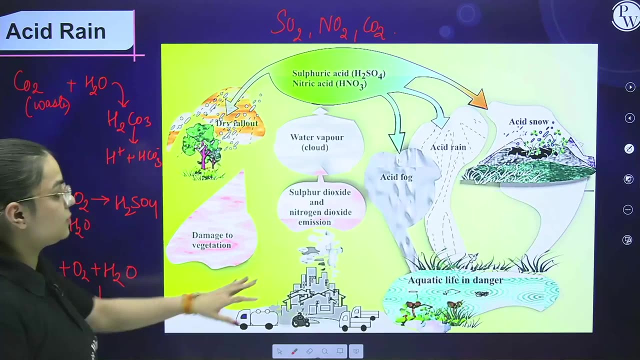 Which is again responsible for causing acid rain. Now NO2 on reaction with O2 and H2. the third reaction: NO2 on reaction with O2.. This also produces HNO3, which is responsible for acid rain. See what happens over here. this is the industrial waste you know. 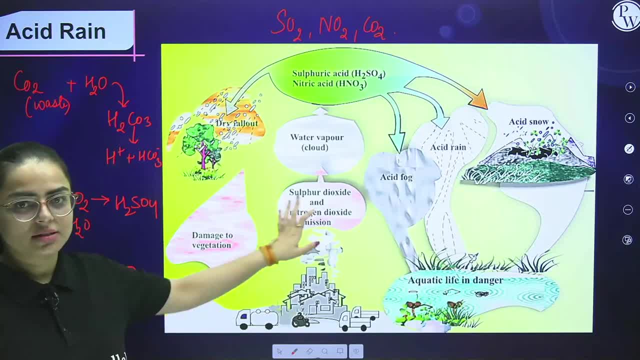 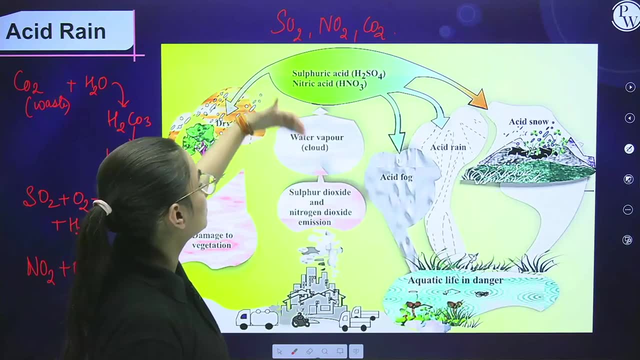 Sulphur dioxide and nitrogen dioxide emission is seen, that is, SO2 and NO2.. And also CO2 is produced. right Now, what happens? in the form of water vapor? they move in the form of a cloud. Then it is being converted in the form of water vapor. that means in the reaction, in the presence of the air. 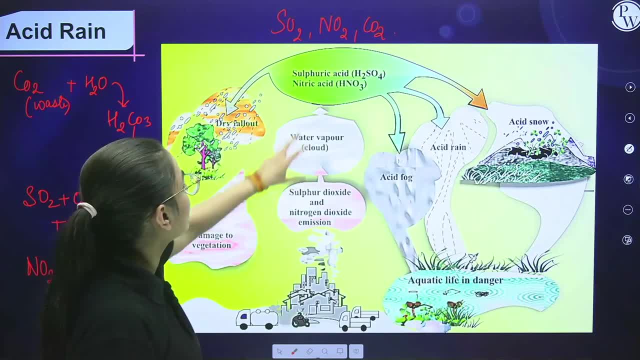 As well as with the presence of the water right. So they react and they form sulfuric acid, that is H2SO4.. Nitric acid, that is HNO3.. Other than this H2, CO3 is also produced. Now these are basically responsible for acid rain, acid snow, as well as acid foam. 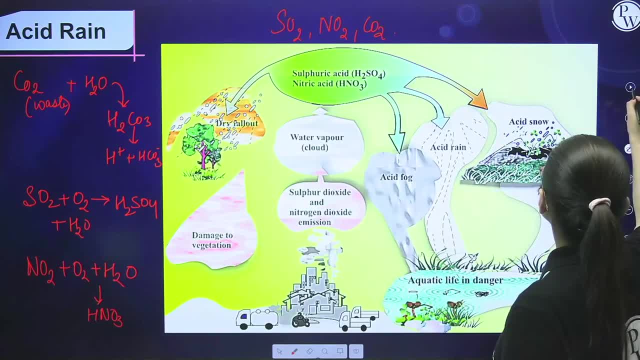 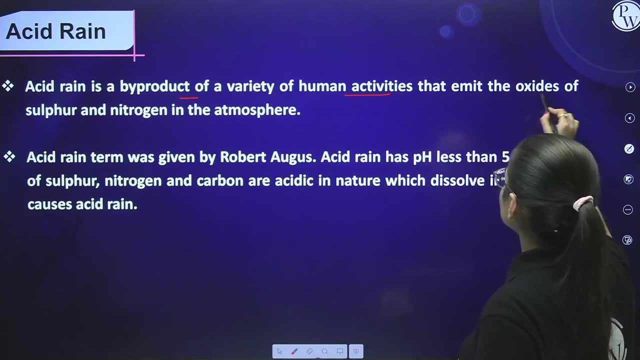 Is it clear to you? Right, great students? So this was about acid rain. let us read over here. Acid rain is a by-product of variety of human activities that emit the oxides of sulfur and nitrogen in the atmosphere, Because it is basically caused due to the industrial waste. 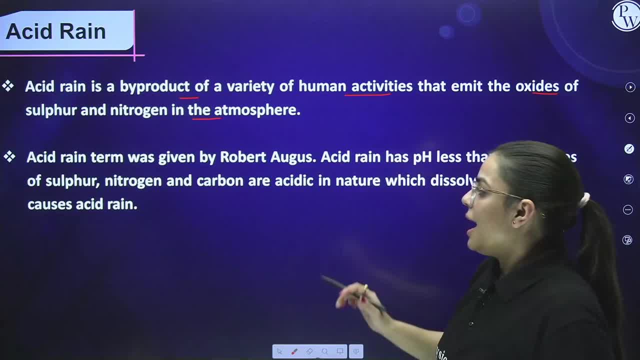 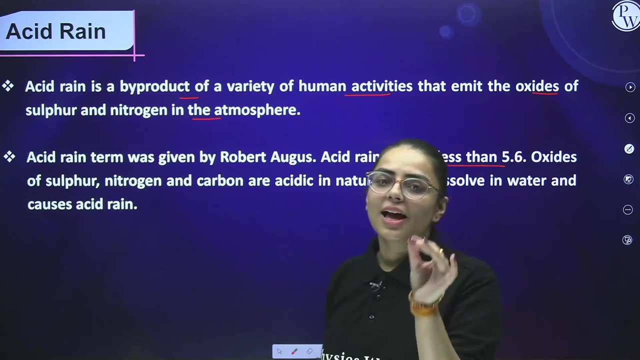 So humans are responsible for that right. Okay, Acid rain term was given by Robert Uggis. Acid rain has pH less than 5.6.. It is quite interesting fact, right. Oxides of sulfur, nitrogen and carbon are acidic in nature, which dissolves in water and causes acid rain. 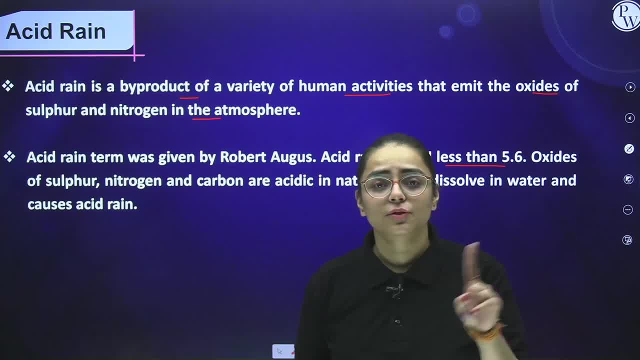 We have seen the reactions When CO2 is reacting with O2 and water, producing H2CO3.. When SO2 is reacting with O2 and water, producing H2SO4.. When NO2 is reacting with H2O and water, it is producing HNO3. 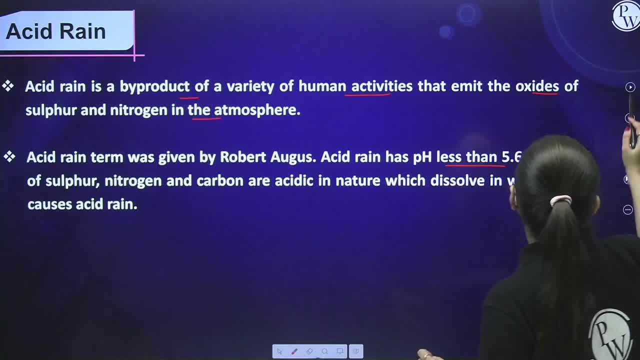 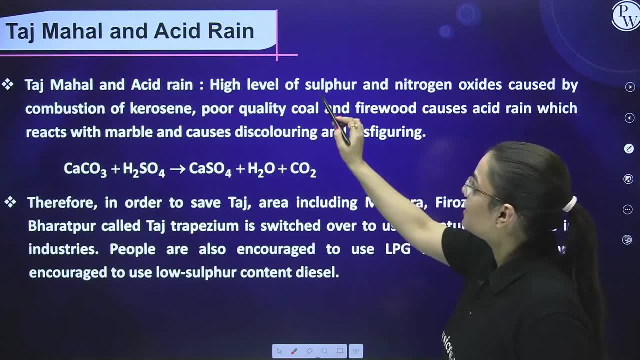 Which causes acid rain? Right, So quite easy reactions. Now, students, come the Taj Mahal and the acid rain. It is quite easy concept. you know: Taj Mahal and acid rain. High level of sulfur. High level of sulfur and nitrogen oxides caused by combustion of kerosene, poor quality coal and firewood causes acid rain. 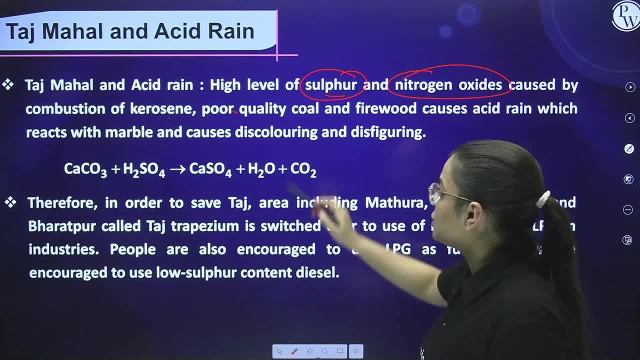 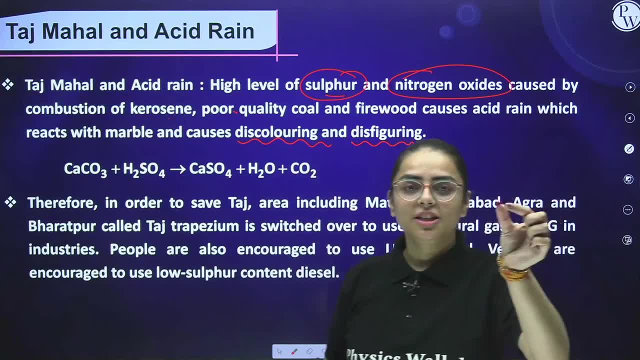 Which reacts with marble and causes discoloring and disfiguring. You know, The Taj Mahal, which was white in color, has been a bit yellowish color, In a bit light of slight of yellowish color. Why? Because it leads to discoloring and disfiguring. 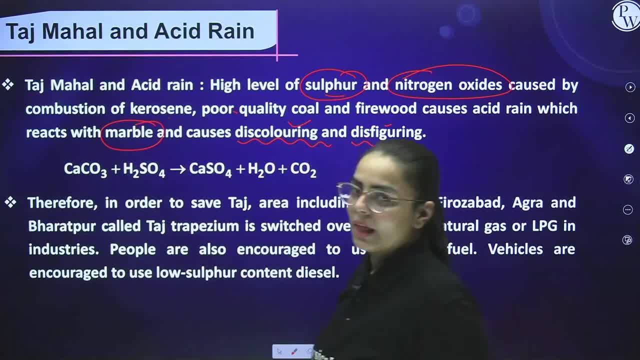 How? Because it reacts with marble. When calcium carbonate reacted with H2O4, it produces CAsO4, water and sulfur. Therefore, in order to save Taj area, including Mathura, Ferozabad, Agra and Bharatpur, called. 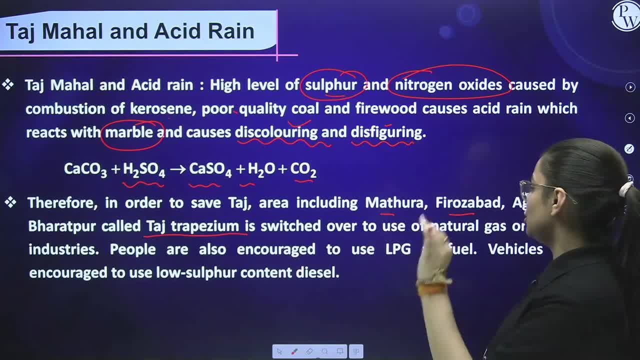 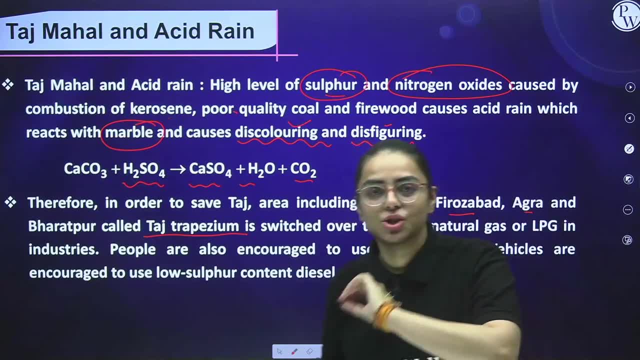 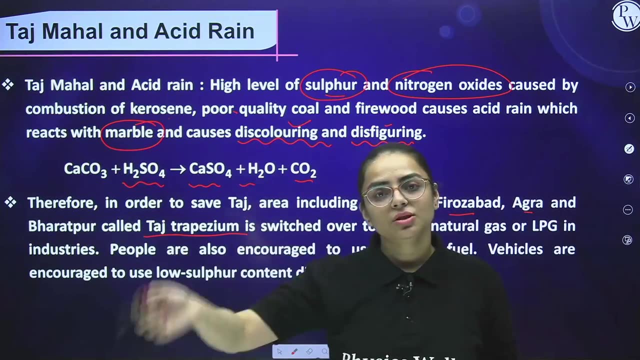 Taj trapezium is switched over to the use of natural gas or LPG in industry, Because it is all caused by industrial pollution. Industry pollution is responsible for the discoloring Because they produces SO2, they produces N2, they produces CO2, which are responsible for acid. 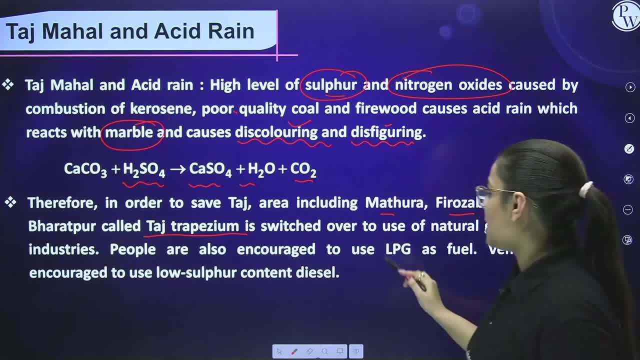 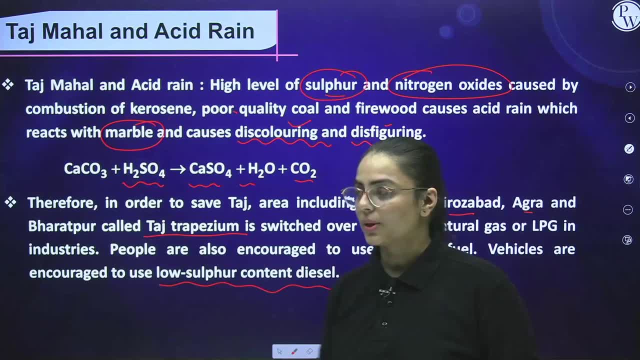 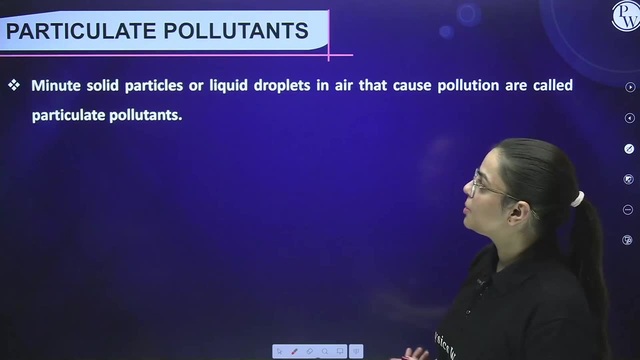 Clear. People are also encouraged to use LPG as a fuel. Vehicles are encouraged to use low sulfur content diesel. Is that clear? Okay, Now students, moving to the next part. that is the particulate. That is the particulate pollutants. If I talk about particulate pollutants, these are basically minute. that means very little. 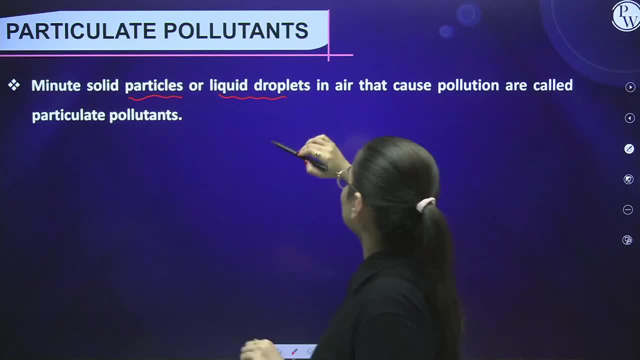 solid particles or liquid droplets in the air that causes the pollution, or called as particulate pollution. Now, what happens over here? For a longer period of time they don't stay in the air, You know. for some time they stay on the ground and whenever the heat, or I would say, the air, 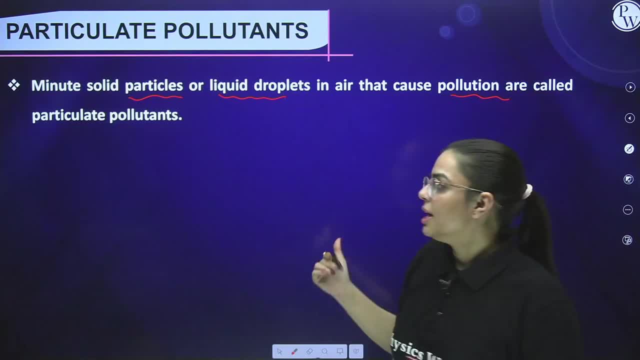 passes on, they are again moving into the atmosphere. Some of the example if I talk about: you know you have water You have heard a word about. you know smoke. You know you have seen about smoke. You have seen dust mist. So particulate pollutants are smoke, dust mist. 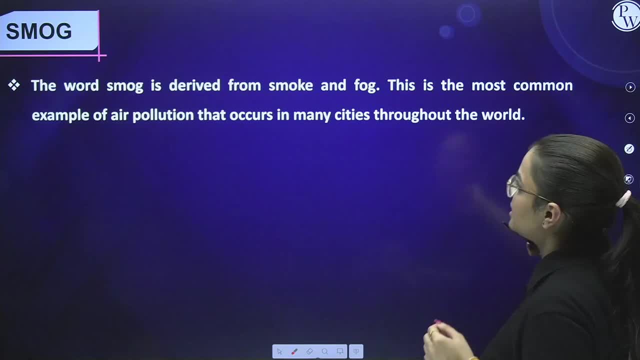 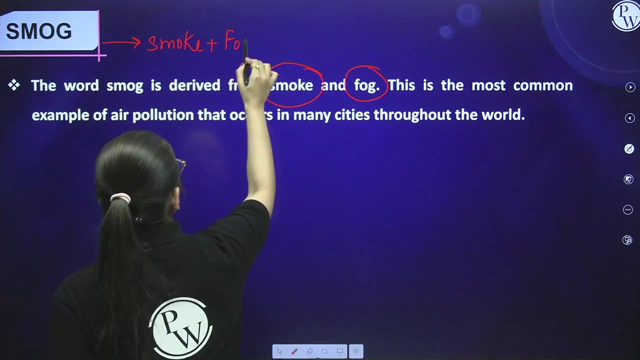 All of these are what Particulate pollutants? If I see the very first, that is smoke. How is smoke obtained, students? Smoke, basically, is a combination of smoke and fog. It is a combination of Smoke plus fog. Now, this is the most common example of air pollution, right? 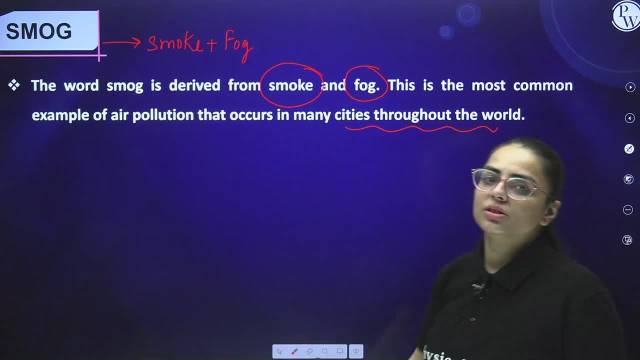 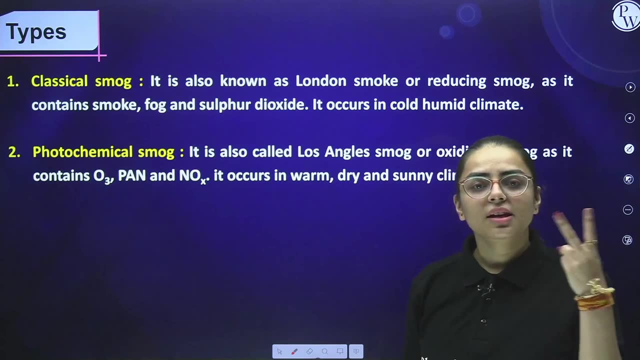 Okay, that occurs in many cities throughout the world. Is it clear, students? Now comes our next part, that is, the types of smoke. you know. These are basically classified into classical and photochemical. One thing that you need to differentiate and you need to remember is classical smoke, basically. 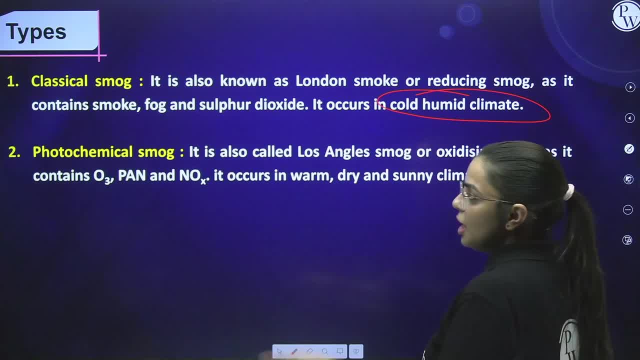 students occurs in cold, humid climate, while photochemical smoke occurs in warm climate. This is really very important. if you put a star mark over here, it will go into be. Now let me tell you about more about classical smoke. Classical smoke is also known as London smoke, or reducing smoke, as it contains smoke fog. 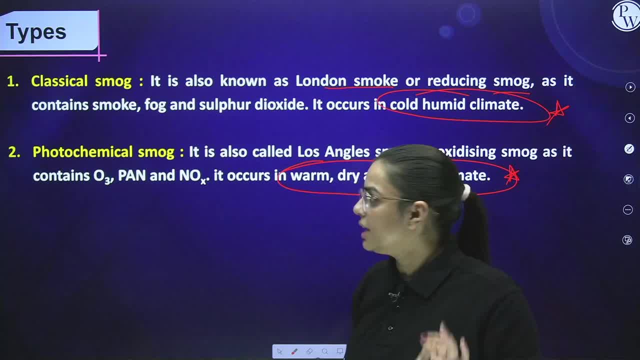 because it is a combination of smoke and fog, So it will have right And sulphur dioxide with it, right. If I talk about photochemical, it is known as Los Angeles smoke or oxidizing smoke. Now, this is reducing smoke, This is oxidizing smoke. 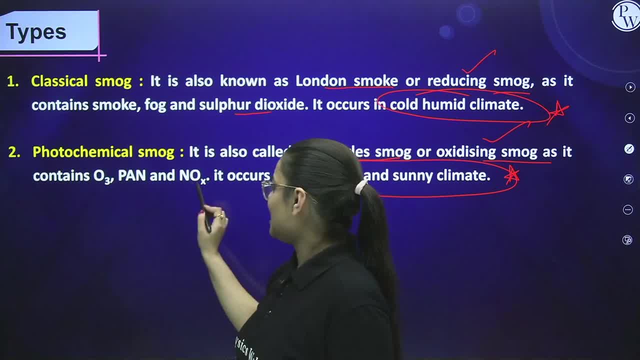 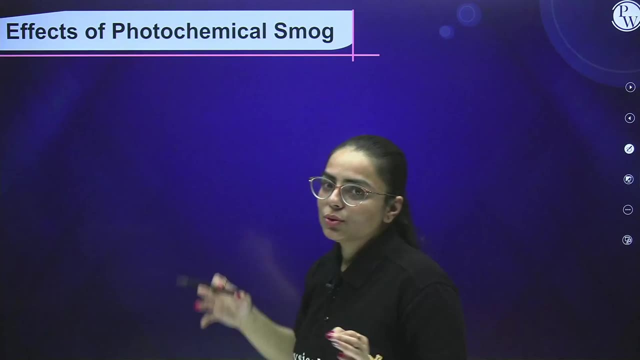 As it contains O3, PAN and NO, you know, nitrogen oxides, oxides of nitrogen particles, and it occurs in warm, dry and sunny climate. So this, basically, is the important part that you need to underline or put a star. Now comes effective photochemical smoke. 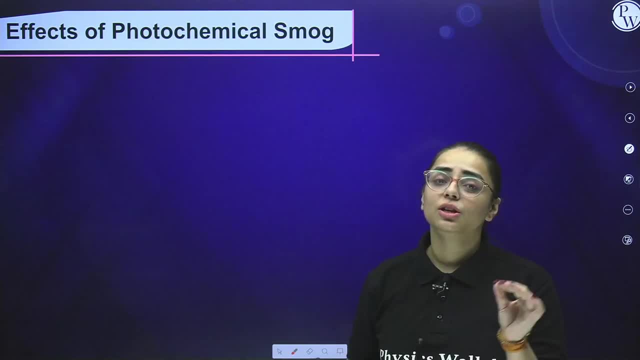 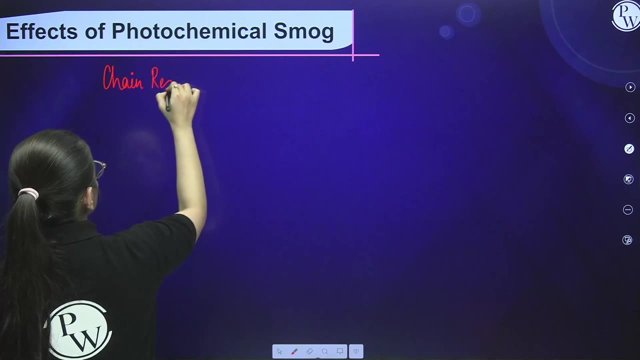 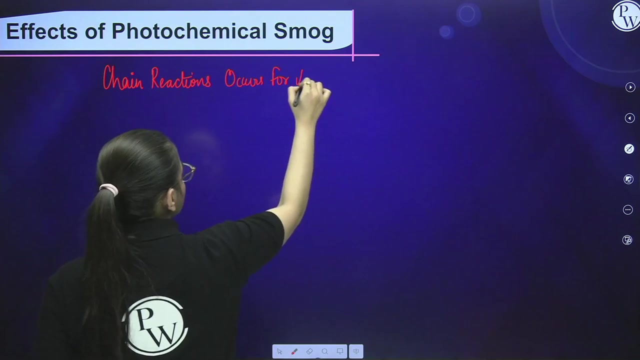 If I talk about effective photochemical smokes, first of all we need to understand what is responsible for photochemical smoke. Basically, if I talk about the formation of photochemical smoke, there is a chain reaction that occurs over here. Now what happens? How is chain reaction observed? 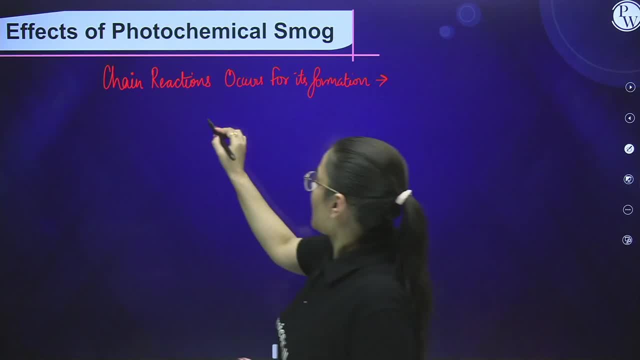 Now see if I say NO2- basically, you know, photochemical, that means that occurs in the presence of sunlight, Is it clear Now what happens over here? See if I take NO2, which is a gas, you know, in the presence of sunlight, what happens over? 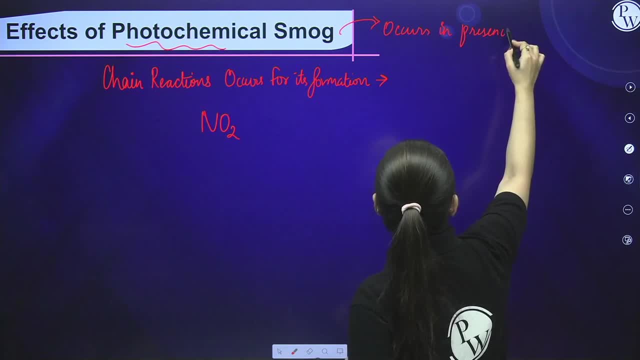 here. That means in the presence of sunlight. that means HNO energy, right, So it splits into NO as well, as nascent oxygen is produced over here. This is nascent and this is the gas Oxygen. this is what This is nascent oxygen. Now, what happens This nascent oxygen further? 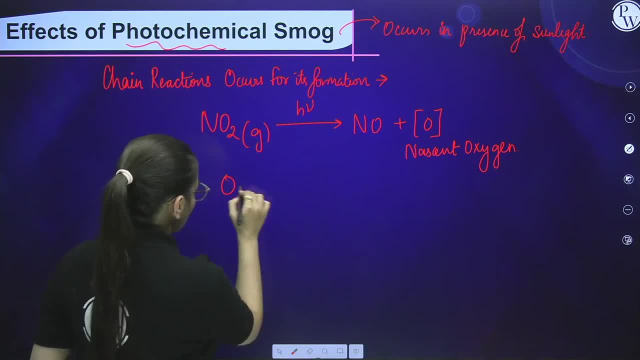 combination with oxygen. you know, O2 forms ozone, That is, O3 forms ozone. Now what happens? NO on reaction with ozone. We have already seen this reaction. NO that was produced here on reaction with O3 forms. what Forms? NO2 as well as forms O2.. Now NO2: we know that it is a. 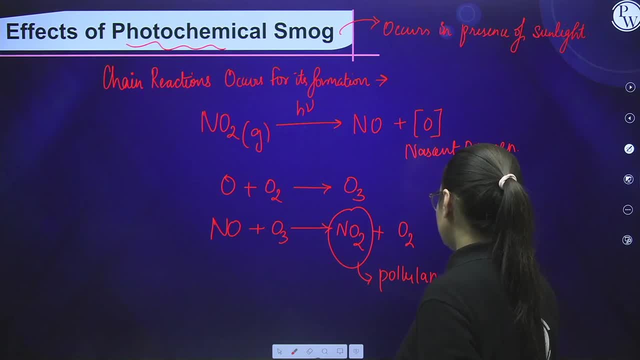 pollutant gas. This reaction we have already seen before. This is a pollutant gas which is responsible for causing pollution. So what is happening over here? See, you took NO2 and the reaction was occurring, and after that, at the end of the reaction, again NO2 is produced. So this is. 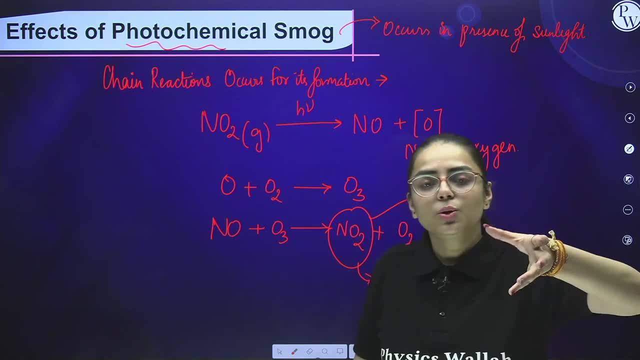 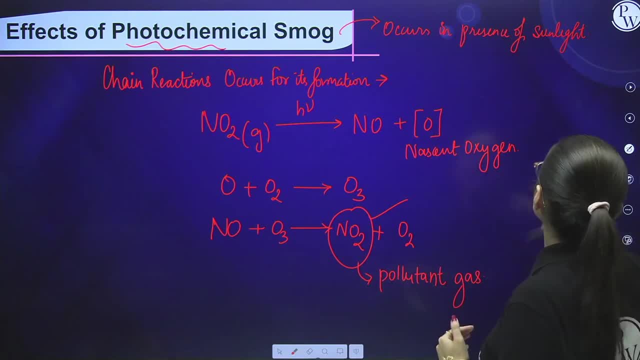 and again a pollutant gas is being produced. Is it clear? Is it clear? So this is basically responsible. The effect for this is because pollutant gas is produced, it will cause respiratory problems, other problems, you know. So, yes, now students comes. how can photochemical smog be? 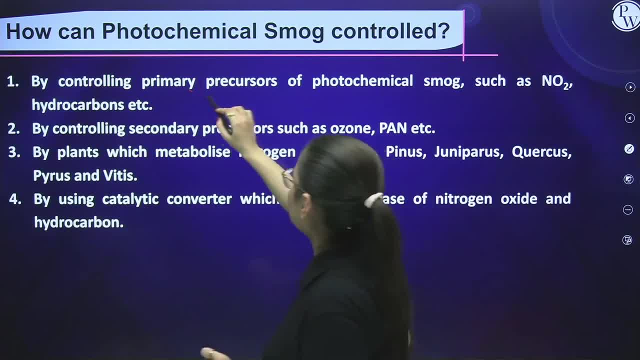 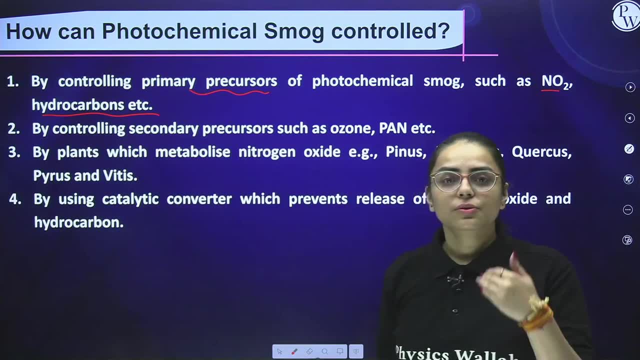 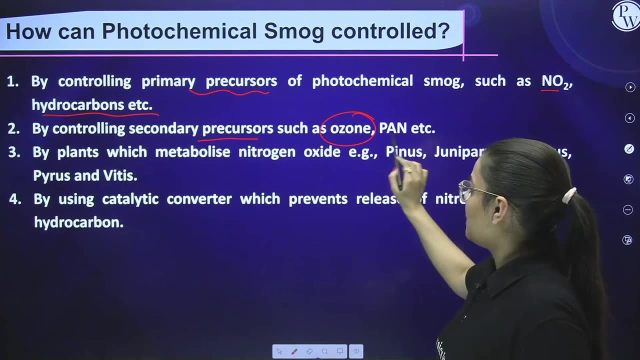 controlled, you know, by controlling primary precursors of photochemical smog, such as NO2, hydrocarbons. If we can control these all, so we can control the further reactions also. First, by controlling secondary precursors, such as ozone fan, etc. Third is by plants which metabolize. 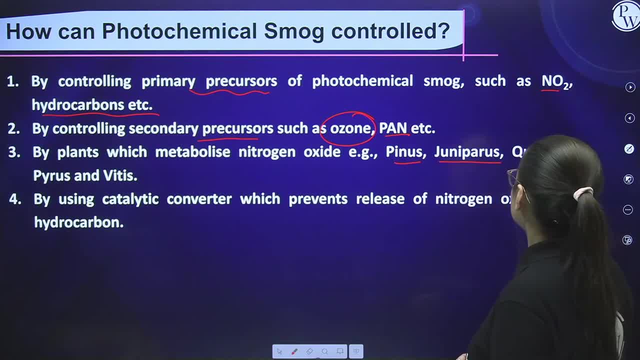 nitrogen oxide. Example: Pinus Juniperus. you know all of these plants, Pyrus Victus, all of these which metabolizes nitrogen. These can be used by using catalytic converter, which prevents a release of nitrogen oxide in hydrocarbons. So, this way, these are the ways from which photochemical smog 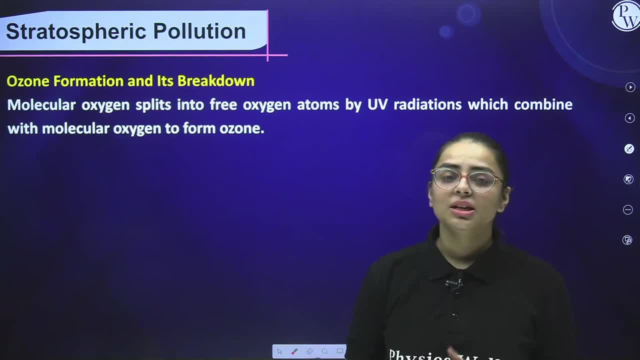 can be, you know, controlled. Now comes the next kind of pollution. We have done the first kind of pollution, that is, the tropospheric pollution. Now comes the stratospheric pollution. Again, stratosphere is basically, when seen from the troposphere it is at a 40 km, but when seen from the earth sea level it is 50 km. right, 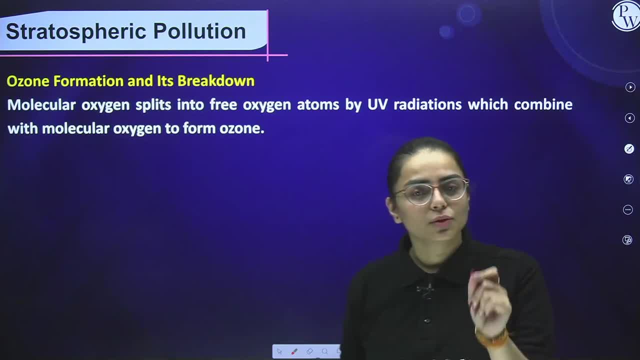 Now, if I talk about stratospheric pollution, what happens over here? I have already told you: in stratosphere ozone layer is present. that means formation of ozone will be seen right. So it says: molecular oxygen splits into free oxygen atoms by UV radiations which combine with molecular oxygen. 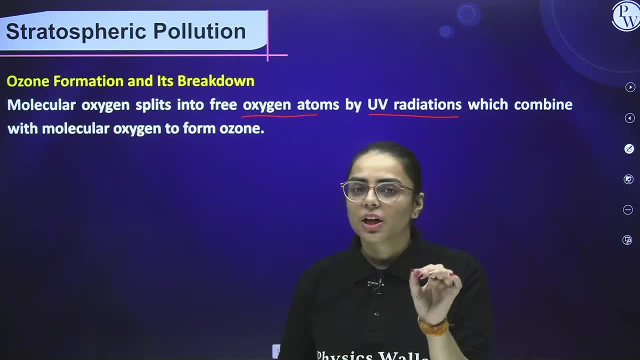 to form ozone. Now, what is this? When this below comes into voluntarily, this reaction, see here, formation and breakage both occurs. Now, if we talk about formation, Now if I am talking about formation, what happens? see, Putu basically reacts with an ozone. that is. 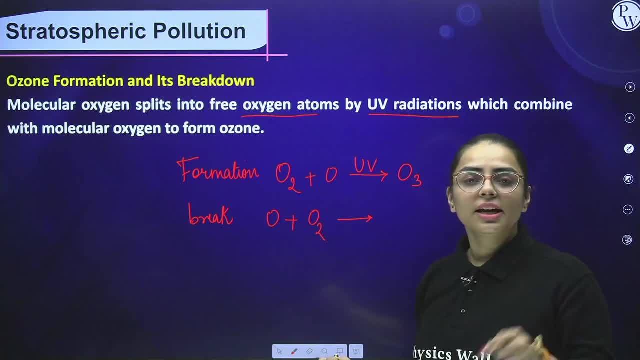 plus O2. basically what happens over here. it again breaks. this reaction was seen, first O3, this was seen, now seen. see this carefully. this was produced. this was the first reaction formation one. now O3 again can be broken into O2 and O. now, basically this happened now when 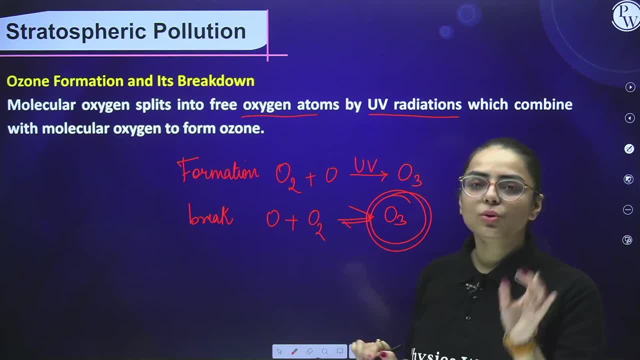 there is a depletion in the ozone. the depletion in the ozone is responsible for the formation of free radical. okay, now, which is also not good for us. why it is not good for us? because ozone is protecting our earth from the harmful radiation, and if ozone is, you know again. 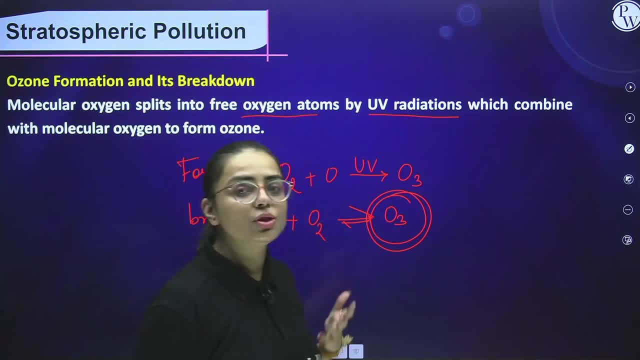 depleted into again. it is, you know, decomposed into oxygen and O2. the deflection level basically leads to the formation of free radical, which will cause pollution. clear now, students: if I talk about the effects of deflection of ozone layer, what happens over here if I talk? 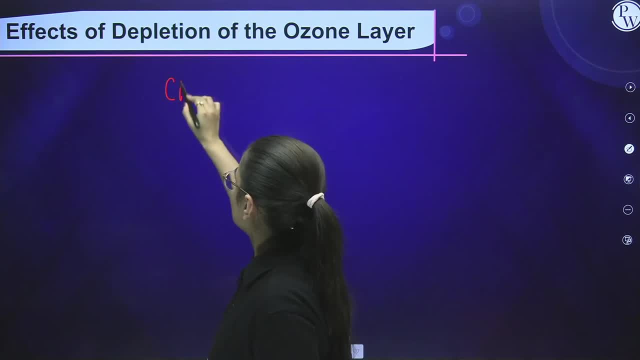 about fluorofluorocarbons, CF2, CL2. now what happens in CF2- CL2? I have already told you that free radicals will be produced. so what is the very first free radical which is produced over here? CL radical is produced over here, and other than this, yes, if one CL is taken. 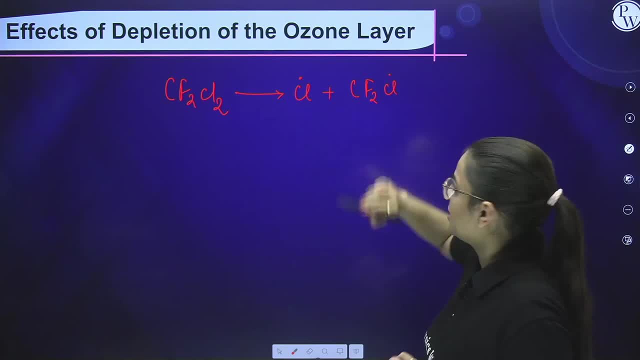 out, it will be left with CF2CL radical right now. what happens now, students? we know that there is O3 that is being produced in the previous reaction. so what will happen? this CL radical basically combines with the ozone. now, when this is combining with ozone, it will 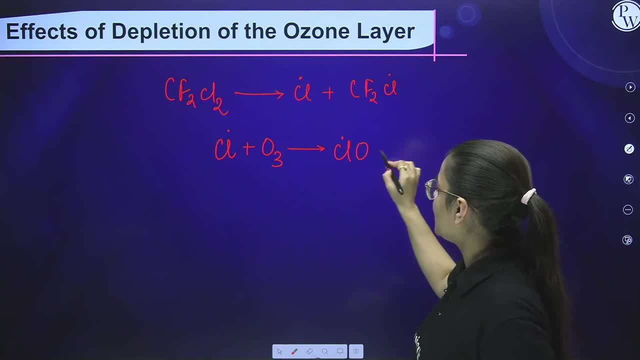 lead to the production of CLO radical plus NaFeO radical, which is the reaction of O2 and O3, which is the reaction of O3 and O2, which is the reaction of O2 and O3, which is the reaction of O2 and O3, which is the reaction of O3 and O3, which is the reaction of O3. another 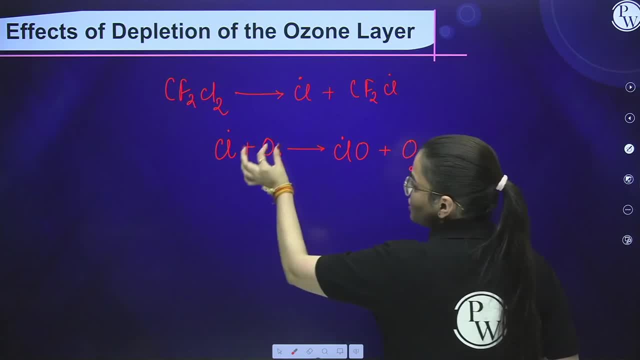 thing will happen is that O2 will be released. one oxygen will combine with this, while two oxygen are left over. which form O2? now, what happens over here? here? you know that this O2 is produced in now stratosphere. it is being produced in stratosphere and when it is being. 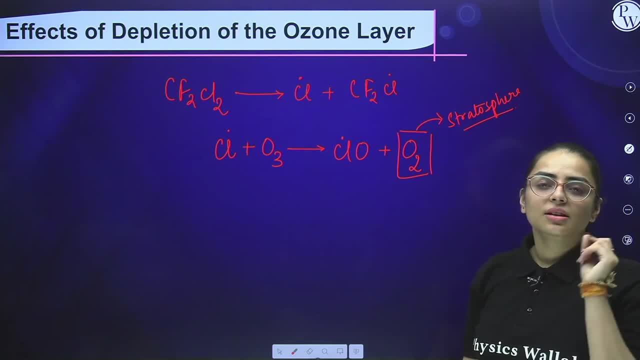 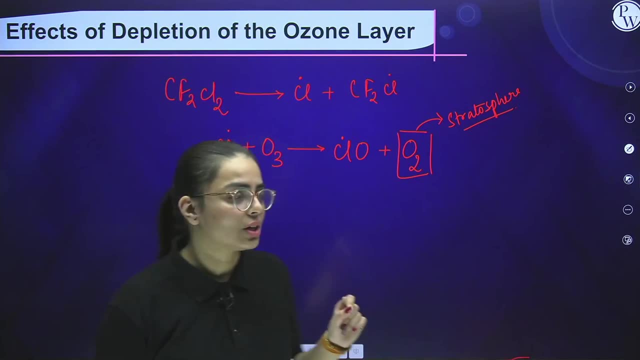 produced in the stratosphere. it is really, really bad because it will consume O3. it will consume O3, so this is harmful. this is this is the thing that we both require. other than this, students, other reaction can also occur. this is the thing that we both require. other 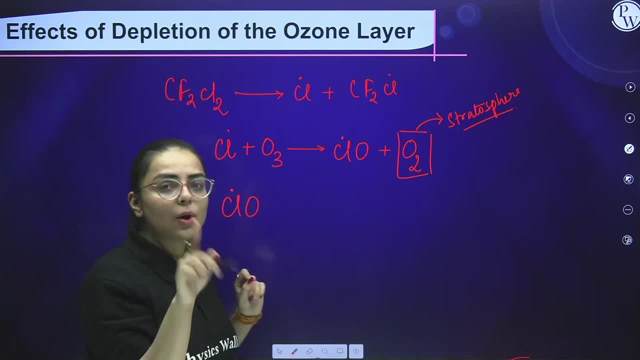 can be seen is that this CLO radical basically now it reacts again with O2, again with this O2 it will react, it will lead to the production of CL radical plus O2.. So this O2 that is produced basically will consume ozone, and when it will consume ozone, 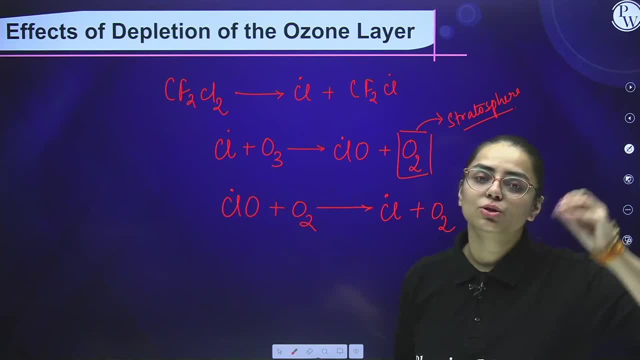 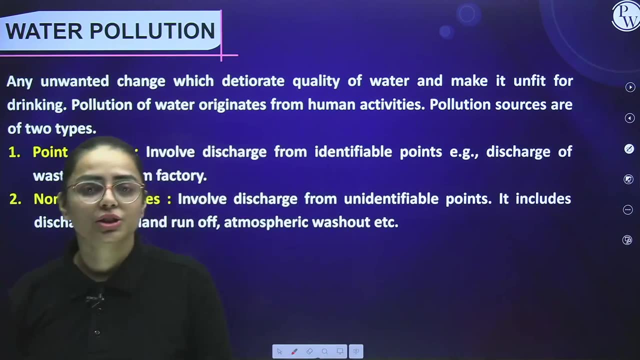 ozone will be less. it will be deflected, which will lead to the pollution Clear. Okay, students, now comes our next kind of pollution, that is, water pollution. We have already done air pollution. I want you all to take 5 minutes and revise quickly. till then, I will take a glass of water. 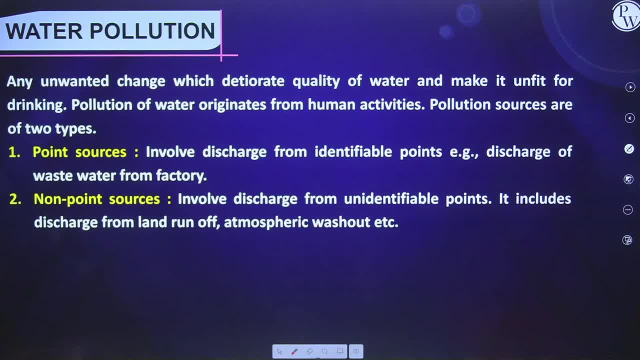 Right, Okay, students, I hope so. you have revised it and I know that there is no need to revision, also because it is the concept that we have started already. Yes, there are some reactions, but if you will open your NCRT, you will be very clear with 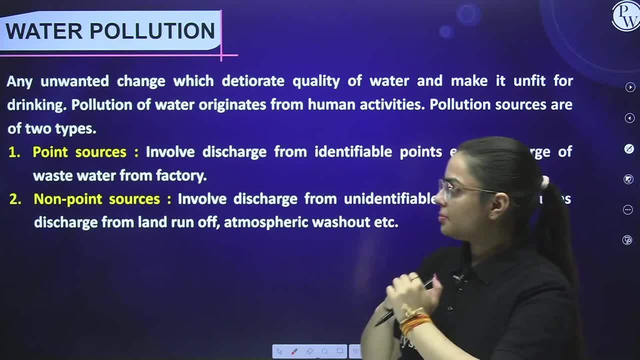 each and every reaction and with my lecture, right Okay, now comes our next kind of pollution, that is, water pollution. Now again, when there is an undesirable change, you know, which affects the quality of water, right, Which will cause How. 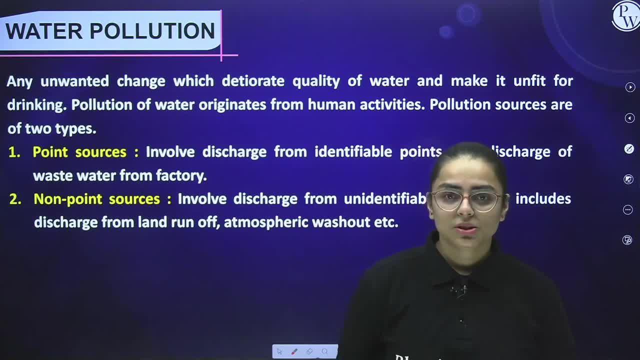 How harmful effect in the drinking in the, you know, the sea animals. they are affected by this. so that is water pollution. Now let us see any unwanted change which causes, which deteriorates or, you know, reduces the quality of water and make it unfit for drinking, due to that which we are unable to. 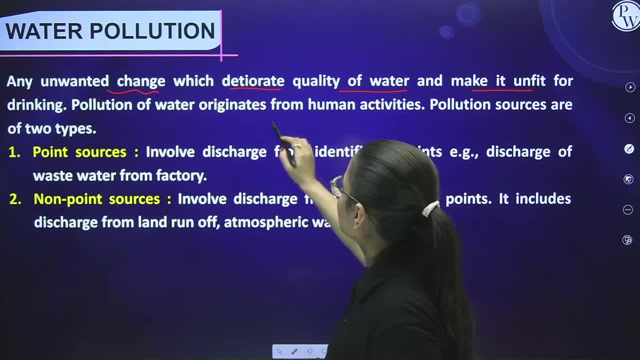 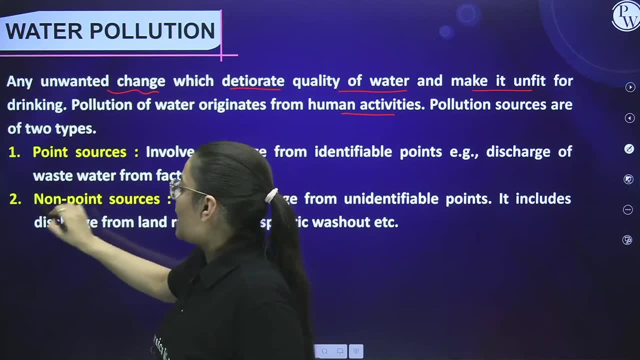 drink that water right. Pollution of water originates from human activities. Pollution sources are of two types. now over here in the water pollution it is point sources and non-point sources. If I talk about point sources, It involves discharge from identifiable points. example, discharge of waste water from factory. 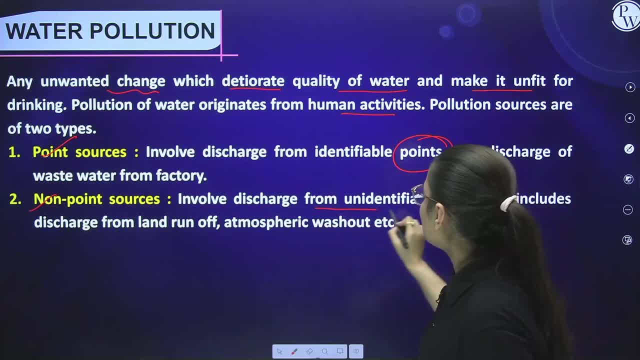 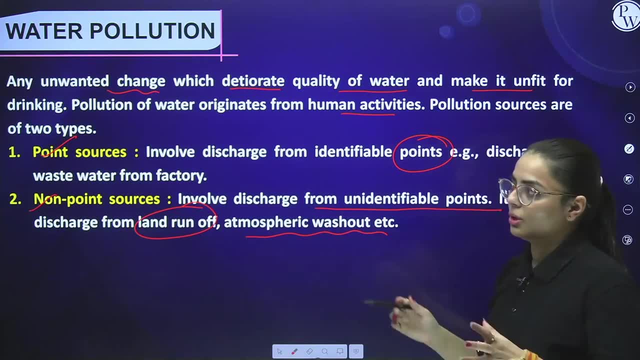 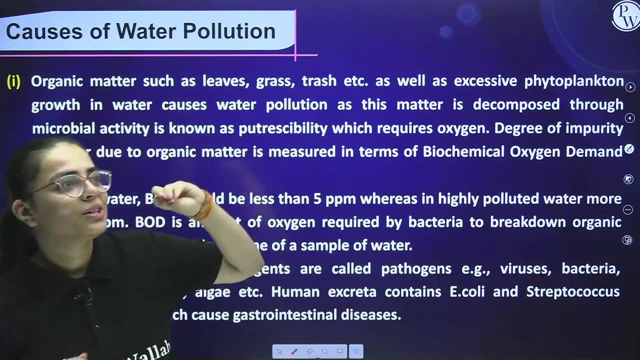 Now, if I talk about non-point source, involving discharge from unidentifiable points, it includes discharge from land runoff, you know, from atmospheric washout, these all. So these are of two sources. right, If I talk about the causes for water pollution, I know in your smaller classes you would. 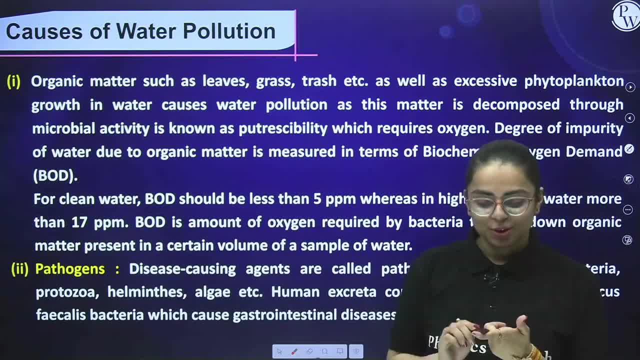 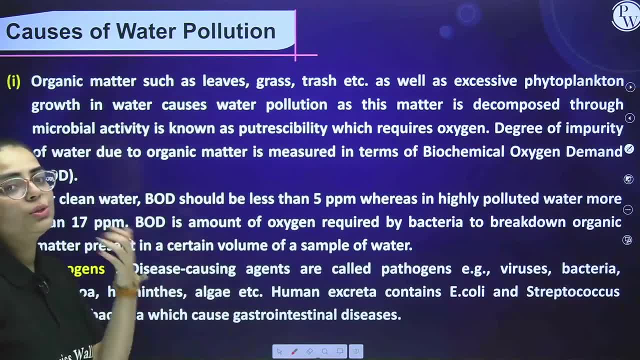 have written the essays on this right. What is water pollution? What are the causes, What are the effects? So you all are familiar with this, but still, I will be reading for you, because there are some things that you will need to know, okay, which you do not know in the previous classes. 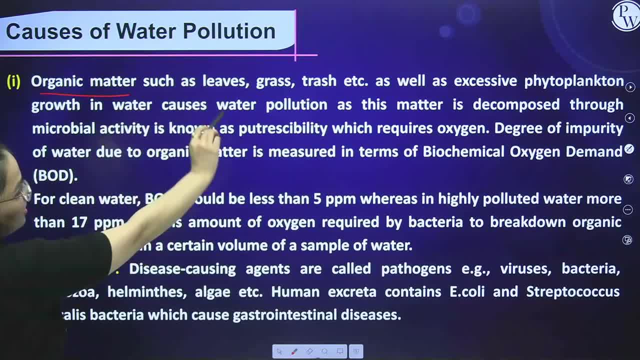 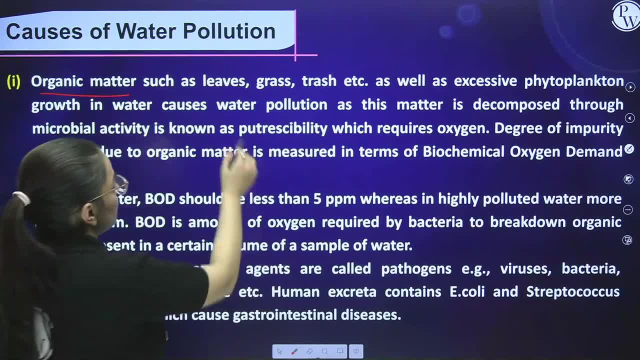 So very first cause of water pollution is organic matter such as leaves, grass, trash, as well as excessive phytoplankton growth in water. they causes water pollution. you know Now this is really important. this is a quite different concept, right as this matter is. 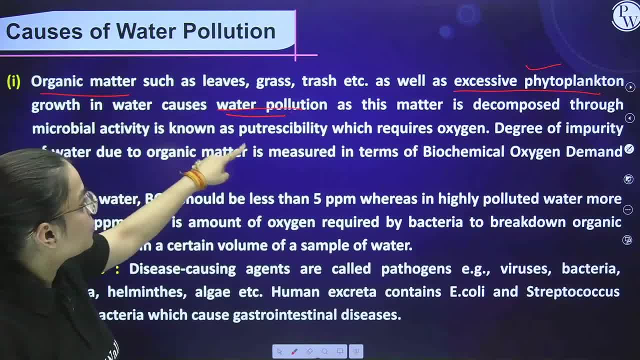 decomposed through microbial activity. So what happens? The microbial activity is known as produceability, which requires oxygen. degree of impurity of water due to organic matter is measured in the terms of BOD, that is, biochemical oxygen demand. Now, to check the degree of impurity in the water, you need to know about the bio you. 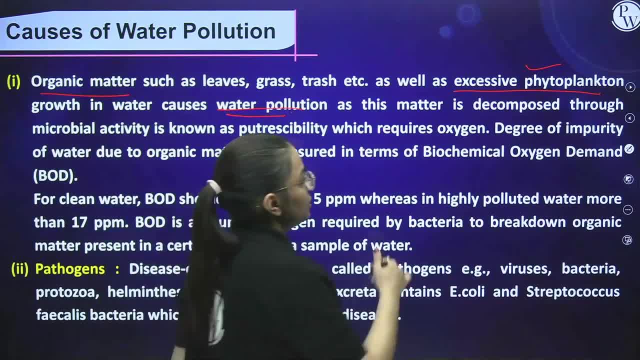 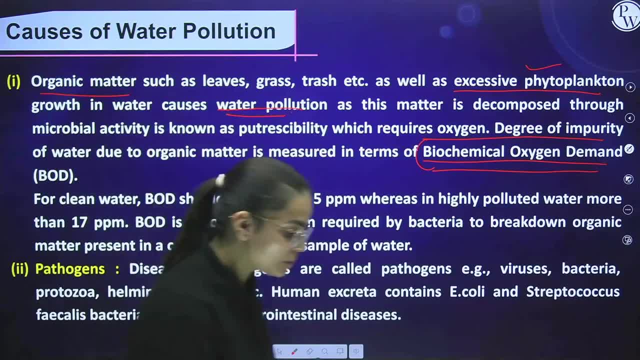 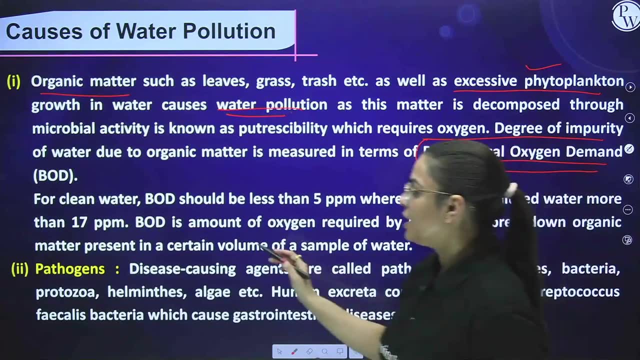 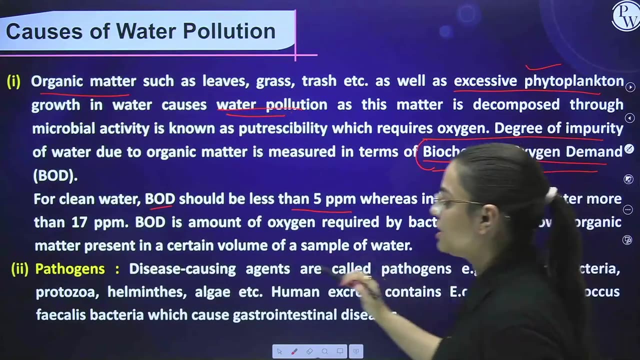 know you need to know about biochemical oxygen demand, that is BOD. Now what happens here? For clean water, BOD should be less than 5 ppm, that is, parts per million, whereas in highly polluted water it should be 5 ppm. water it should be more than 17 ppm, that is, 17 parts per million. POD is the amount of oxygen. 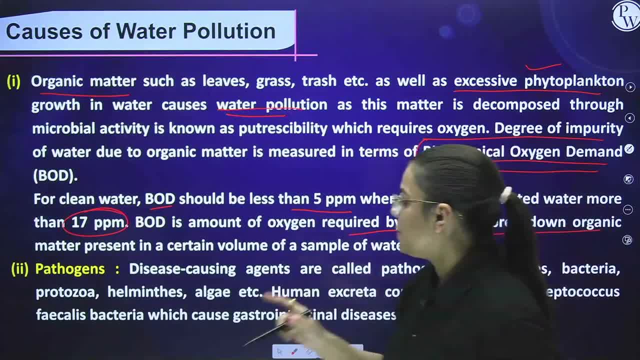 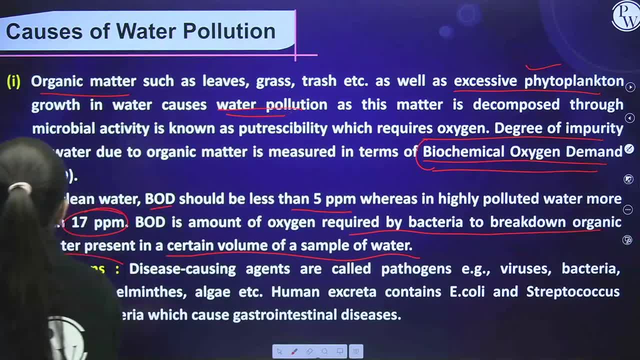 required by bacteria to break down organic matter present in a certain volume of a sample of water Clear. Now comes the next cause, that is, the pathogens. The very first was organic matter. right, just, for example, leaves, trash, all of these stuffs, or we can say as well as the excessive. 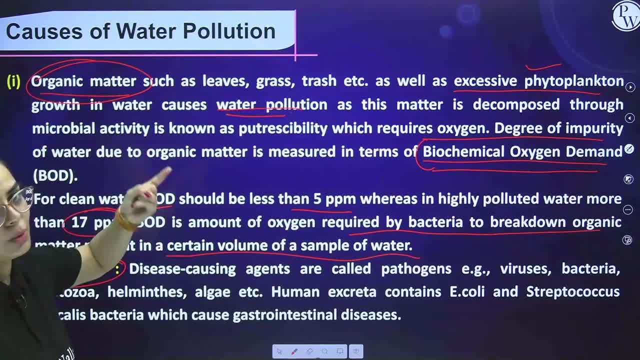 phytoplankton that has been growing in the water, which causes water pollution. Now comes pathogens. Disease causing agents are called pathogens, for example, virus, bacteria, fungi, or if this protozoa, algae, Human excreta contains E coli, you know, bacteria and streptococcus. 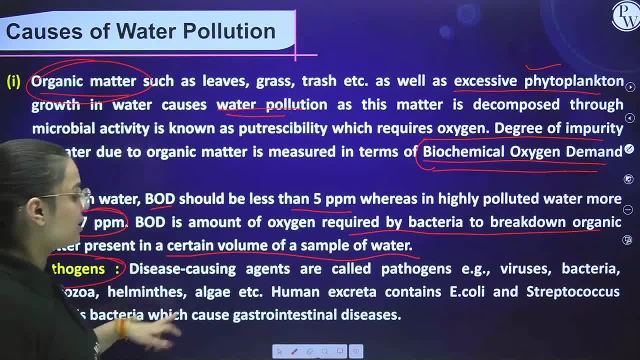 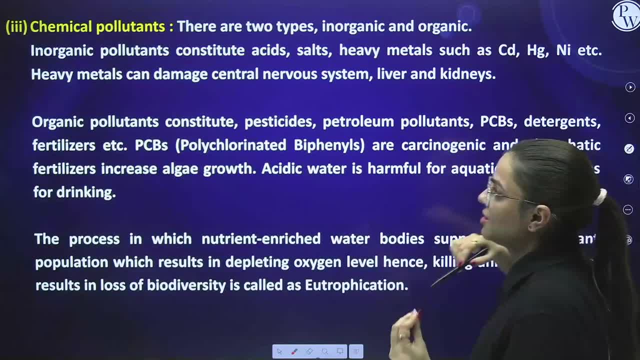 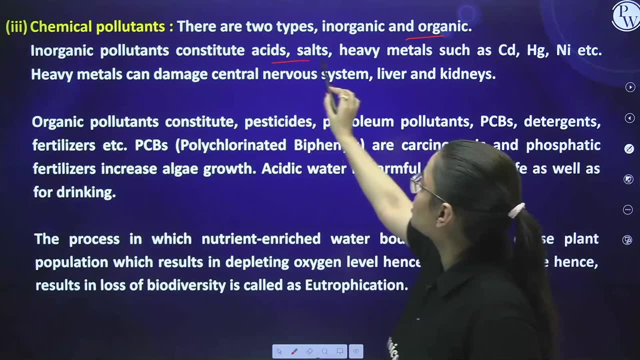 facilities, bacteria which causes gastrointestinal disease. You know there are a lot of diseases being caused due to these pollutions which adversely affect our health. Now comes chemical pollution. okay, There are two types: inorganic and organic. one Inorganic contains acids, salts, heavy. 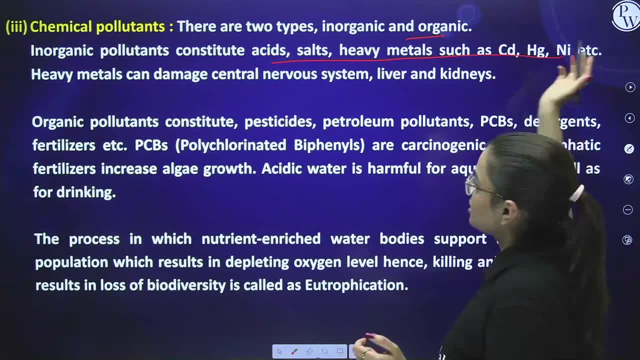 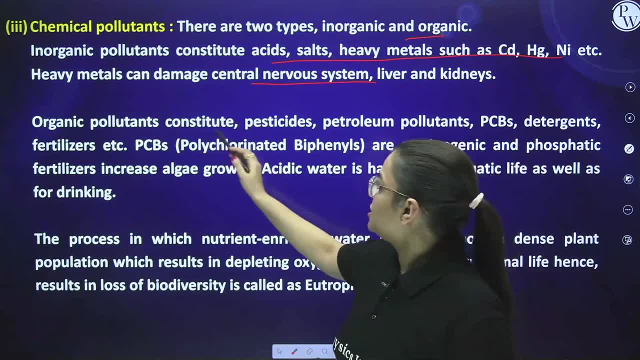 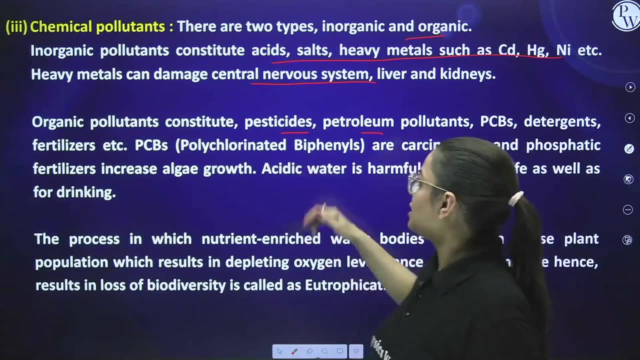 metals such as you know, cadmium, Hg, nickel and heavy metals can damage the central nervous system, the liver, the kidney right. Organic pollutants constitute pesticide, petroleum pollutants, detergents- you know all of these stuffs- and polychlorinated biphenyls are also. 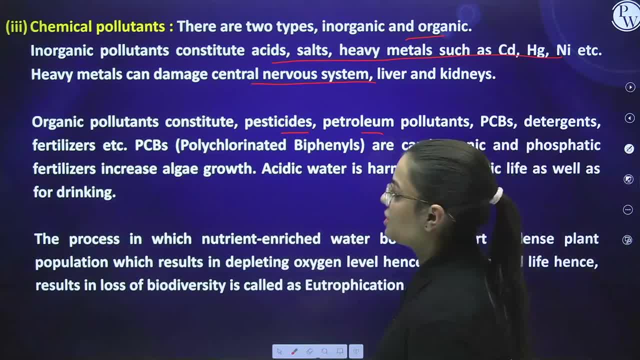 there which are carcinogenic in nature, and phosphatic fertilizers increases the algae growth. again, Inorganic means made of a kind ofодiated compound. So it's seen as a chemical material which is responsible for the pollution, which is unfit for drinking, right, Okay, the process. in which nutrient enriched water bodies support a dense plant pollution population which results in depleting oxygen level, hence killing animal life, hence results in the loss of biodiversity, is called eutrophication. You know this definition is also important. kindly put a star in your 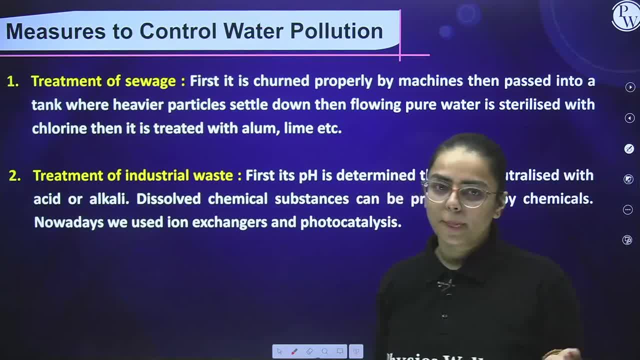 Now let us see the measures to control water pollution again. There should be a treatment of the sewage, You know, first it is churned properly by the machines, then passed into a tank where heavier particles settle down, Then, following the pure water, it is sterilized with the chlorine. 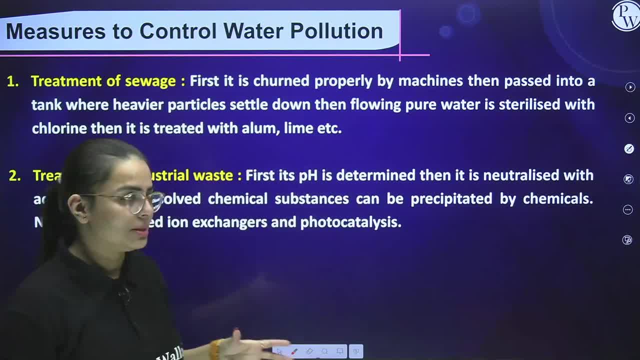 Then it is treated with alum and lime. This is the treatment Now. next, the treatment of industrial waste. First its pH is determined, Then it is neutralized with acid or alkaline. Now dissolved chemical substances can be precipitated by the chemicals. 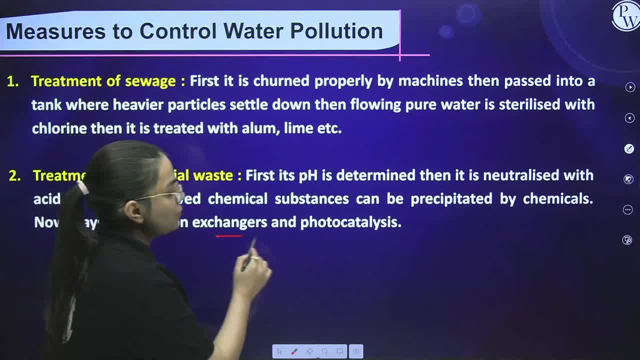 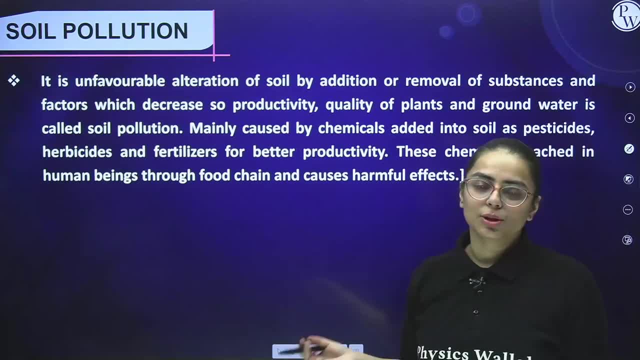 They are great. Nowadays we use ion exchangers and photocatalysis for the treatment of industrial waste. Clear, Okay, Now comes the next kind of pollution, See water. pollution was quite easy, I would say, If I talk about soil pollution. 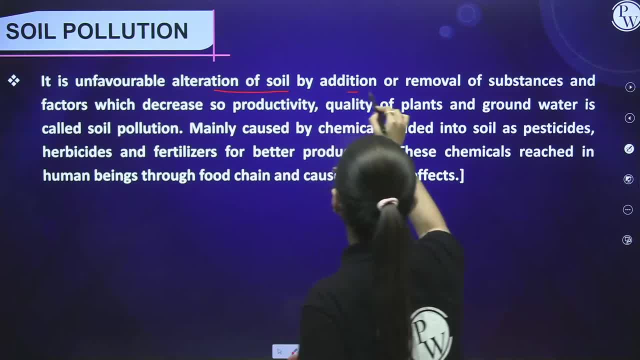 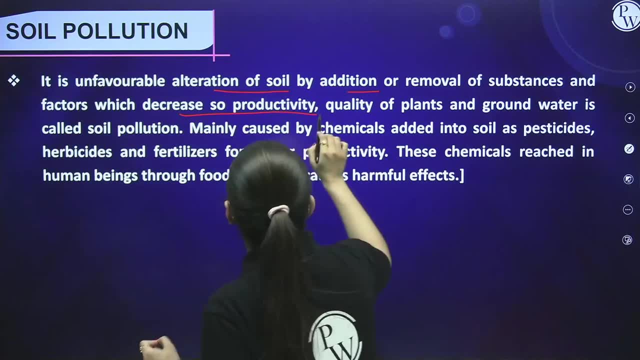 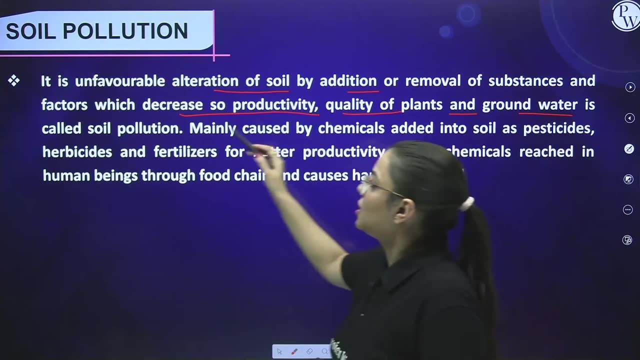 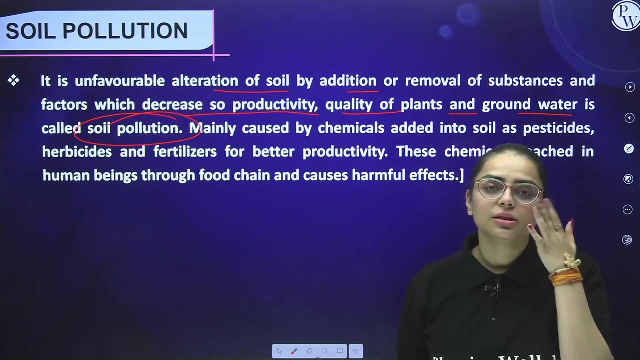 Now, unfavorable alteration of soil by addition or removal of substances you know, and factors which decreases Its productivity, its quality, you know. both of the things Of plants and groundwater is called soil pollution. Basically, the quality of the soil which gets you know which gets affected is soil pollution. 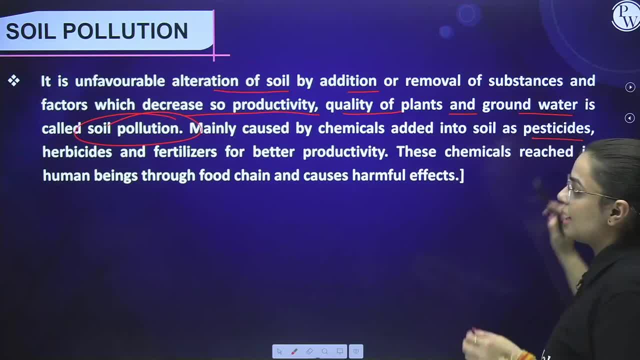 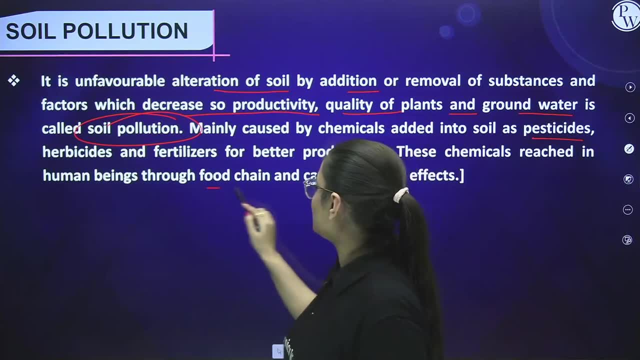 Mainly caused by chemicals added into the soil, For example pesticides, herbicides, fertilizers for better productivity. Now these chemicals reached in human beings through food chains and causes harmful effects because that food we take. It will be harmful. It will be harmful. 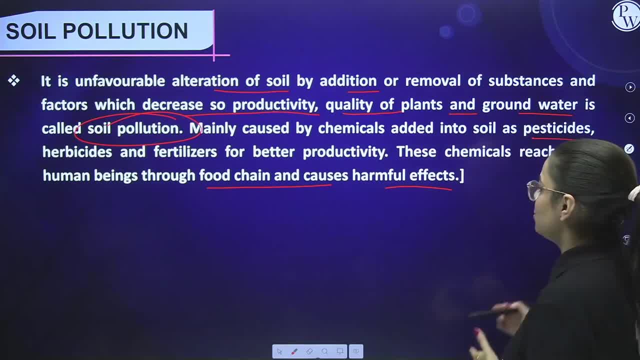 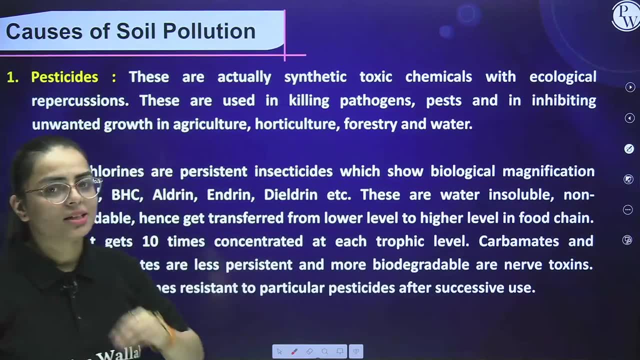 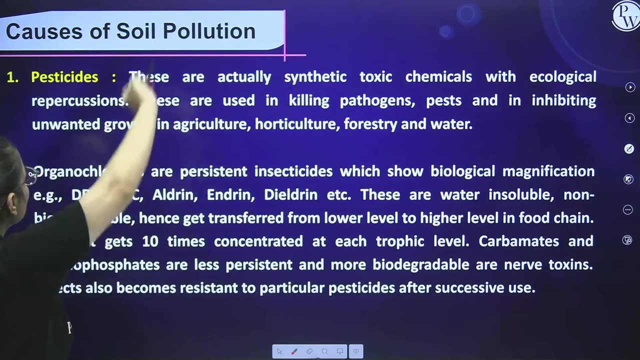 intake that food and we are having a lot of problems due to that, which causes harmful effects. now comes the causes for the soil pollution, as summed up in the previous line. first is pesticide. if i talk of pesticide, they're actually synthetic toxic chemicals with ecological- you know uh- repercussions. these are used in killing pathogens, pests and in invading unwanted 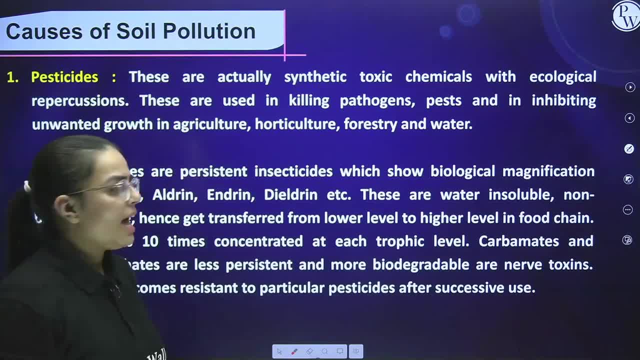 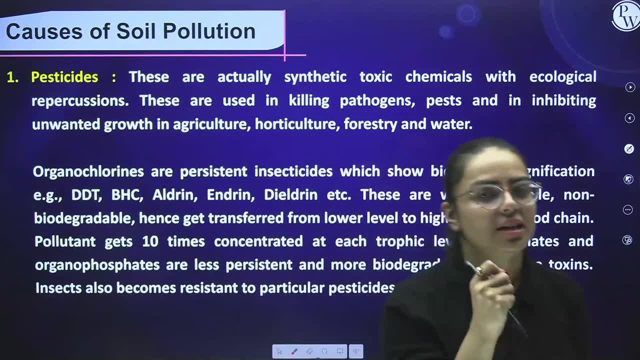 growth in agriculture, horticulture, forestry, water. i guess this is the thing that you already know. there is no need to explain over here. it is just to sit and read in the ncrp these points. right, okay now students. uh, i guess this you can read. this is not. 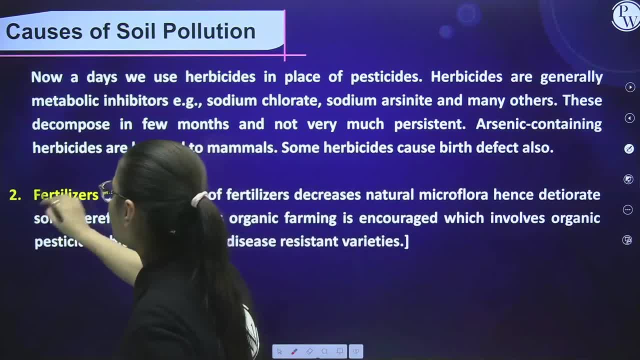 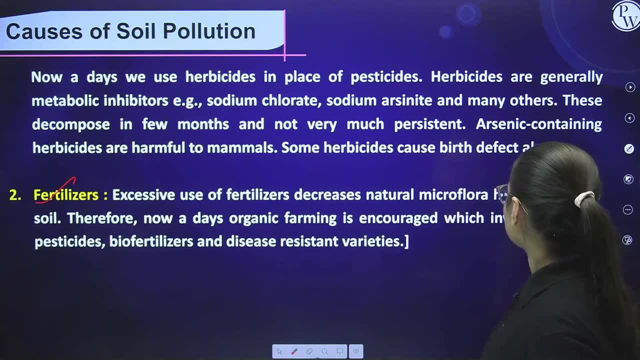 necessary for us to see. uh. the next is fertilizers. again, just like pesticides, it is the fertilizers. excessive use of fertilizer decreases the natural micro flow, micro microflora, hence deteriorate or decreases the soil, or it affects the quality of the soil. right, okay, other. 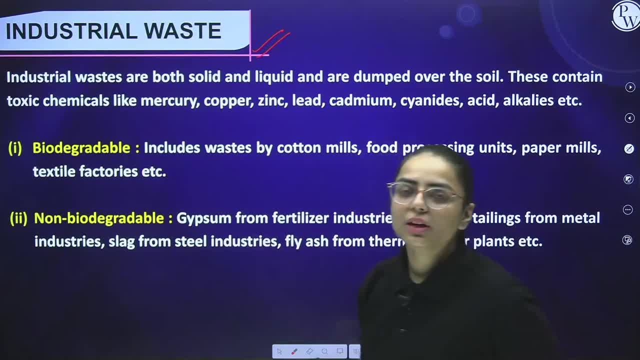 than this, students, we have industrial waste. now, if i talk about industrial waste over here, i have two kinds of ways, that is, the biodegradable and non-biodegradable. if i talk about industrial waste, they are both solid and liquid and are dumped over the soil. okay, now what happens over? 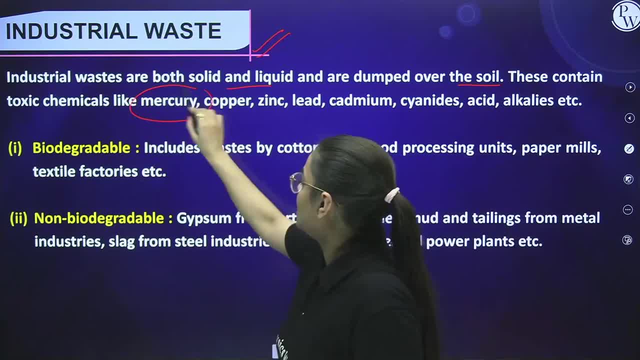 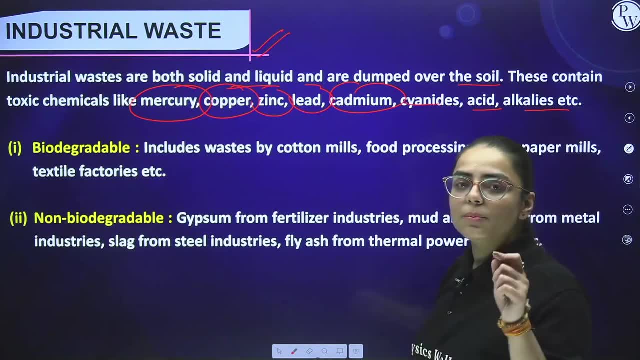 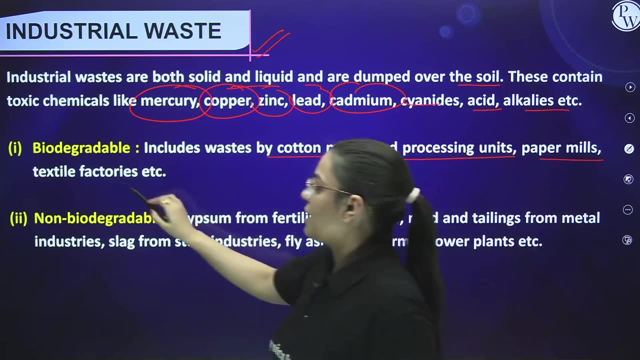 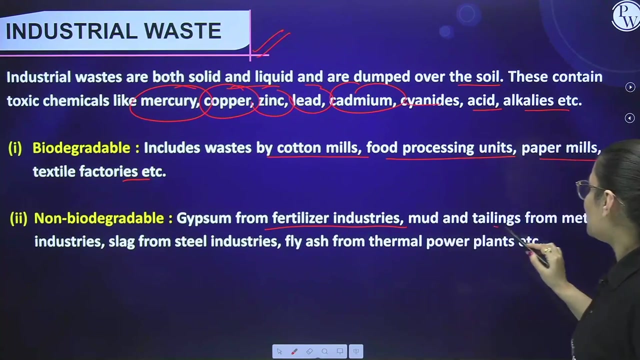 here. these contains toxic chemicals like mercury, copper, zinc, lead, cadmium, cyanides, acids, alkalis, all of these. now, what are biodegradable? one which includes waste by cotton mills, food processing units, paper mills, textile factories. all right, this is biodegradable. if i talk about non-biodegradable, it is gypsum from fertilizer industries, mud and tailings from the 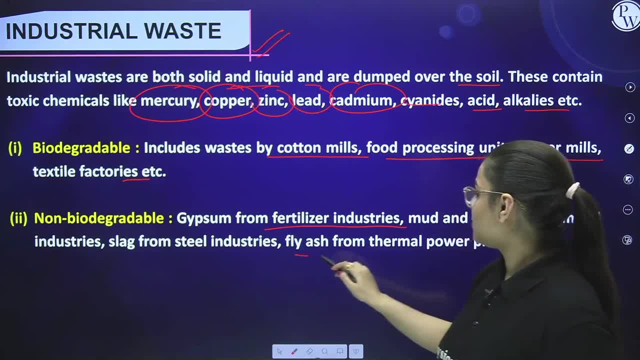 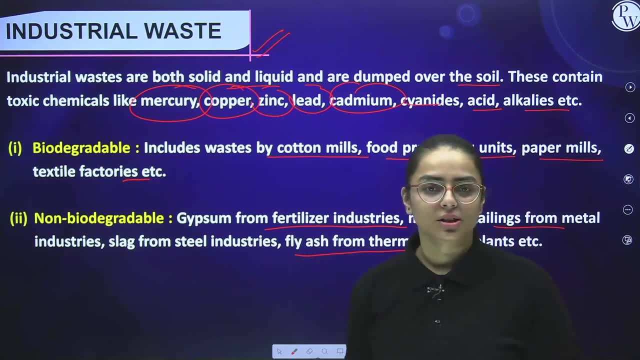 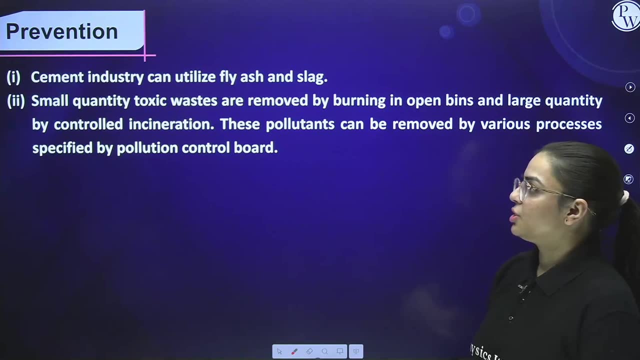 metal industries, slag from the steel industries, fly ash from the thermal power plants, all of these stuffs right. so this is basically the biodegradable one and the non-biodegradable. is it clear to you? great now, students, if we talk about the prevention over here, let us see the prevention the very first. 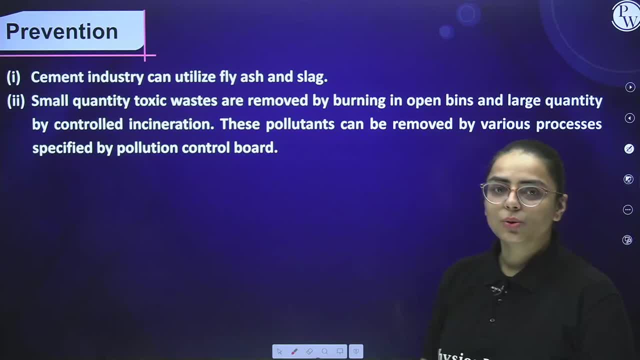 prevention is: cement industry can utilize fly ash and slag. okay. the next is basically: small quantity toxic waste are removed by burning in open bins and large quantity by controlled, you know, in serenation. these pollutants can be removed by various processes specified by pollution control board. now this is again the prevention method that you need to remember. you can write on. 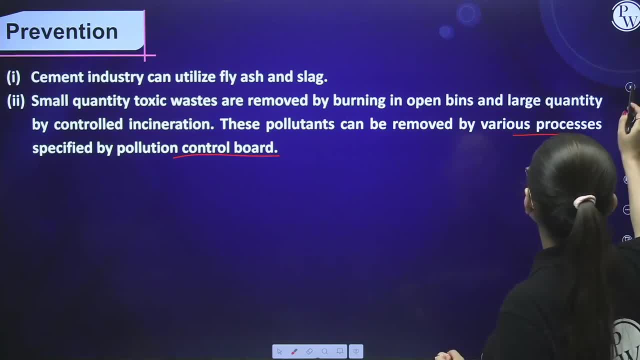 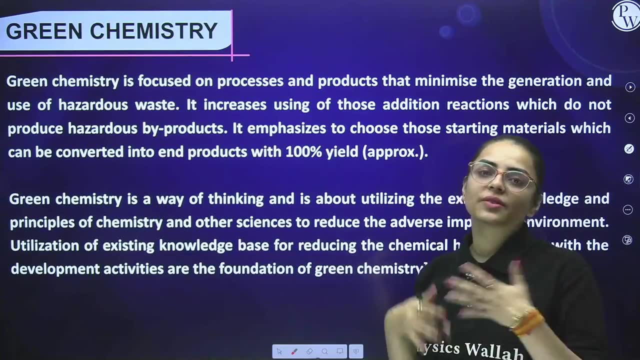 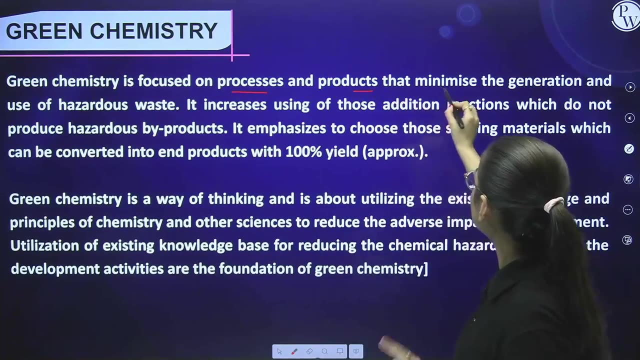 your own also. let us see, students, our next segment over here. now we have green chemistry. now, green is basically the chemistry that we are going to use to save our environment. how can we do to see? green chemistry is focused on processes and products that minimize the generation and the use. 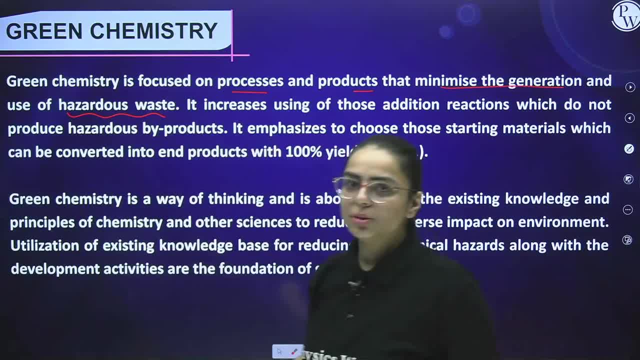 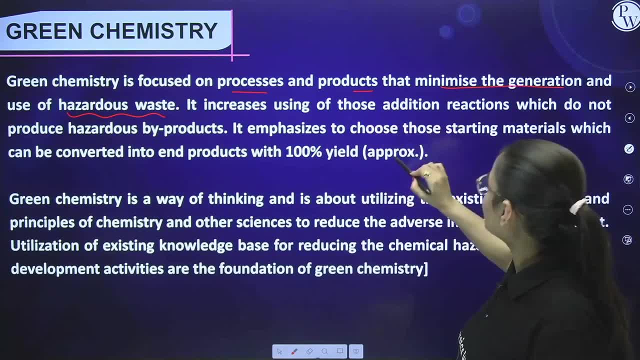 of hazardous waste. you know the production. i would say it minimize the production and the use of the hazardous waste. it increases using of those addition reactions which do not produce these hazardous byproducts or the harmful byproducts. it reduces its effect. right, it emphasizes to choose those starting materials which can be converted into end product. 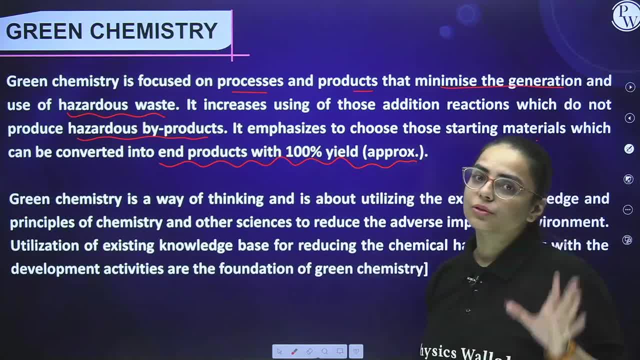 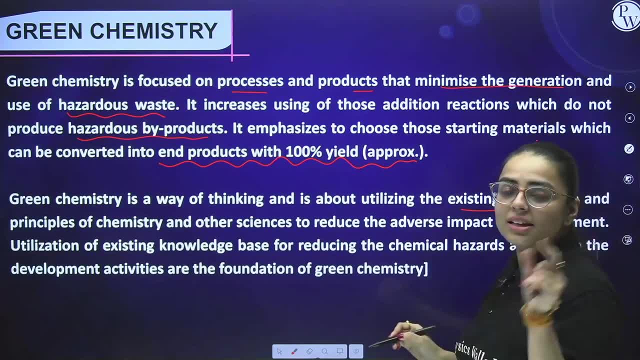 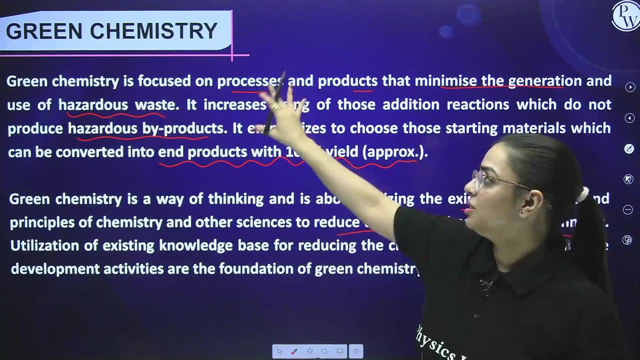 with 100 yield and which are not harmful for the environment. green chemistry is a way of thinking and is about utilizing the existing knowledge and the principles of chemistry and other science to reduce the adverse impact on environment. so this is the thing that we can use to save. 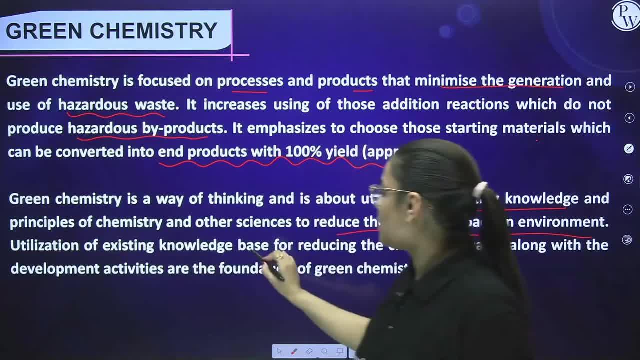 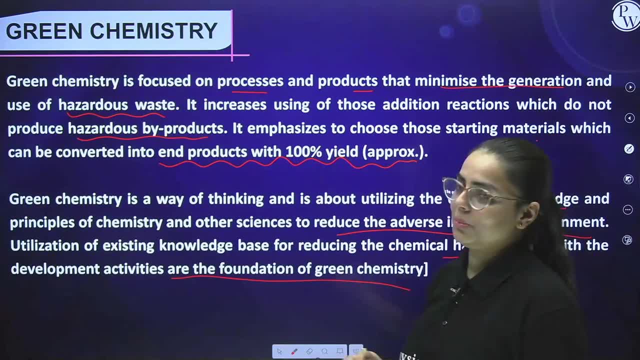 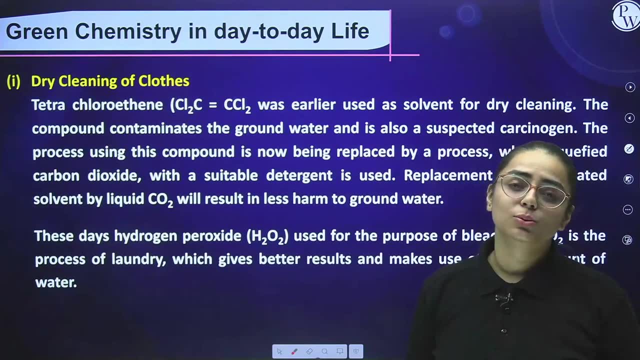 our environment. right utilization of existing knowledge space is to increase the potential of water use. we can also balance that in a simple way by tourists believes that green chemistry is on some of the ground in ancestral waters. but you know, this is the way of life. it is willозя. according to science, our retina gets polluted if that happens. 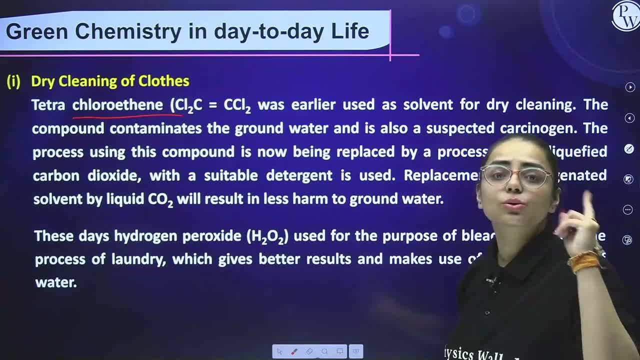 the autantism will happen right. so here it's coming. i've been talking about this, that pulling the dichromycin from having different minion cells and kicking them all out. so if you want to understand the way that this rejuvenation is, like the way that environment works, 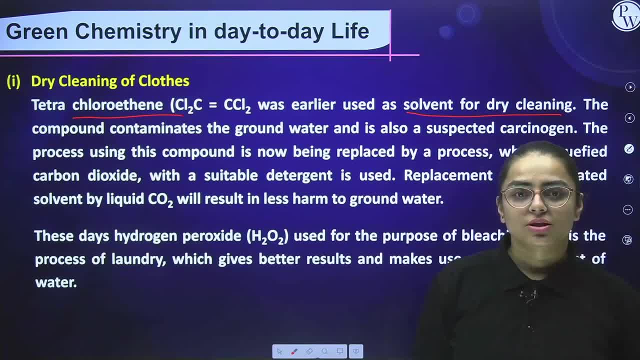 it is to neutralize虹. it is abai c it Workers связ. if you donets Battle forming, you know it is also part of the process called multi application, which we pretty like to know. a little while ago we talked about this is Sara. i said level which recreation. who in the 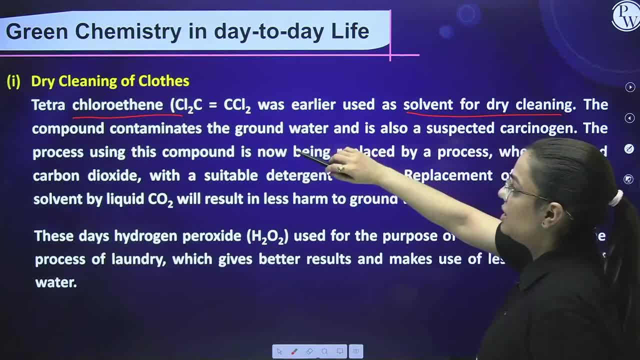 smallnak. which language is how i learn and bor hat meaning or charity? which language is aging? you is quite easy, right see. tetrachloroethene was earlier used as a solvent for dry cleaning. the compound contaminates the ground water and is also a suspected carcinogen. now, if 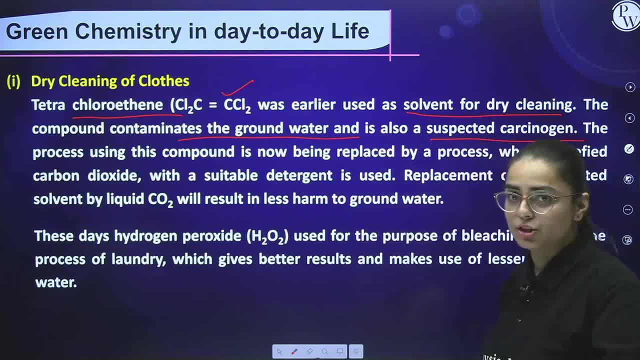 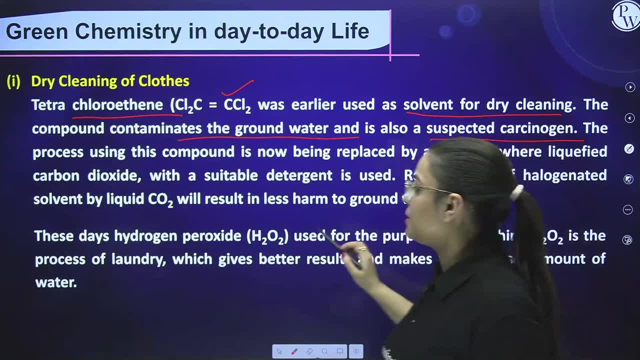 this is a carcinogen, you know. it is replaced by h2o. now what happened? the process using this compound is now being replaced by a process where liquefied carbon dioxide with a suitable detergent is used. replacement of halogenated solvent by liquid co2 will result in less. 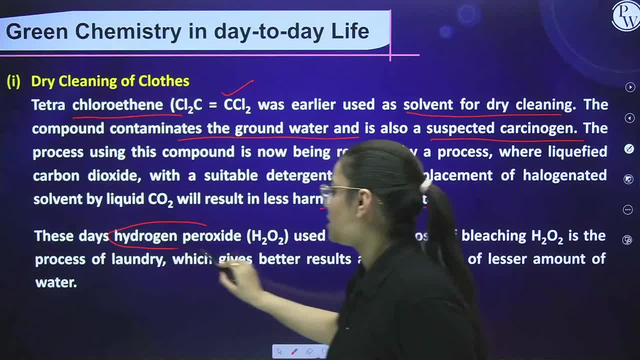 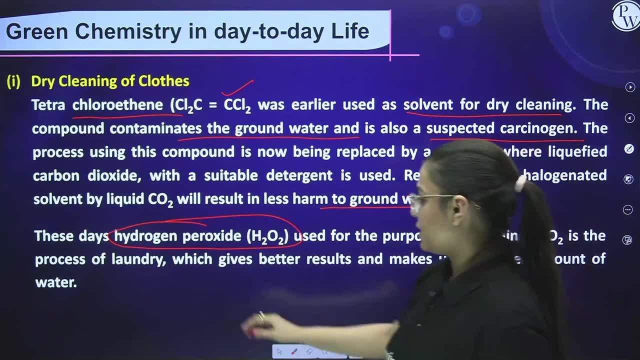 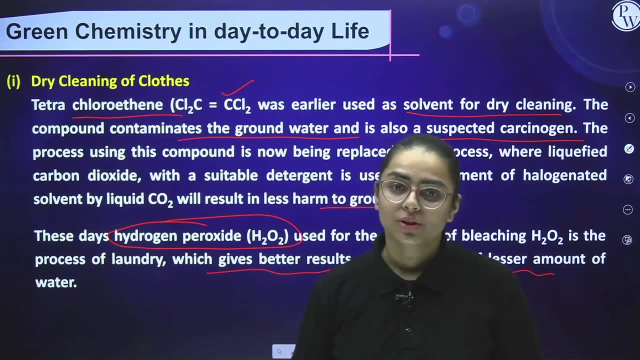 harm to the ground water. these days, hydrogen peroxide, as i told you, h2o2, used for the purpose of bleaching. h2o2 is the process of laundry, which gives better results and makes the use of lesser amount of water, so it has best, better results also, right, so this can be used now. 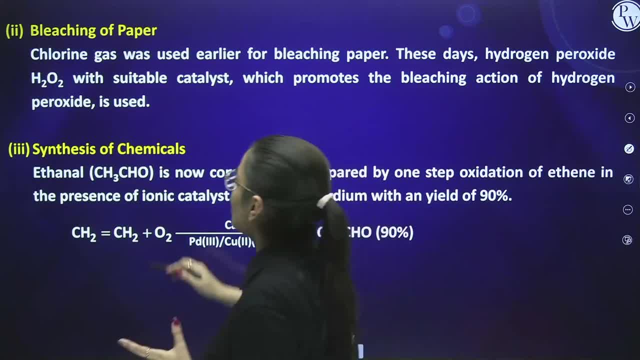 the next thing in day-to-day life is about the bleaching of paper. see over here now. chlorine gas was used for like for bleaching paper. these days, hydrogen peroxide is used for bleaching of paper, so this can be used now. the next thing in day-to-day life is about bleaching. 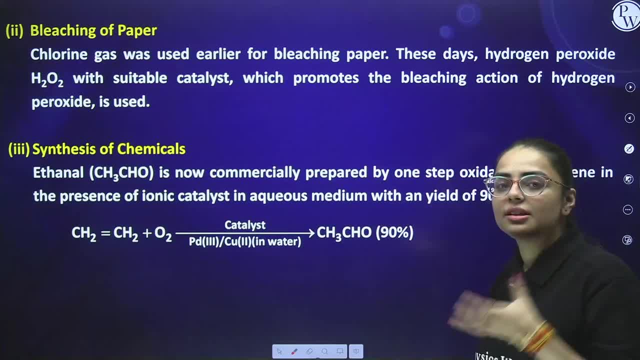 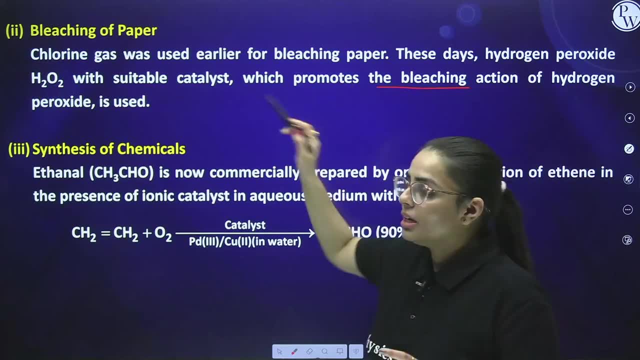 of paper. this is a process of reducing the chance of a performant reaction of hydrogen peroxide, again with suitable catalyst. now, catalyst can either increase the reaction or decrease. the reaction depends upon which catalyst we are using right, which promotes the bleaching action. here we are using a positive catalyst which basically increases the reaction. 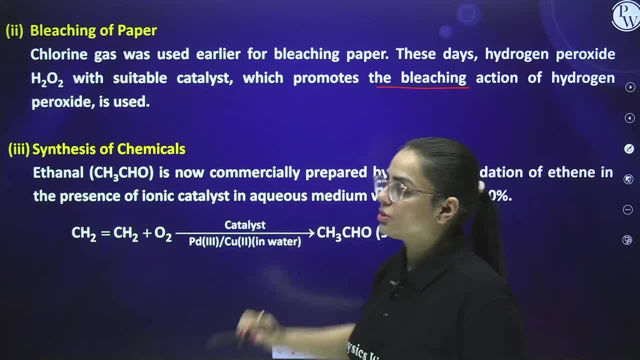 ok, now what happens of the hydrogen peroxide that is being used? now comes synthesis of chemicals. ethanol is now commercially preferred by one step: oxidation of ethnein in the presence of ionic catalyst in aqueous medium with a yield of 19%. so this is the weakening of the 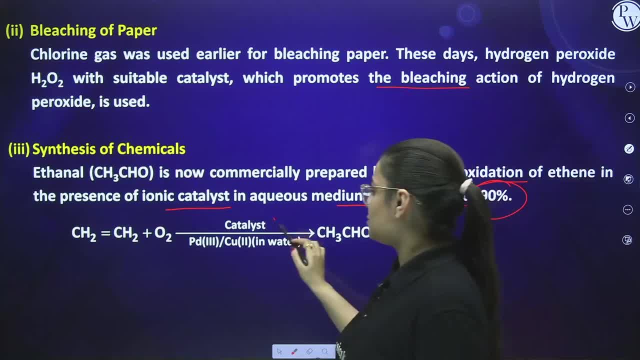 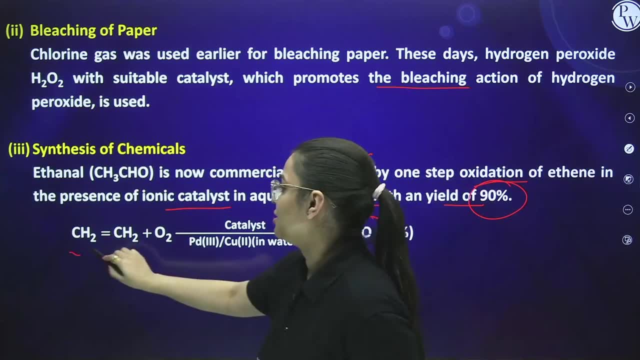 chemical 마음in social巨 part of the process which is called a neutralization of the grade percent. you know, you can see this in the presence of catalyst. now ethanol, basically, is now commercially prepared. we prepare ethanol from this ethane. is it clear, students? so by this way, green. 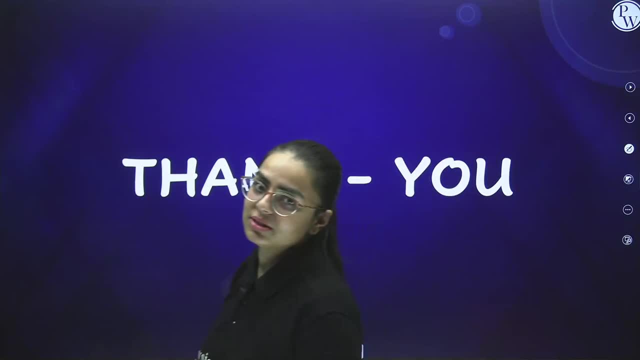 chemistry is used in our day-to-day life, students, it is used in our day-to-day life. so, yes, students, this ends our chapter. we have seen air pollution, water pollution, industrial pollution, foil pollution and green chemistry, right, so these all are the things that we've already studied. but, yes, now we 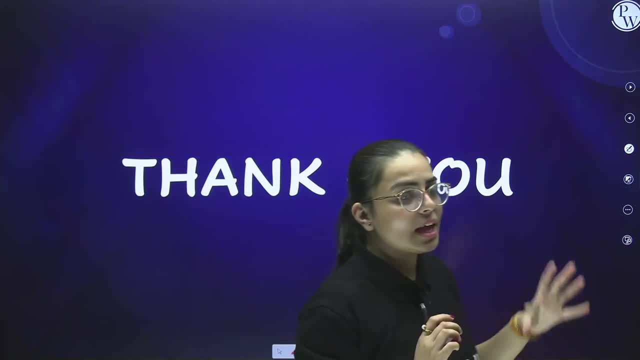 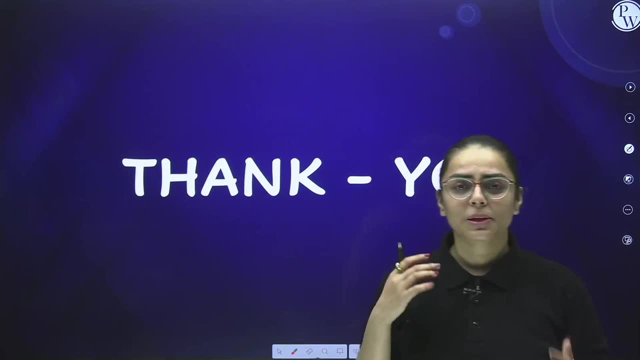 have done in a symmetrical manner. we have read all this. i want you all to practice your dpp, because all of the questions are theoretical. so you'll practice in the dpp. you'll get to know how the questions are being asked, because many of the questions are some of the previous years, some of 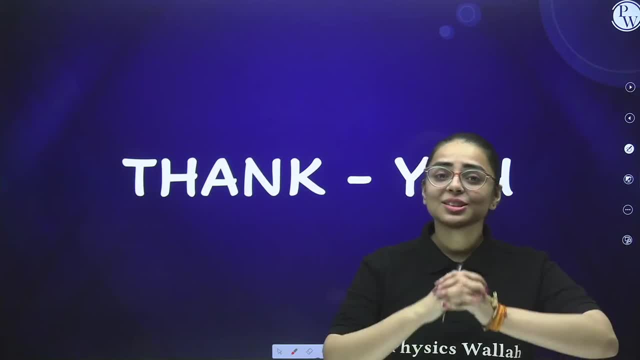 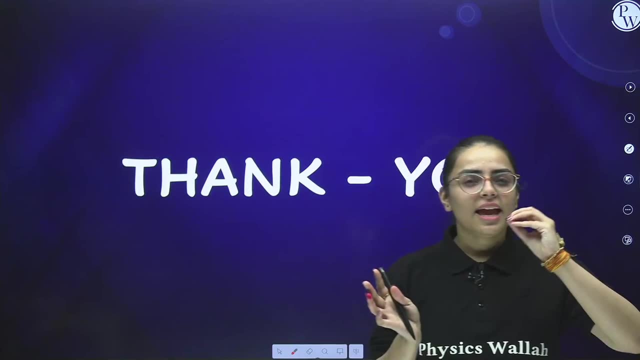 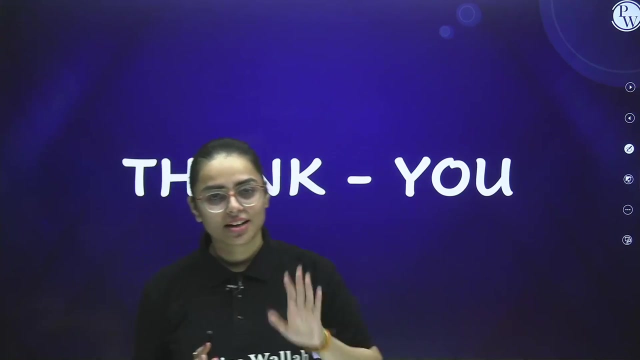 are from the good books right now. students, this also ends our organic chemistry of class 11. but as you all know that every story has an end, but in life every ending is just a new beginning. so i would just say never, never give up in your life. you know, just practice. we have covered all the lectures of the class 11 of. 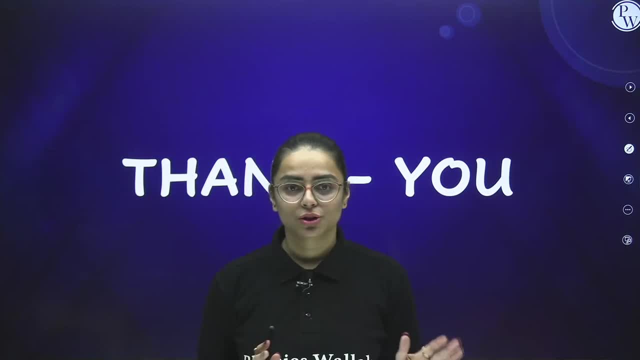 organic, of physical chemistry, of organic chemistry also. so i want you all to practice more and more questions and whenever you are stuck in a particular question, kindly go back to that video or go back to your notes, re-revise it and brutalize it concept in your questions. you will be able to achieve it until and unless you do it right. so